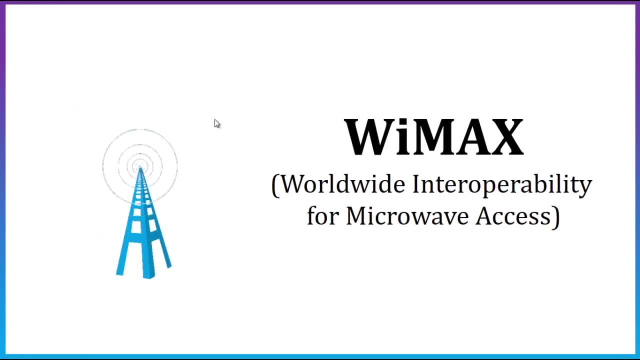 AAA standard of 802.16 standard, which provides you a high-speed data over a wide area. the later, WiMAX, stands for worldwide interoperability, for microwave access, and it is a technology for your point to multipoint wireless networking. okay, so before that, I need to clear out some of 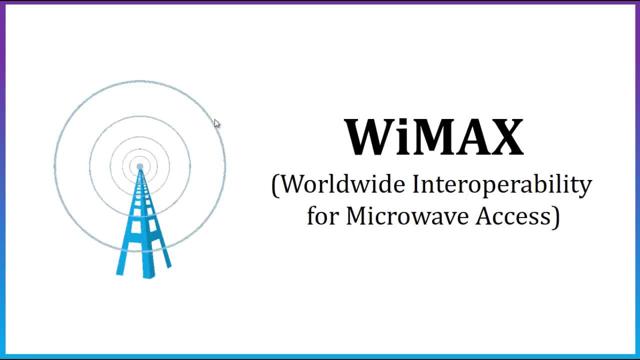 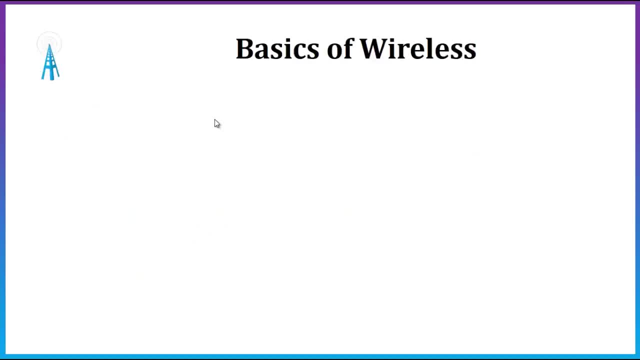 the basics of your wireless. so, before directly getting into an WiMAX, I will just briefly sum up what is a wireless so just to start with. so what are the basics of wireless? so wireless means transmitting your signals using radio wave as a medium instead of wires. so wireless technology are used for a task simple as a switching, or switching on and off your 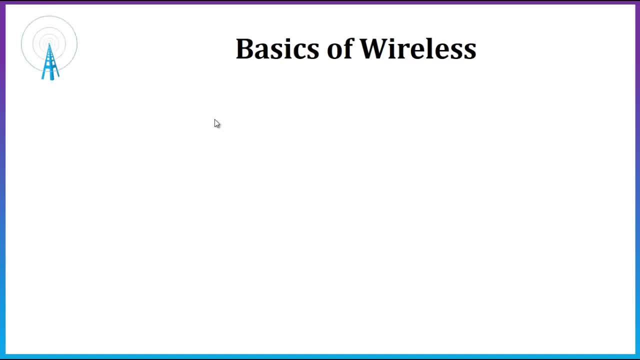 television or as complex as like supplying a Salesforce with information form and automate, automated enterprise application, while in a field now- cordless keyboard and mice, your bounce, your PDA pager and your digital or cellular phones- it has become actually a part of our daily life. so wireless is being very much. 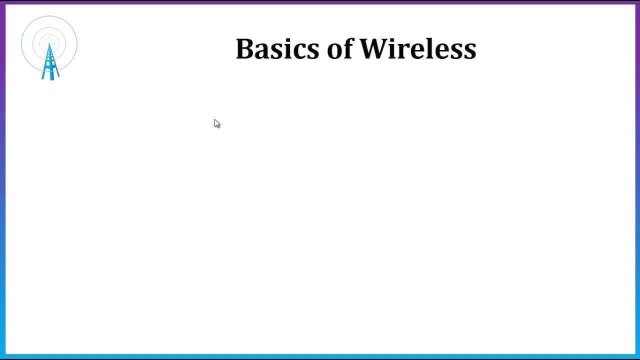 known to you. so some of the inherent characteristic of a wireless communication system which may make it more attractive are like mobility, then reachability, then simplicity, maintainability, then new services are there, then roaming services are there, so in general, uh, wherever it comes out to be like a basic of wireless, so basic of wireless is in general. so whenever it was a case, like you, 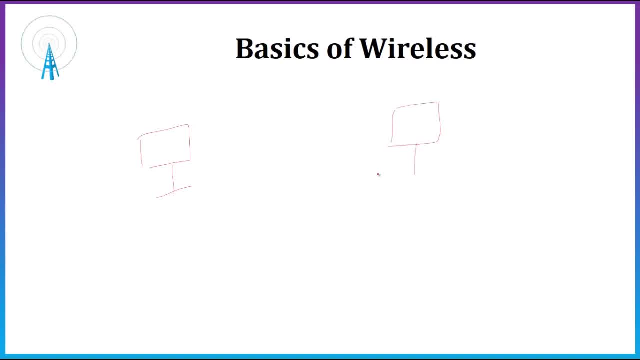 have one PC and you have another PC here. so we used to have some kind of topologies to connect an internet over this as many number of pieces which you want to create a network. so it was a case like I cannot move this particular PC to another place, or even like, uh, if I need to create a tapping, so yes, I could tap it. 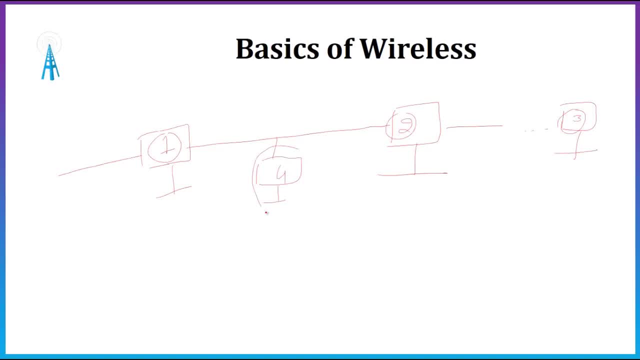 here and I could put a another node here, but again, this is called as actually a security bridge. so this security breach will arise in these kind of networks. but if, in case of wireless, if I have simply like my PC is there, my mobile is there, or even like my tab is there, so 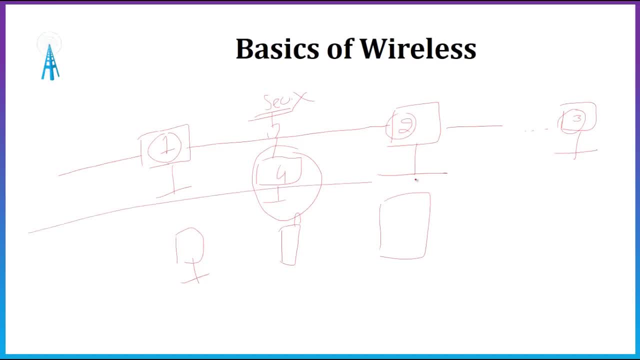 everything is there in a network or in a mode of wireless. so in that case, if they are associated with some kind of access point, that in that case everyone is connected with that access point and no one in uh, no new node will be able to connect in that particular segment or that particular. 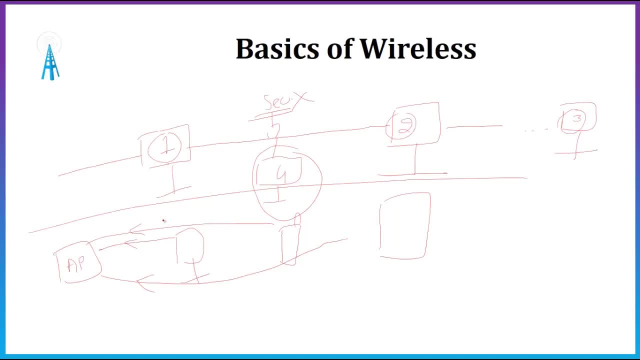 access point, then authentication is not done. it is simply like: uh, in your institution you don't have a access to some of the some part of a network, and if you want access to your Wi-Fi network, that in that. in that case it is always mandatory that you need to register. uh your device with a system like your. 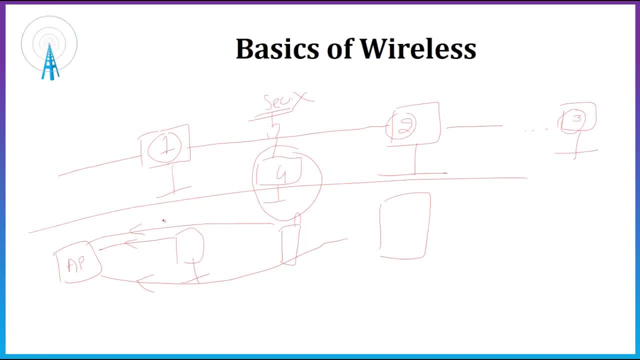 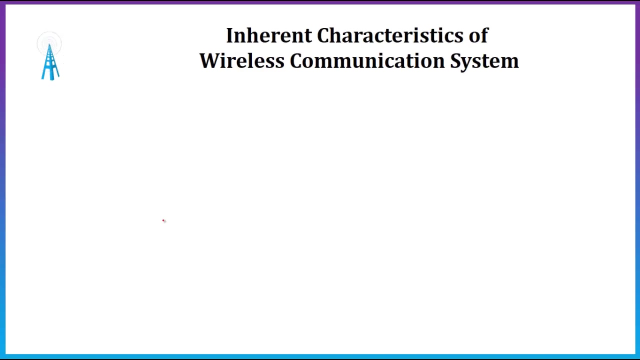 Mac address needs to be registered, a hardware Mac address, so so that a system will understand the- yes, this is a authenticated person to use the network through the wireless connection. so that's why wireless is always better than your wired- uh, wired- operation. so this is a basic idea. so what are the different inherent, inherent? 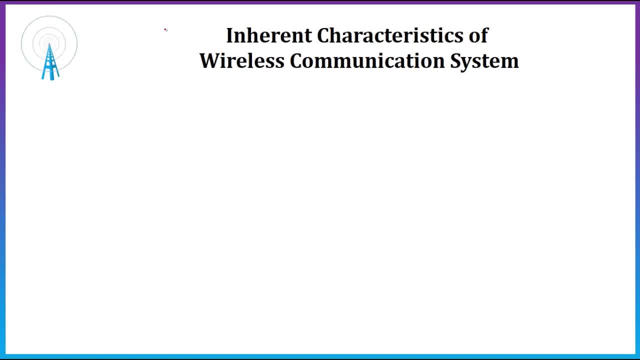 characteristic of your wireless communication system. so we'll just list it down and then I'll explain one by one. so first one is your mobility. so obviously that is a big characteristic and you always understand is mobility. the second thing is reachability. then third one is your simplicity. 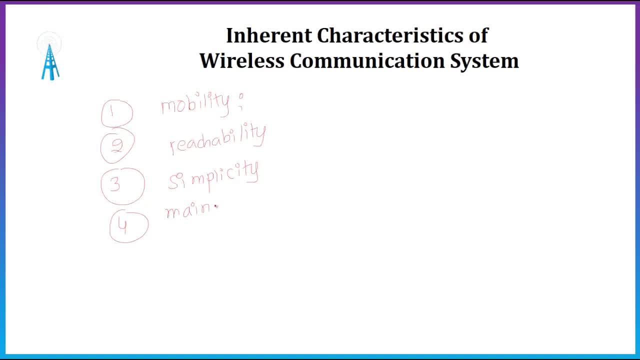 and fourth one is your maintainability, then the fifth one is your roaming service that you could actually roam around, then the sixth one is your new services. so these are the few of the inherent characteristic of your wireless communication systems. so now, by a, each individual word, we better understand what are their meanings. 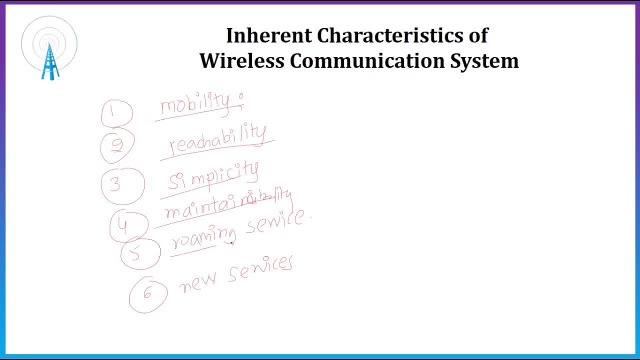 like mobility, reachability, Simplicity, manteinability, roaming service and new service. so we just need to see what are those words in terms of Wireless communication. so mobility is like a wireless communication system that allows user to access information beyond their desk and conduct their 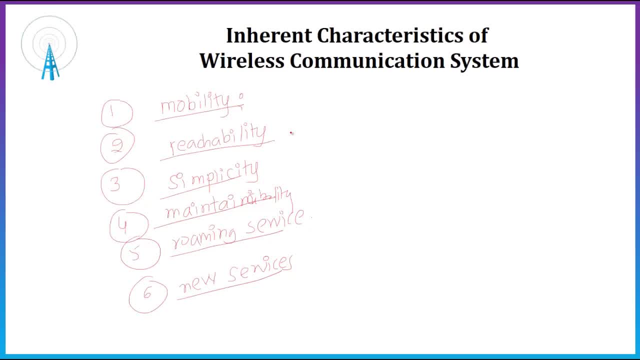 business from anywhere without having any wire connectivity. okay, so that is a technical terminology, terminology of your mobility. So again, what is reachability? So reachability is actually like a wireless communication system, uh, that enables people to stay connected and to be reachable, regardless of their location and their operate, uh, and what they are operating. 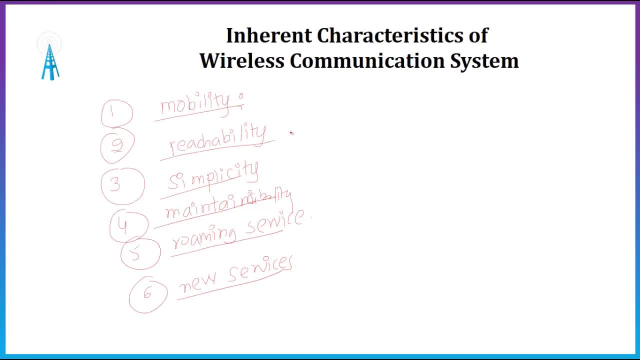 and where they are operating from. Okay, Uh, so simplicity. simplicity is like uh. it's a system which are easy and fast to deploy in comparison to that of the cable network. The initial setup cost will be bit high, but obviously the other advantages will overcome. 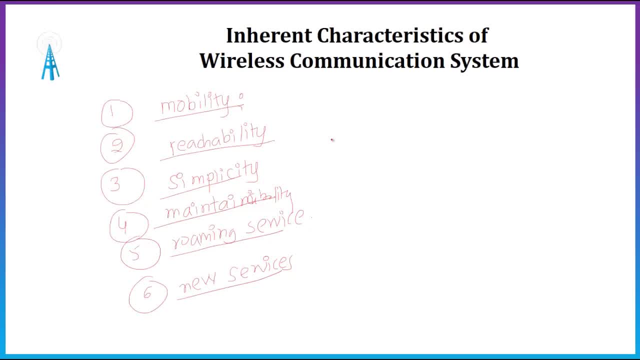 the other high cost. Okay. So simply, like in simplicity, we could say that: uh, I have some kind of a network, Uh, uh, for example, I'll consider a wired network in the wired network, Once the connection is established between our systems. So if you want to incur, 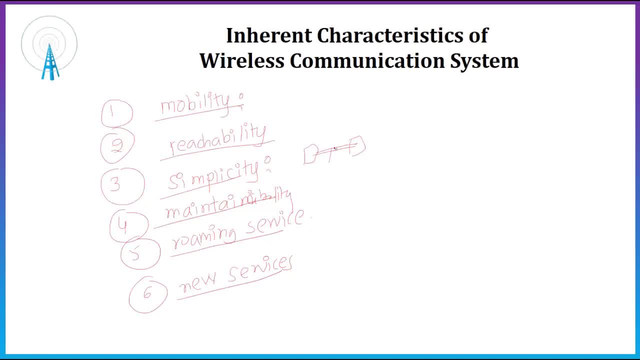 a new system. So for that you need to create a patch somewhere, you need to add a new device, you need to get it registered and you need to see whether it is connecting or not. So but whereas in wireless, if you have already established a network and you need to incur some new device, 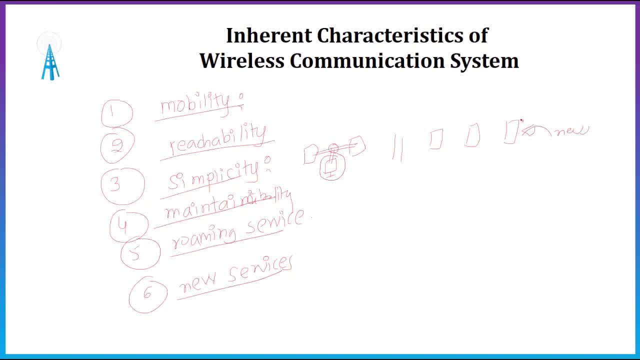 in that case it's common sense that you just need to put simply like on a server, you need to deploy some address and that's it: your new device will be added into a network and obviously you will get a service. but whereas this was actually a trickier process that you need to have actually physical 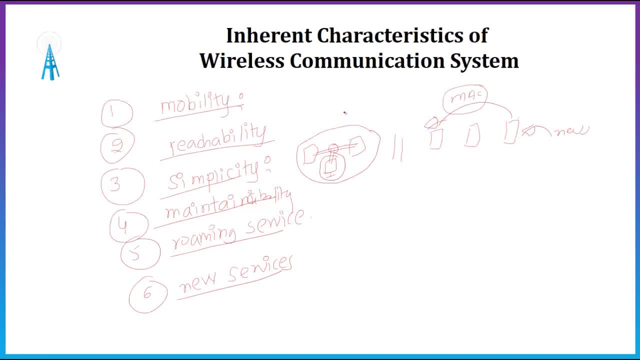 media will be required to connect to that device, and again it will be struck, so this thing will be lost. so simplicity means you can easily maintain those things, or we could say advantages in case of like easy to deploy. so that's it. that's why simplicity. then next one is your maintainability. 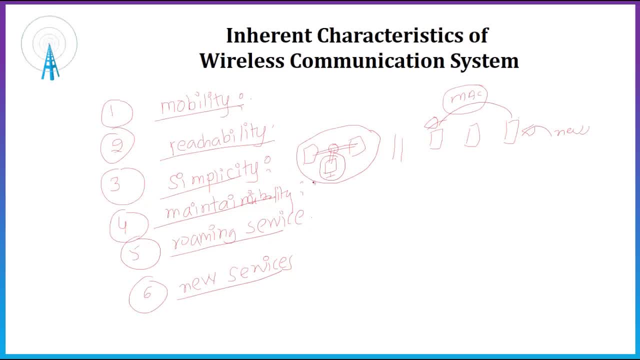 so what is maintainability? so obviously in a wireless system you don't need to have or to spend much time or much cost to maintain that particular network setup. it's actually a one day job, or like system root, systematic system rebooting: they're maintaining their different. 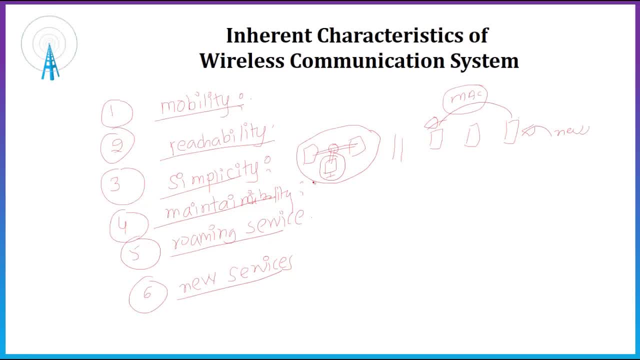 access points and all those things, that those are actually a one day or two day jobs, but whereas maintaining your wired network is actually a difficult thing, then next is your roaming services. so, using your wireless network system, actually you can provide a service anywhere, anytime, including your train, buses, aeroplane, anywhere. and then the new system in wireless: 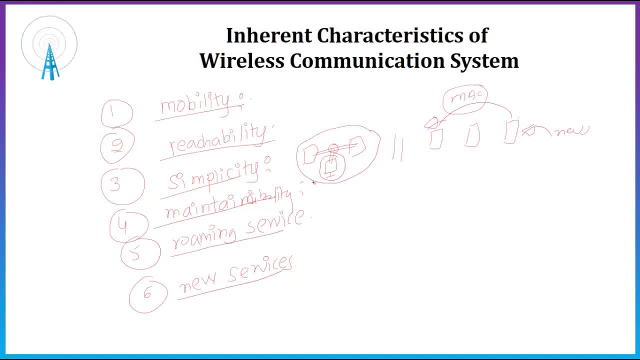 communication are like, or to provide a various smart devices, or smart devices with the smart services like SMS, MMS. these kind of new services could be deployed into your wireless network system, your wireless communication systems. okay, so we'll next see what are the different topologies of it. 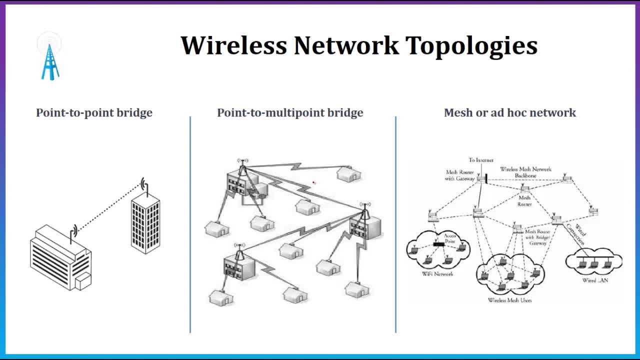 so in general in a wireless network there are topologies like point to point, point to multi point and mesh or a ad hoc network. so these are actually we could say it's a permanent network, this is also a permanent network, this one is a permanent network and again, this is we already know. ad hoc means temporary network. okay, so in 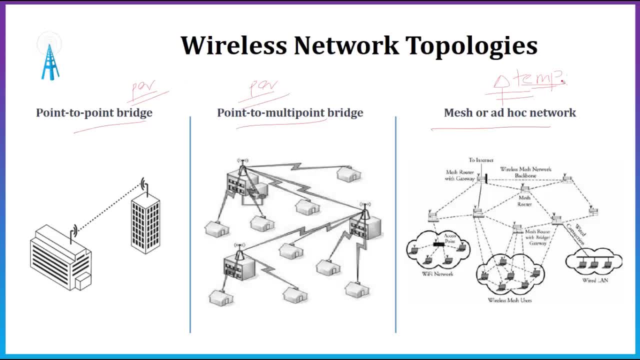 general, in a point to point bridge, or in a point to point bridge topology. as you know, a bridge is used to connect two networks. a point to point bridge interconnects your two buildings having a different network. so, for example, a wireless land bridge can interface with a Ethernet network directly to a particular access point. okay, so what is in point? 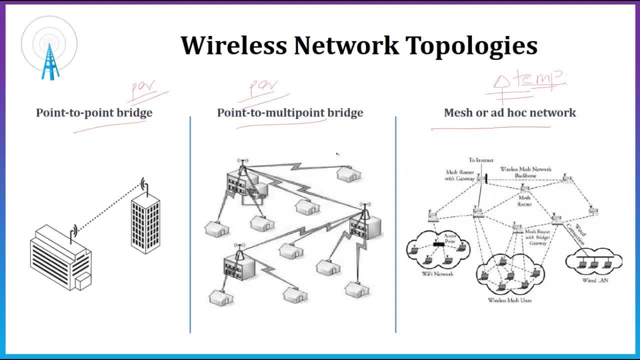 to multi point bridge, so point to multi point. this kind of topologies is used to connect three or more lands that may be located on a different floors, floors in a building or across buildings, different buildings, so this kind of hierarchy would be there, that these are three different. 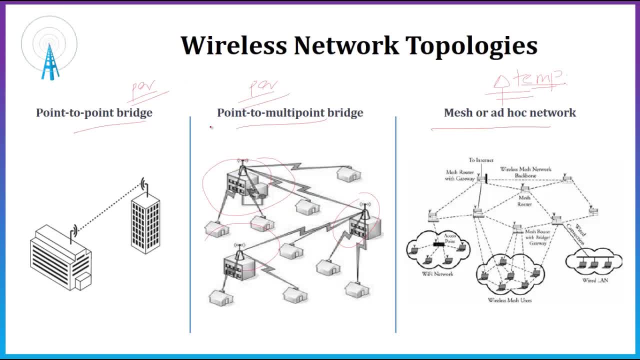 buildings and there are various networks are there, so that will be called as your point to point bridge, to point bridge, so the mesh or ad hoc. so obviously it's a temporary network. so this network is an independent- uh is an independent local area network that is not connected to a wired infrastructure. 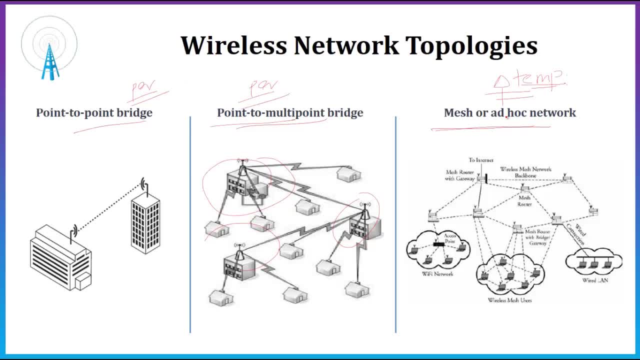 and in which all stations are connected directly to one another, like we have seen in this particular image. so there are different networks. they are associated through the different mesh router and all those things. so this is a topology which is called as mesh or ad-hocnato. okay, so next one is: 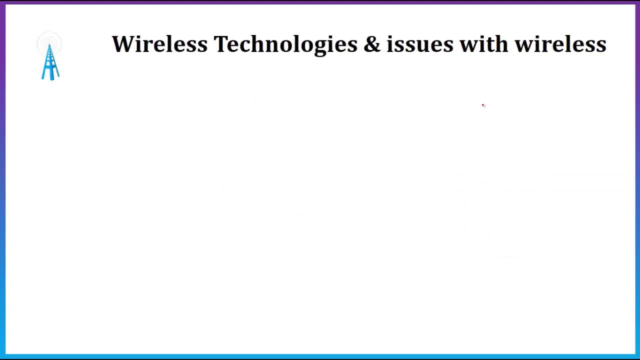 your wireless technologies and different issues that we face in wireless. so wireless technologies in general. they are classified into various different segments, like they will just note it down one by one and we'll discuss it. so the first one is your W pan, then the second one is: 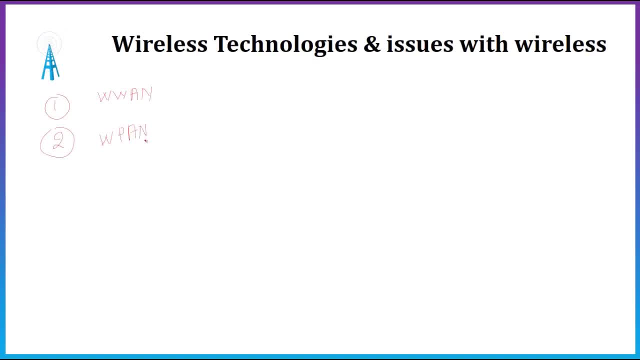 your W pan, then the third one is W lan. then we could say there is another W man, then again there is one major which is to be considered as a WB a okay, so these are actually in general considered wireless technologies. so what are these W and W pan, W lan, W man, W BA. so 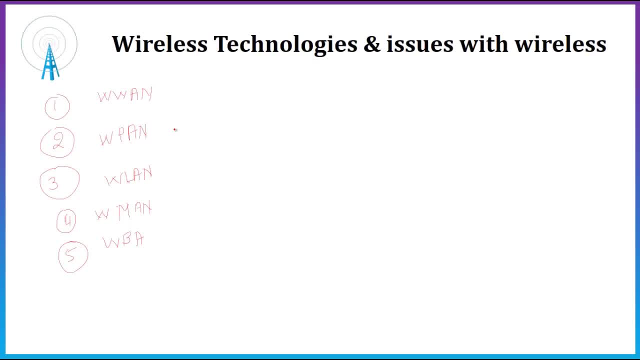 I like some one by one. so, W van, is your wireless wide area network? okay, so wireless wide area network. so these kinds of network enable you to access internet via wireless wide area network access card and a PDA or a laptop. so these network provide a very fast data speed, comparing with the data rates of your 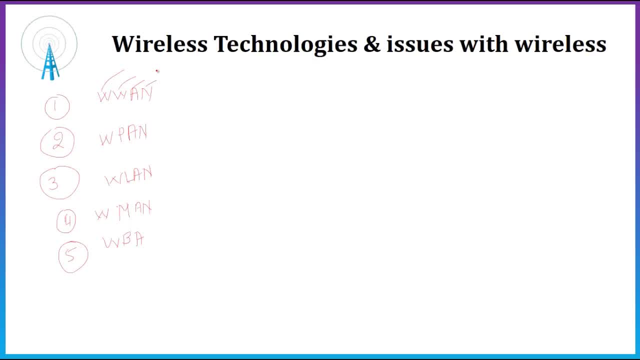 mobile telecommunication technology, and their range is also extensive. the cellular and your mobile networks are based on CDMA, and GSM are good example of your WAN, wireless wide area network. okay, so what is then WPAN? so these kind of networks are very similar to your WAN, except the range for WPAN is actually very small, so obviously this is called as. 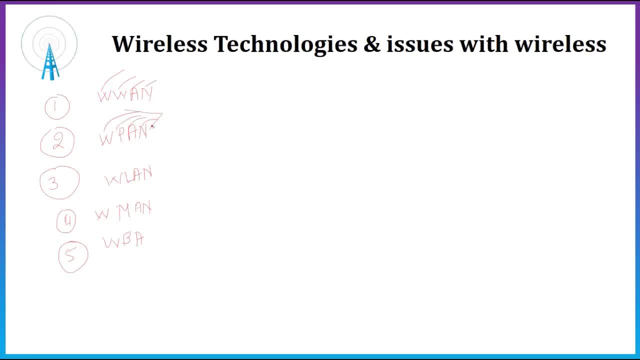 wireless personal area network. so obviously the range of network is very less and in this case range of network is very high. so example is like your. what we could say is your 3G, 4G or in general, cellular system for attacks. so this cell system, okay, so these cellular system will be considered in WAN. 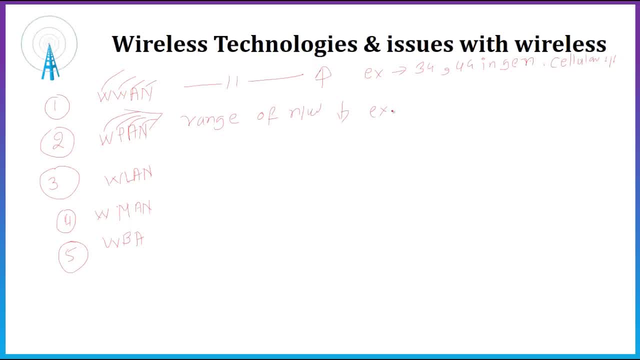 and WPAN are like we could say as a Bluetooth, ZigBee, these kind of whatever. they create a terminology. So in general, you have seen it in a Bluetooth and ZigBee. so they create a WPAN, Wlan. So wireless, So wireless. 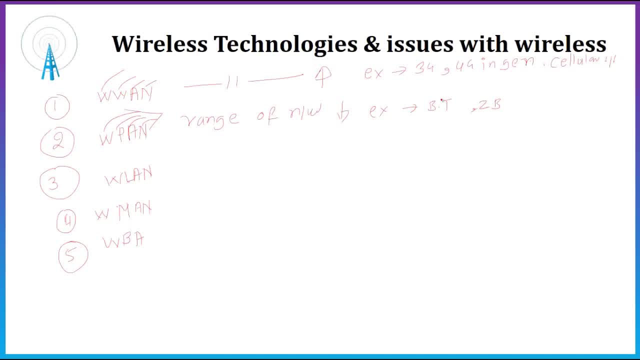 wireless local area network. okay, so in wireless local area network. so these kinds of network enables you to access the internet in localized hotspots, or we could say via a local area network access card or a laptop. so it is a type of local area network that uses a high frequency radio. 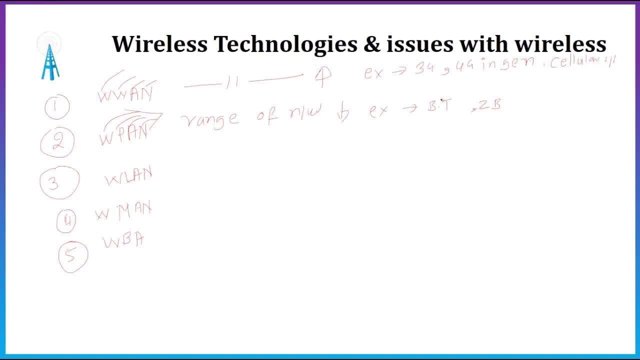 waves rather than your wire or wires to communicate between your two different nodes. so these network provides a very fast data as compared to that of your PDA and again, the data rates of your mobile telecommunication technology and their range is very limited. so in comparison we could say, as compared to your mobile telecommunication technology, their range is limited with Wi-Fi. 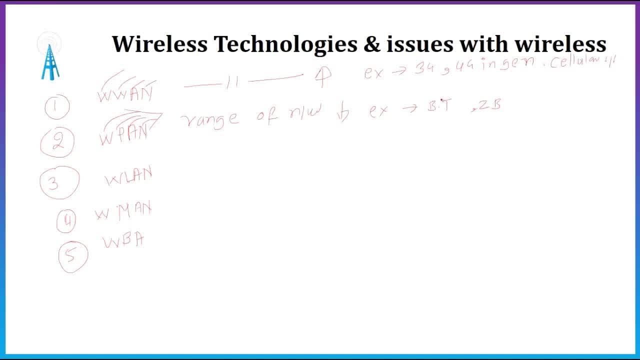 but actually the bandwidth or speed is more so. the Wi-Fi is actually a most wide spread and most popular example of your wireless land technology. so next, what is W man then? so W man is actually your wireless metropolitan area network. so this network enables you to access internet and multimedia stripping in services. 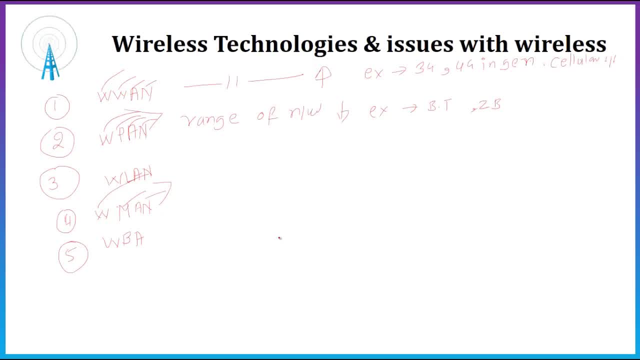 like wireless region area network, so sometimes W man is considered as your W ran. okay, so, so your W ran is nothing but your wireless region area network. okay, so these network provide a very fast data speed compared to the data rates of your mobile communication technology and as well as your other technology. so W? 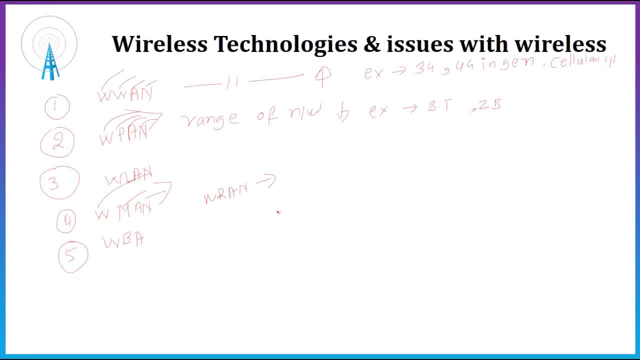 man is actually a most popular thing nowadays. so now, yes, second segment, it is. so what are the issues with your wireless? oh, I think I just forgot one more thing. yes, WBA, so we'll just cover it. WPA. so what is WBA? so WBA is actually your wireless broadband network, or we could say: 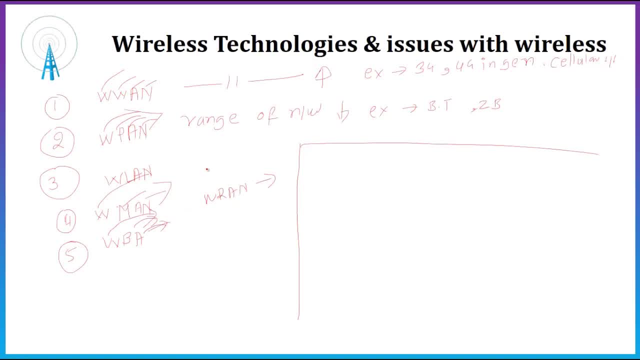 wireless broadband access. okay, so wireless broadband access. so I'll explain this thing. so broadband wireless is a technology, signal technology, so it has a sort of very low-range communication system that actually promises a higher speed connection over the air. so it uses radio waves to transmit and receive data directly to and from a potential user. 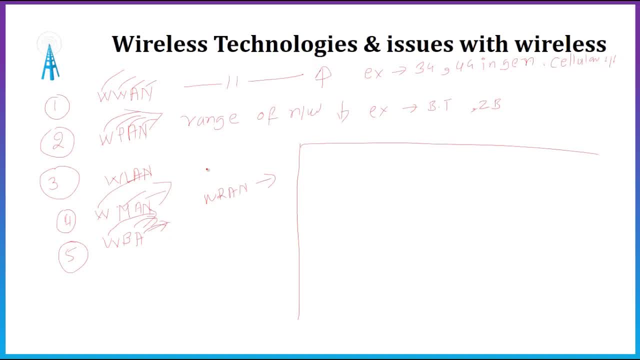 whenever they want it. so technologies like 3g, Wi-Fi, WiMAX, UWB, they work together to meet a unique customer need. okay, so WBA is actually a point to multi point system. so always remember WBA is your WPA network and it is always a device which is connected to your system. 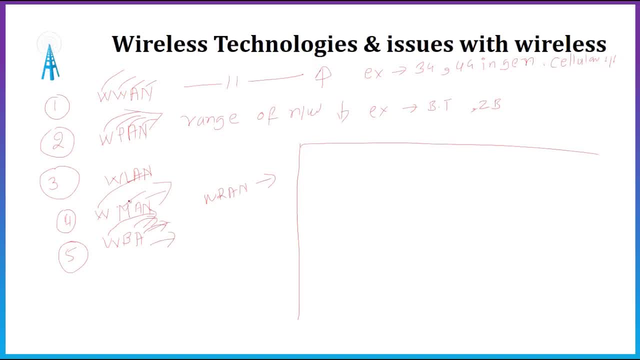 is because this is a important part of w man, wba. these are actually an important part of what we are going to study today, so consider this to be a point to multi-point technique. okay. so wba is point to multi-point system. okay, in which, uh, it is actually a made up of like. 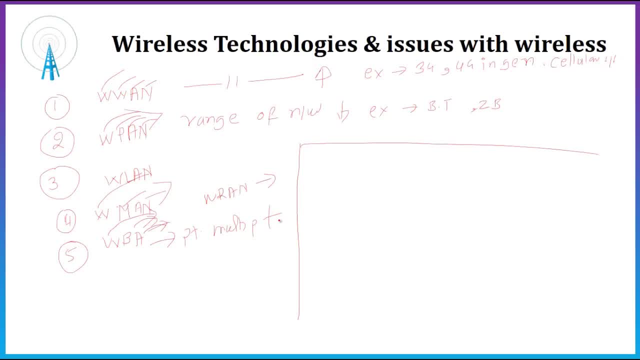 base station and subscriber equipment. so instead of using a physical connection between base station and a subscriber, the base station uses a outdoor antenna to send and raise your high speed data and a voice to subscriber equipment. so wba offers actually a very effective complementary solution to wireline broadband. so, uh, which has actually become a globally recognized by your. 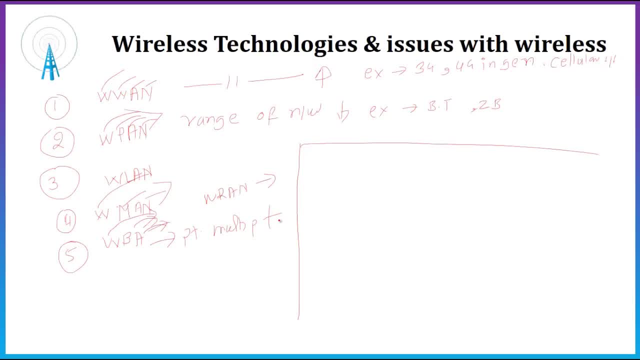 uh, higher percentage of population. okay. so basically we need to understand now what are the different issues that have been considered while uh considering wireless networks. so what are the different issues? so i'll just write issues with wireless network, okay. so we'll just cover it one by one. so quality of service then. 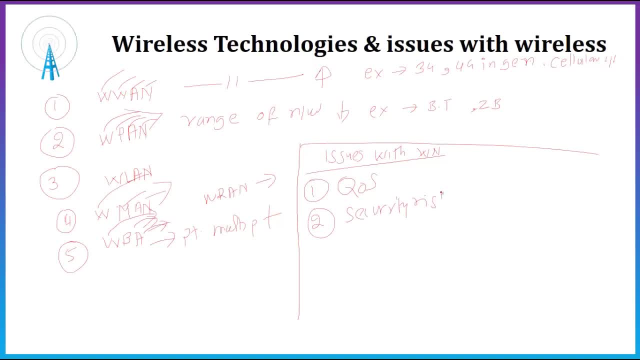 security risk always there, so we need to consider that parameter. and last one is actually, uh, reachable range. okay, so what is qos? so qos is actually your quality of service. so one of the primary- we could say, yes, primary- concern about your wireless data delivery is that, unlike the internet, through the wired services, quality of service is actually inadequate. okay, 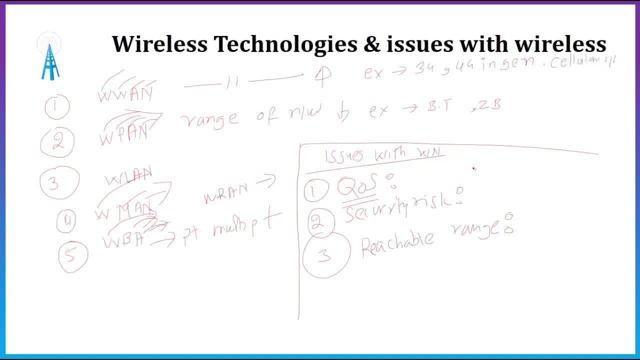 so lost packet and atmospheric energy or whatever interference they recur a problem in actually your wireless protocol. so quality of service is always a important parameter that we need to consider. then again, the security risk. so this is actually another major issue with your data transfer over a wireless wireless. 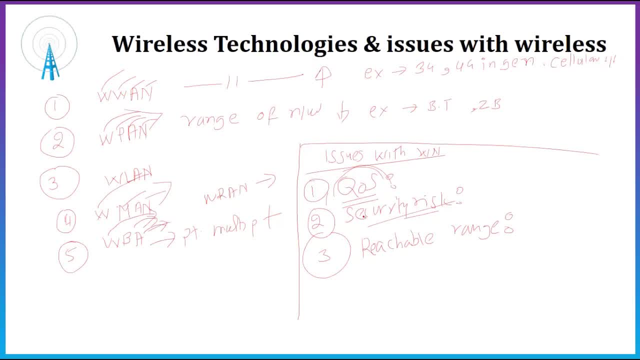 network. so basic network security mechanism like a service set identifier, like what we in generally say as SSID and all those things and wireless wireless equivalency privacy. so I think we- you have heard maybe WEP, so these majors may be adequate for a residence and a small. 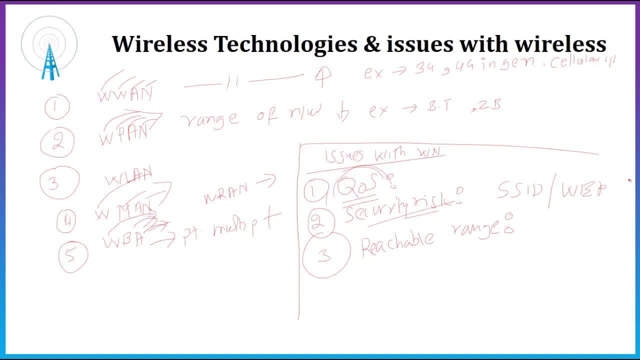 business, but actually they are inadequate for your larger entities, like where you require more security. so only SSID and WEP will not work. so that's why, again, it's an issue with your wireless network. that security risk is there. again, the important phenomena is your reachable range, so normally 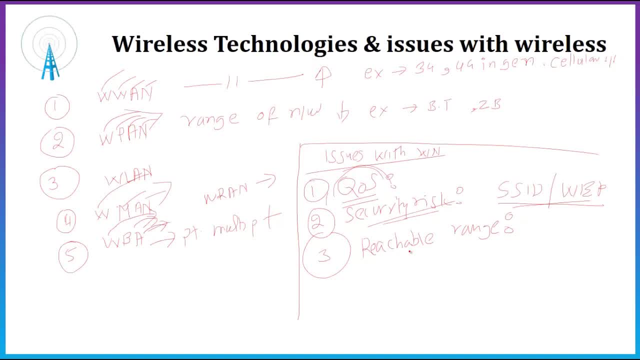 wireless network offers a range of about 100 meter or less. okay, so the range is actually a function of your antenna design and again a power. so nowadays the range of wireless is actually extended in a tens of miles. so that, so that this application is working, because in other situations you can operate ableLAN. 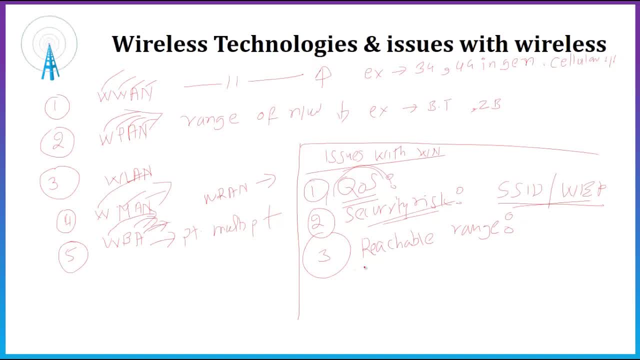 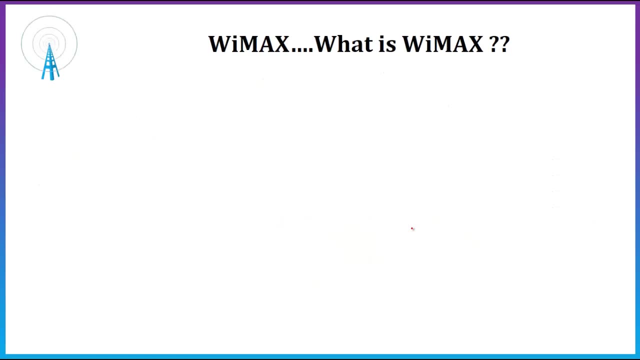 especially a service device, but in your MWB or hardware owners and those kind of options it is not really a mainstream option- although this should not be an issue anymore, I suppose- but still it becomes actually viable option that a reachable range is actually always limited. okay. so I think. 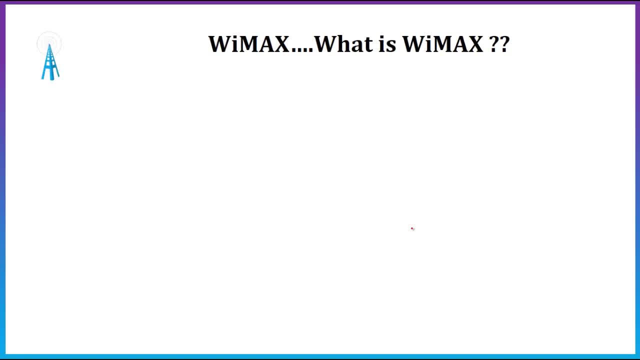 now we are ready to move on with what is y max, so, yes, what is a while max. so I think first, so Wi-Fi is actually your wireless fidelity. so Wi-Fi is based on your I, triple eight, zero, two point one, one family of standard and is actually we. 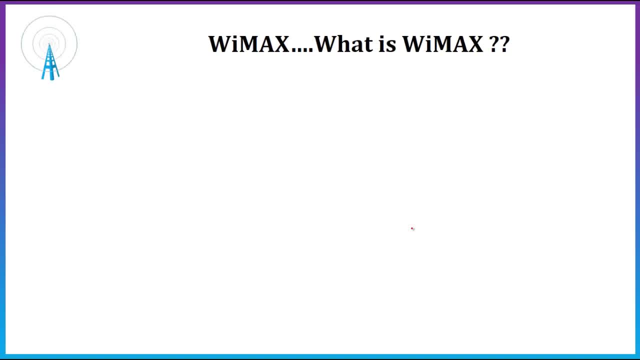 could say primarily a local area network, but wireless. so the technology is be that Wi-Fi technology is designed to provide, we could say, in building broadband coverage. okay so, but we are here for a WiMAX. so what is a WiMAX? so WiMAX is actually one of the hottest broadband wireless technology around. 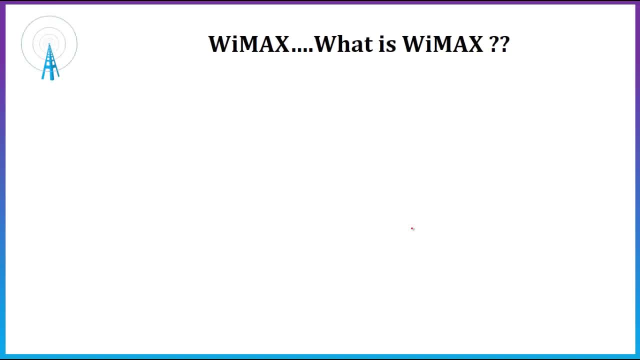 today. so WiMAX systems are expected to deliver broadband access services to residents as well as to enterprise customer in economical way. so loosely we could say that WiMAX is standardized wireless version of your Ethernet intended intended to- we could say primarily- as alternative to your wire technology, like your cable, modem, DSL, then your t1e1 links. 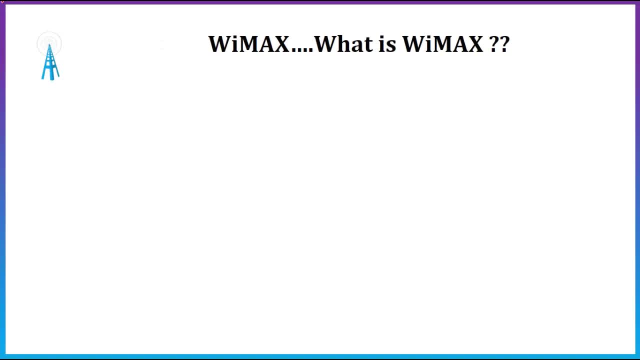 so I think you understand what is mean by your DSL and what we say is: okay, I'll just write it down. what is DSL? so I think you know of a form of it. so this is actually a digital subscriber line. okay, so digital subscriber line is like: 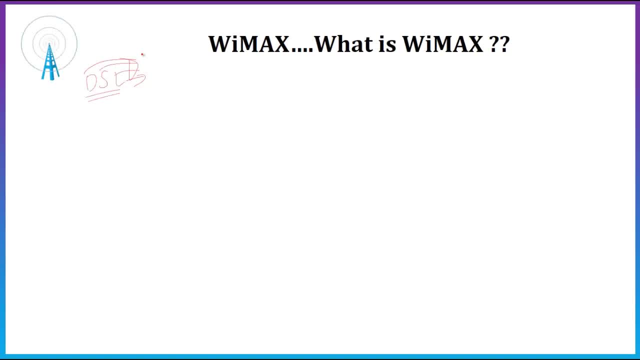 your what we used to get broadband like for through your telephonic company, so that used to be called as a DSL. okay, so in that. actually, there is one more thing that is mentioned before also. that's a diagram of this one. so this pattern was actually can be seen on the, on the WiMAX one and the other one called E1, and even. 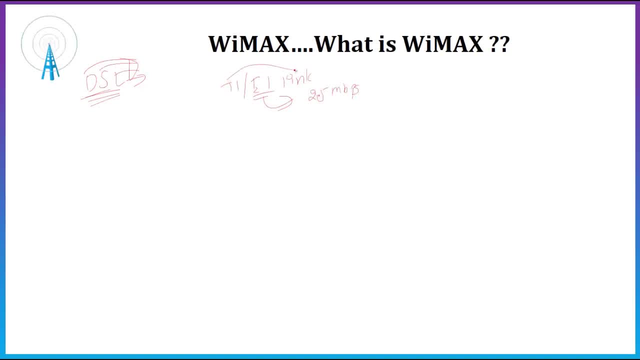 links. so out of is this? even link is actually used to provide like approximately 2.5 MAPs of speed, and this one was actually your half of the half of the rate of this. okay, so these were many links were there before this Wi-Fi and all those things. 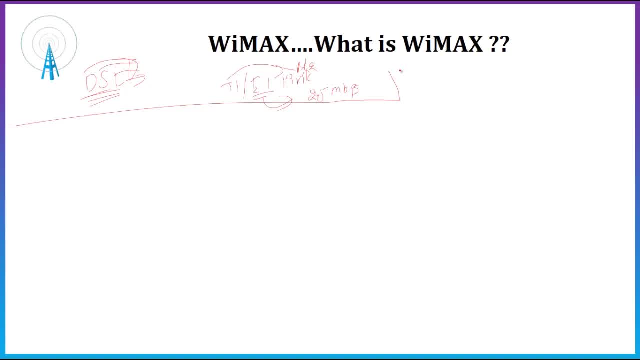 technology. okay, to provide you a broadband access at a customer's premises. okay, so don't consider this to be a wi-fi. i am just writing it as a wired broadband. okay, so consider this to be a wired one. don't consider this to be like for your wireless or your wi-max. so there is one more. so, whenever 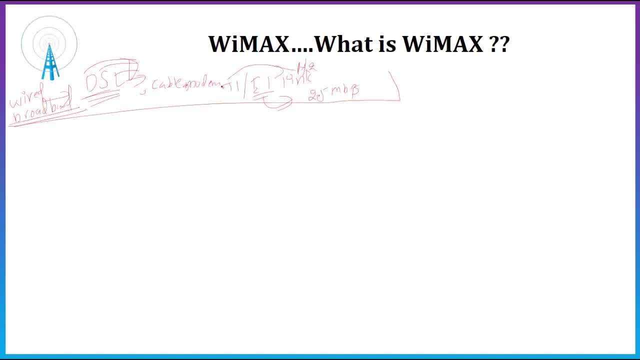 you refer it again. so there are actually cable modems. okay, so we are ready to move on with wi-max. so, most likely, uh, your wi-max is actually a industry trade organization which is actually formed by a leading communications and component, or we could say a equipment companies to promote. 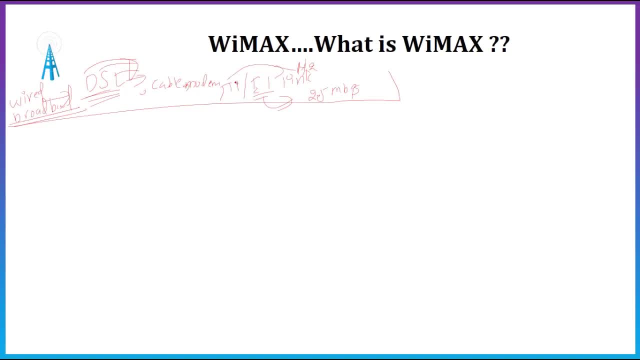 and certify your compatibility or interoperability of your broadband wireless access equipment. that confirms that i triple a 802.16 and, uh, your hyperman standards. so wi-max would operate similar to wi-fi, but at higher speeds or over a greater distance for a great number of user. okay, so wi-max has actually ability to uh provide. 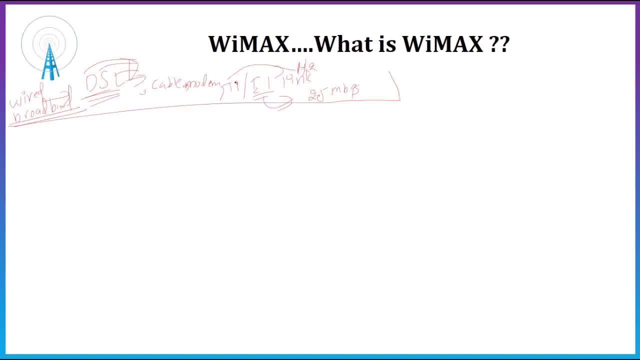 service, even in areas that are difficult for your wired infrastructure to reach, and the ability to overcome that physical limitation or traditional wired infrastructure. so wi-max was actually formed in- uh, approximately- i don't remember exact month, but i think in a march or april of 2001. 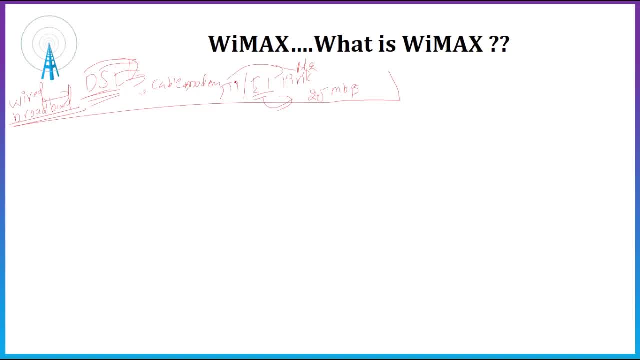 it was formed in anticipation of your publication of uh, what would say 10 to 66 gigahertz, ieee 802.16 specification. so wi-max is uh 802.16, as wi-fi alliance is to like 802.11. so uh again. what is ymax? 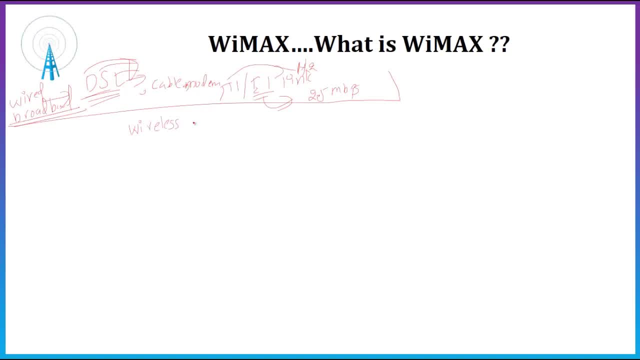 so it is wireless inter operability, okay, interoperability for microwave access, okay, so this is your y max, okay, so it is actually based on. so it is actually based on your what we could say w man- wireless metropolitan area network technology. so this wire technology, wireless technology, 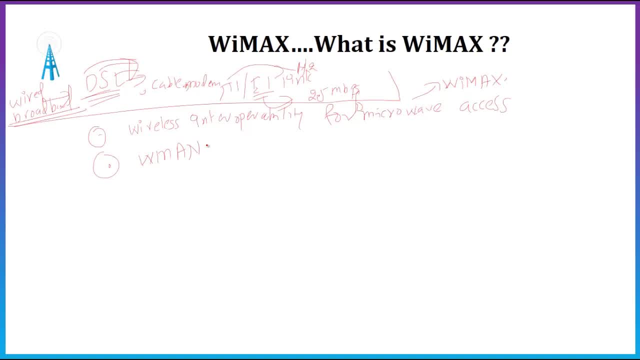 is optimized to deliver a ip centric services over a wide area. then the certification. that denotes interoperability of equipment built in your IHH802.16 or compatible standard. the IHH802.16 2.16 working group develop standards to address two kind of usage model. so there are again. 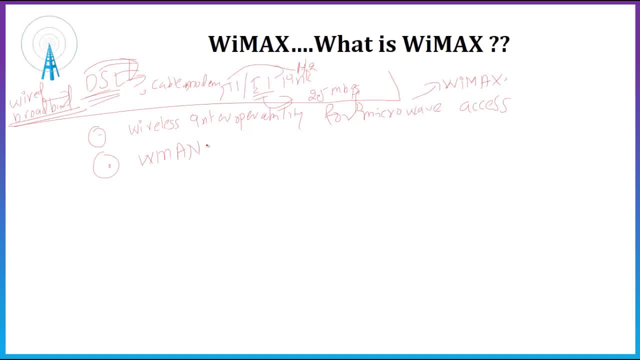 or two different usage model. so one is- I suppose I will just write ymax usage model. so there are actually two. so one is actually your IEEE 802.16-2004, another is IEEE 802.16e. so these are actually different things. so this is called as our fixed usage model and another way is: 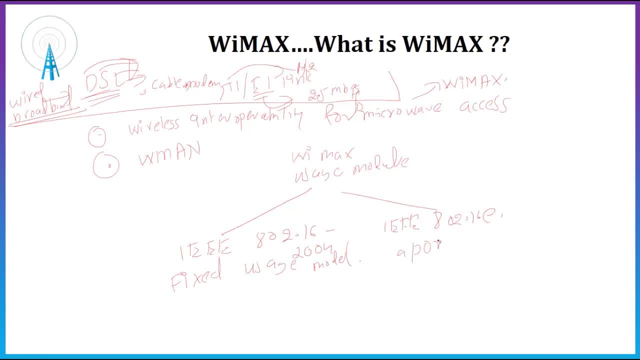 actually a pole table space, portable, a portable use itch order. ok, so this is fixed. well, this is a portable one. so what is then 80 two point 16 e? so there was again a new thing that came into picture. so what is this thing? so we'll come up with that. so 80, 2 point 16 a or Y, max is 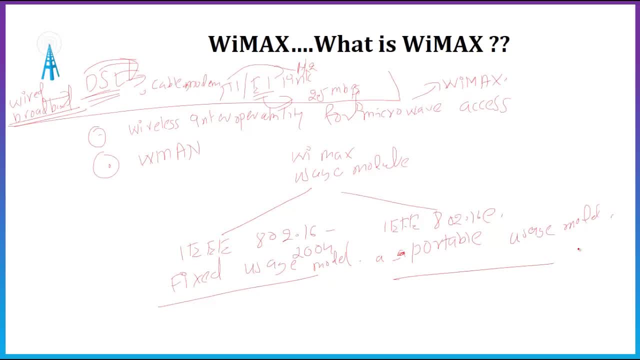 actually a shared usage of embeds happens to a shared usage of embeds, However, there are actually- we could say WiMAX is easy terminology for that- people to tend to use for a 802.16 standard and technology themselves, although strictly it applies. 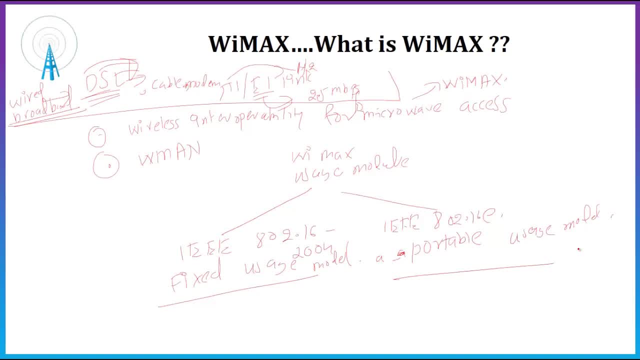 to only a system that made a specific- what we could say a performance criteria laid down by your WiMAX forum. so 802.16, a standard is for like 2 to 11 gigahertz. okay, so if you just need to remember, I'll just write it on 802.16. 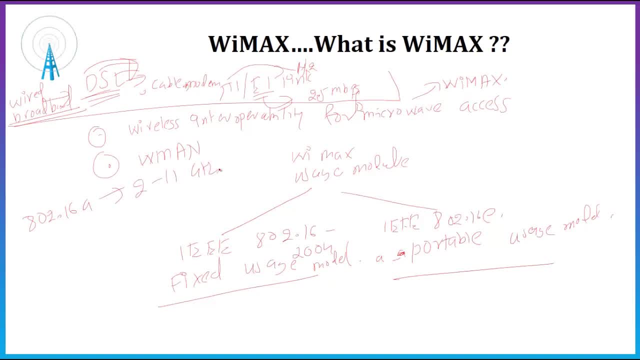 is for your 2 to 11 gigahertz. okay, so it's actually a wireless man. so wireless metropolitan area network, which is operating with a range of with a standard of 2 to 11 gigahertz, but technologically that will provide a broadband wireless. 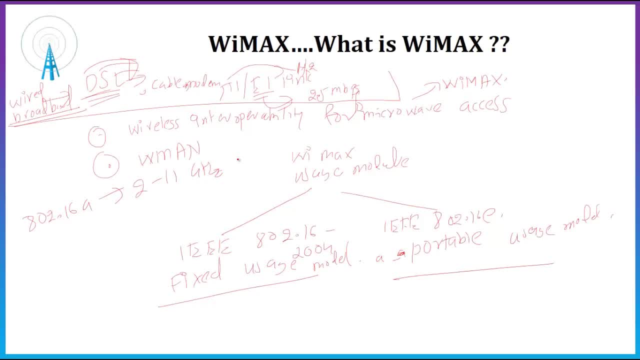 connectivity to a failure of wireless connection and not a failure of wireless connection. I always fixed portable and nomadic devices okay, so it can be used to connect 802.11 a hotspots to the internet, provides a campus connectivity and to provide a wireless alternative to your. 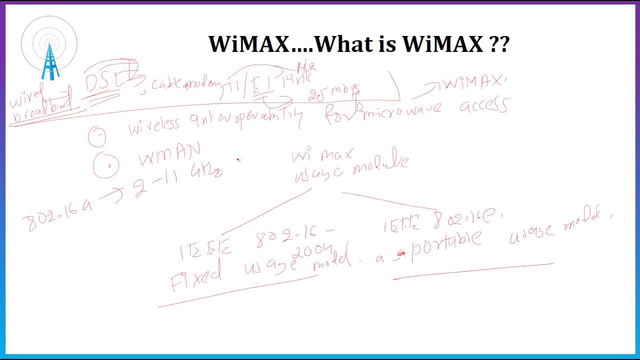 cable or and DSL for a last mile broadband access. okay, so WiMAX? you will ask then, what is the speed of your WiMAX? so WiMAX is actually expected to offer initially up to about 40 kbps capacity per wireless channel for both fixed and, obviously, for a portable application. 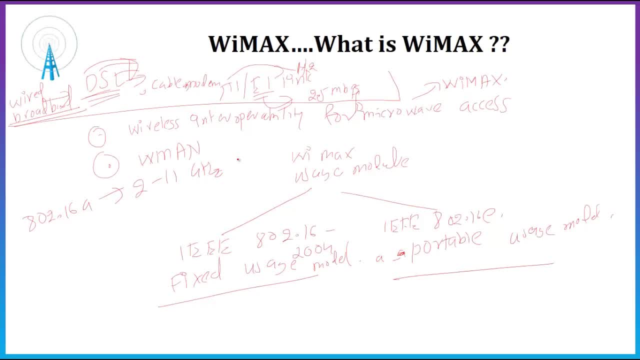 depending upon a particular technical configuration chosen enough to support hundreds of businesses with T1 speed connectivity. okay, so thousands of residential DSL speed connectivity. so WiMAX can support your voice as well as video for as an internet data. so why my is developed to provide actually a wireless broadband access? 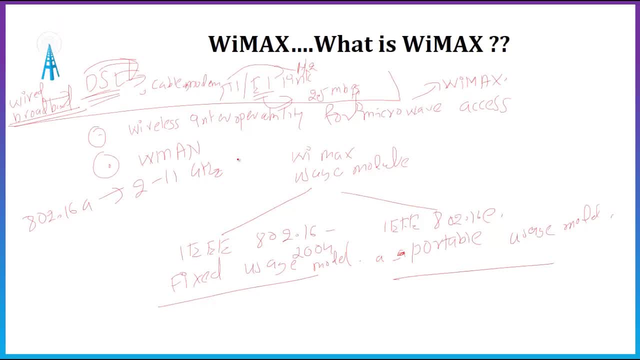 to building, or we could say either in your competition of existing your wired network, or alone, currently we could say, in a rural or thinly populated area, so it can be used to connect wireless LAN hotspot to internet. and again, WiMAX is also intended to provide a broadband connectivity to mobile devices. so it would not be as fast as that these fixed. 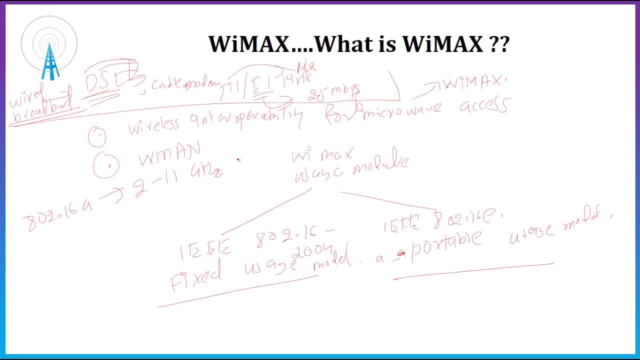 application, but expectations are about like 15 mbps capacity in a 3 kilometer of cell coverage area. so with WiMAX user can really cut free from today's internet access arrangement and will be able to go online at a broadband speeds almost whenever they like from a metro within a metro zone. so WiMAX could potentially 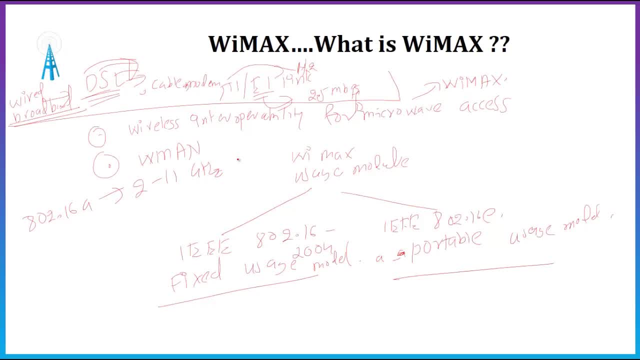 be deployed in a variety of spectrum bands like 2.3 gigahertz, 2.5 gigahertz and so on: 3.5 gigahertz or five point 8 gigahertz. okay, so you in general consider this again. remember many of the time it's a common confusion that whether WiMAX is operating on 2.4 gigahertz 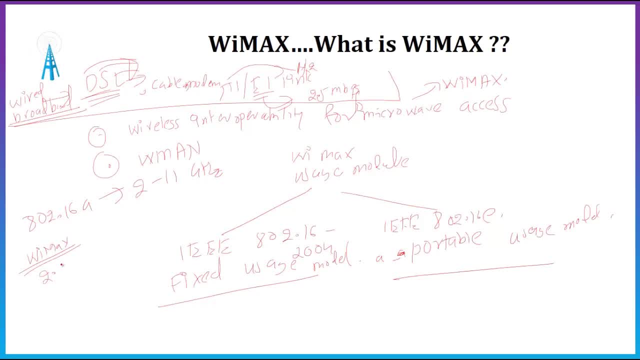 or not, so obviously it's not true. so WiMAX operates at 2.3 gigahertz. okay, then next is your 2.5 gigahertz, then 3.5 gigahertz and then, just like before, like 3.6 gigahertz next. 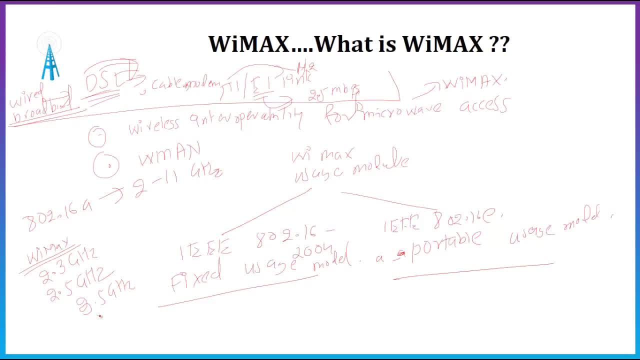 is your 5 gigahertz and then 6 gigahertz and then 7 gigahertz. so the whole thing is divide and your 5.8 gigahertz. so these are the four different variants. so basically the question arises again that why? why ymax? okay, so actually ymax can satisfy a variety of access needs. 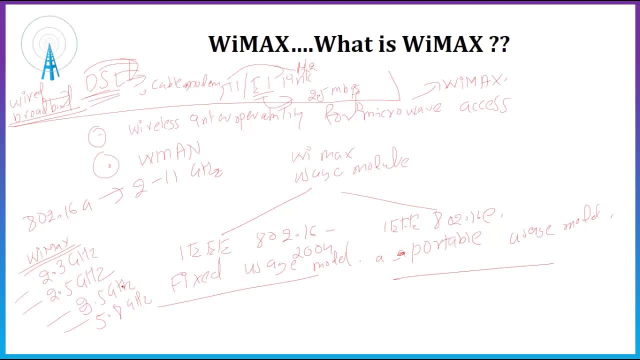 uh potential applications, including extending your broadband broadband capacity or capabilities to bring them uh closer to subscriber, filling gaps in your cable, dsl or t1 services, uh your wi-fi, your- what we could say a cellular black hole backhaul processes, or providing uh last 100 meter access from a fiber to curve and giving the service providers another cost-effective 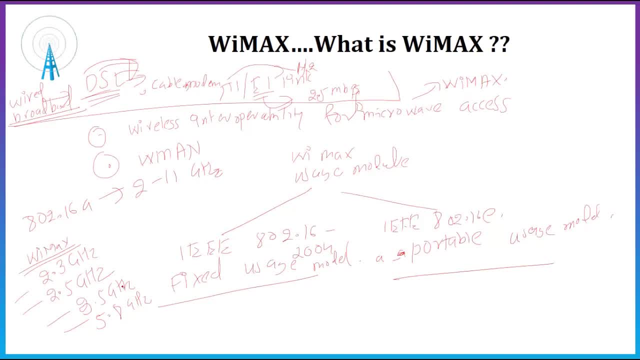 option for supporting broadband services. so why can? ymax can actually support a very high bandwidth solution where a large uh spectrometer can support a very high bandwidth solution where a large spectrometer can support a very high bandwidth solution. where a large spectrometer can support a very high bandwidth. 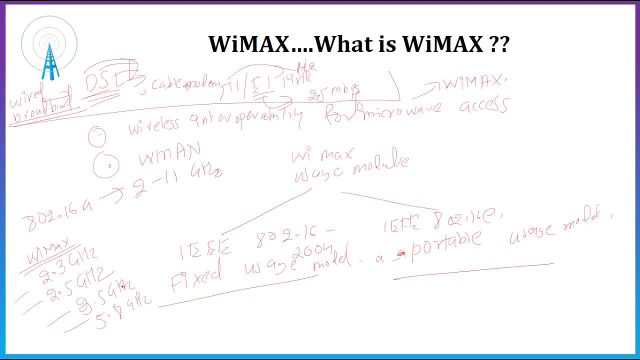 deployment, that is, like your greater than your 10 megahertz are desired, using existing infrastructure, keeping costs down while delivering the bandwidth need to support a full range of high value multimedia services. so why it can actually uh helps- uh, it can actually help you to provide or to meet many of the challenges they face due to increasing number of customer demand. 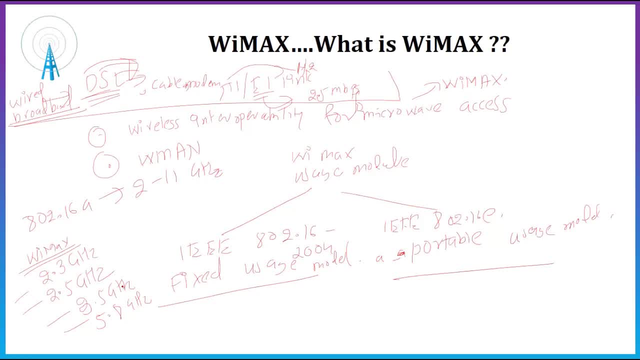 so, without discarding their existing infrastructure, uh, uh, whatever investment they have made. so they don't want that thing to be avoided, or they don't want to raise that cost. so that's why, uh, depending upon customer demand, without discarding the existing infrastructure investment, because it has actually ability to seamlessly interoperate across. 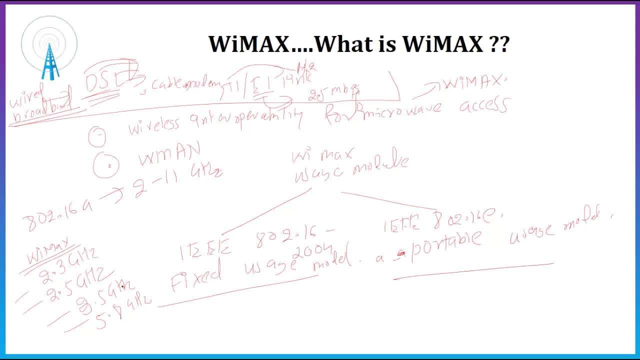 various network types. so ymax will be always useful thing. so ymax again can provide you a wireless uh wide area, uh area of service to your customers. so that's why they don't want to raise uh wide area, uh area of service to your customers. so that's why they don't want to raise. 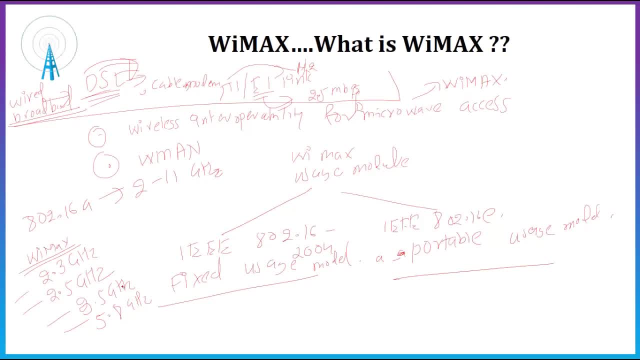 so the quality of service, capability for application, ranging from like real-time data, sensitive voice over ip, so vip, and real-time streaming of video and non-real-time downloads, so uh, these kind of expectation can be carried out again. uh, i could say a last point in ymax, uh, ymax, which is actually ip based wireless. 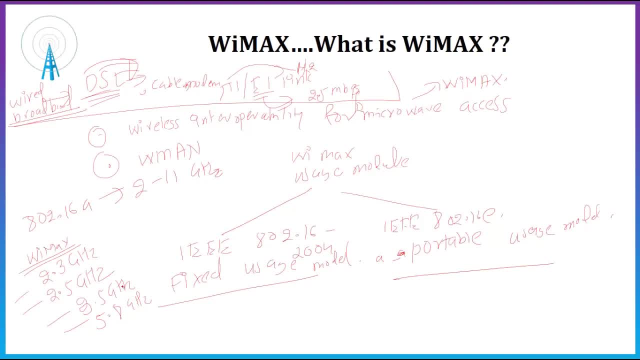 broadband technology. it can be integrated into both, like wide area, third generation mobile and uh wired- uh, we could say wired one or wireless network, allowing it to become a part of any- uh seem part of- a seamless, anytime, anywhere broadband access solution. so, ultimately, wi-fi is actually 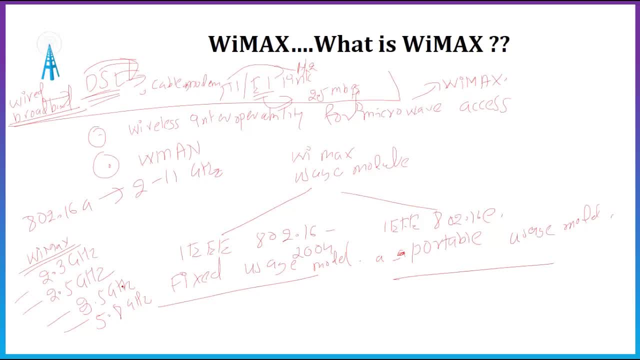 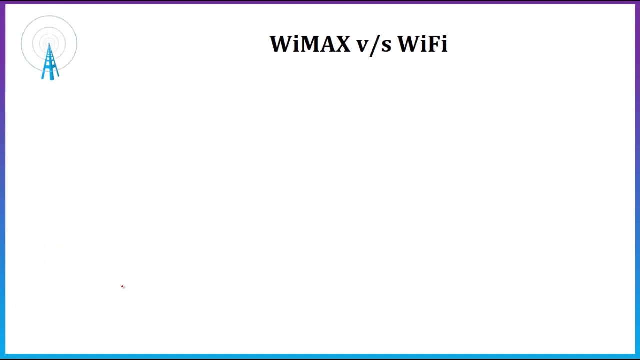 intended to serve as a next step in evolution of your 3g 4g phones. uh, then, potential combination of your ymax and cdma standard is actually nowadays it is called as a 4g. okay, so now what is actually difference between your wi-fi and wi-max? so there are actually variety of different. 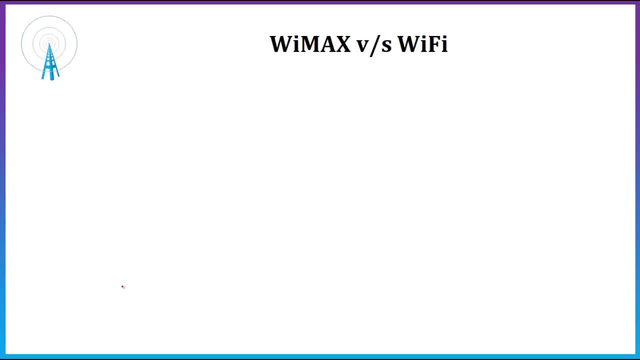 parameters that we need to consider while we are dealing with wi-max and wi-fi. so wi-max is actually- we could say it is- similar to the wireless standard known as your wi-fi, but on a much larger scale and a faster speed. a nomadic version would keep wi-max enabled devices. 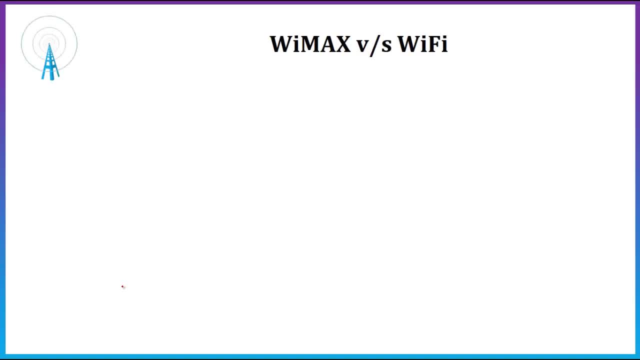 connected over a large area. so much like uh, today's cell phones, uh, that could be a better example. so we can compare uh on different parameters. so like range, scalability, bit rate, quality of service, so there could be many parameters that we need to consider. so let's consider uh factor one by one. so first one is: 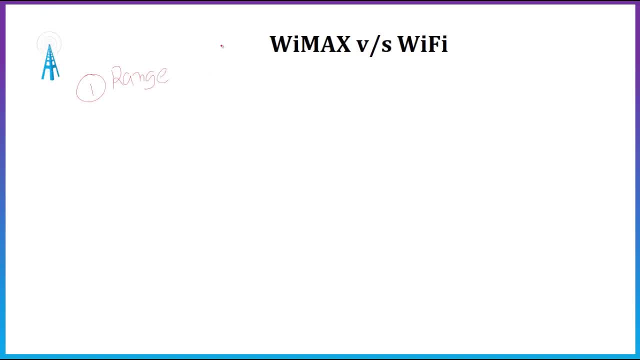 your range. so what is range? so wi-fi typically provide you, uh, local network access for few hundred feet uh, with a speed of like 54 mbps. okay, so 54 mbps- that we have already seen that how which version can be used to get a 54 mbps? a single wi-max antenna is expected to have. 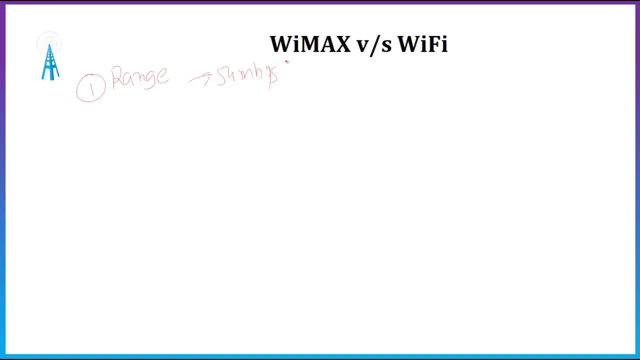 a range up to 40 miles and a speed of 70 mbps or more. 70 is actually a basic. i'm saying so as such could say bring the underlying internet connection needed for a service like local wi-fi network. so here it was 54 mbps and here it is 70 mbps for a single node. okay, i'm just saying wi-fi. 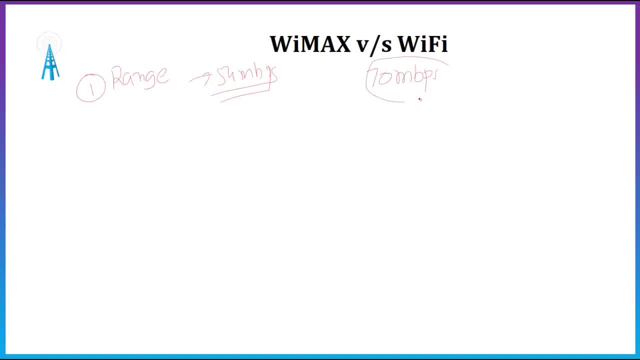 single wi-max antenna. for single wi-max antenna 70 plus, then again i'll compare with one more parameter called as scalability. scalability will be like uh wi-fi is actually intended for a lan application or user scale from one to ten. which subscriber for one cp devices? 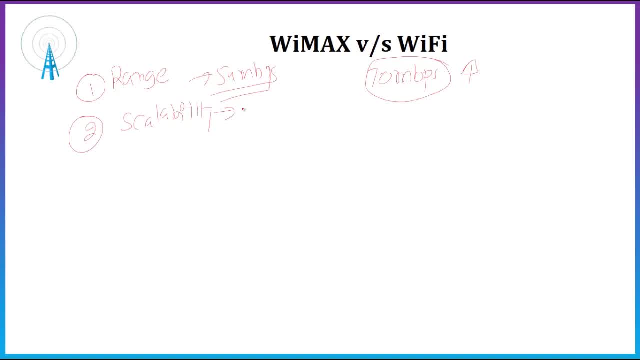 so fixed channel size is like of 20 megahertz actually, and in case of wi-max it is designed to efficiently support from one to hundred of consumer premises equipment. so cp is actually your. cpe is actually consumer premises equipment. okay, so that is actually called a cp, it's always. 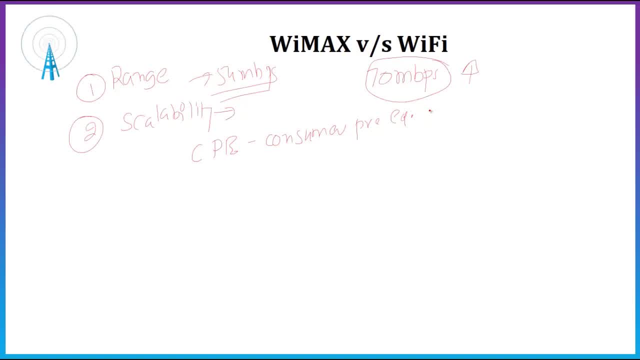 uh, remember this shortcut, so i just forgot to tell you. so wi-max is actually designed to efficiently uh support one to hundred cp with unlimited subscribers. behind each cp, individual cp. so the flexible channel size is from like 1.5 megahertz to 20 megahertz. so 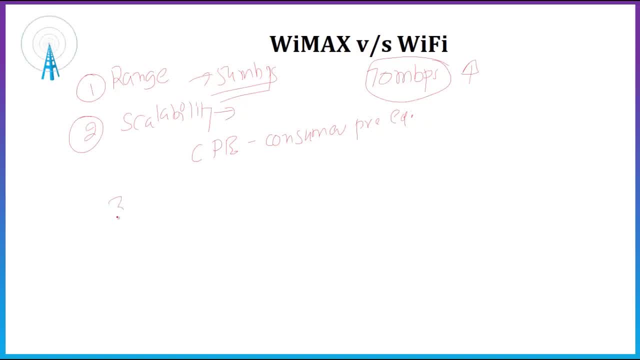 again, scalability is covered. so third one is actually your bit rate. so bit rate in wi-fi is like 2.7 bps per hertz and peak up to like 54 mbps in 20 megahertz channel. so uh, wi-max would be like 5 bps and 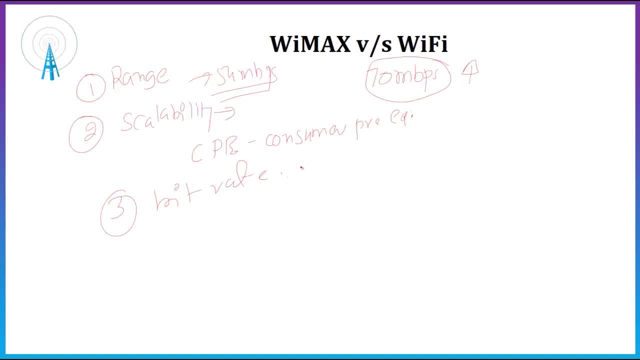 peak of 100 mbps in 20 megahertz channel. okay, so there's a slight difference. so quality of service wi-fi doesn't guarantee you okay. so whenever it comes out to be a quality of service, your wi-fi technology doesn't guarantee you to provide you a any quality of service. but whereas in 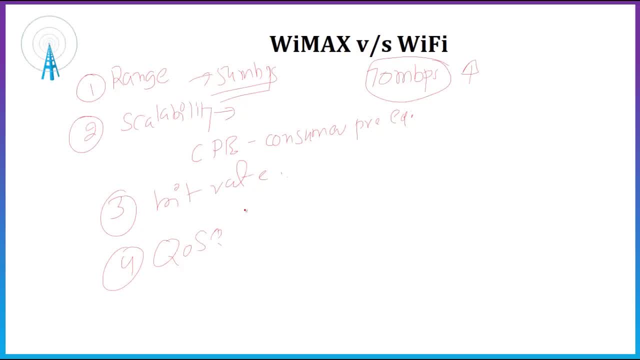 wi-max, it will provide you several levels of your quality of service. as such, uh, wi-max can actually bring the underlying internet connection needed for a service of your uh local wi-fi network. so wi-fi doesn't provide, uh, what we could say uh ubiquitous broadband, while wi-max does provide you. 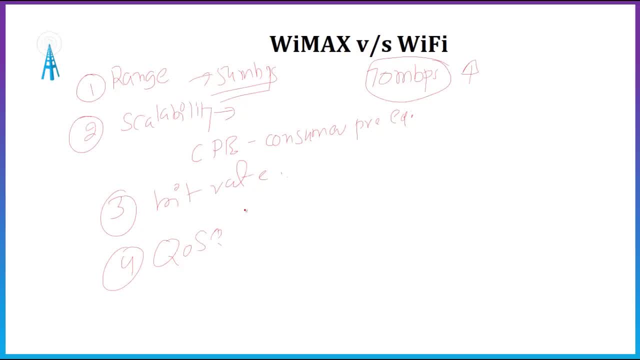 that kind of thing. so wherever in a comparison, uh like whether you compare your wi-max 802.16a with uh whatever a, b, g thing, things are there for wi-fi. so we'll see on a comparison, uh like for your primary application of those things. so you know. 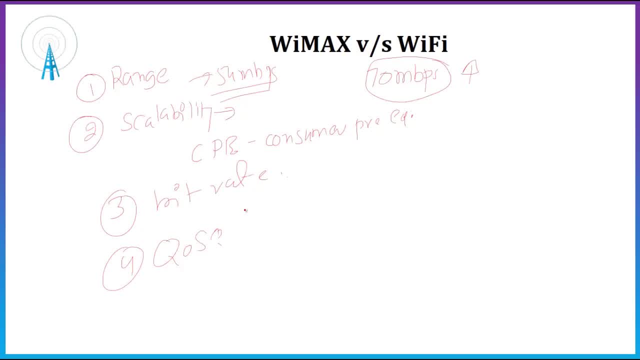 primary applications frequency band. you obviously know that 802.16a is operating on 2 to 11.. your other standards of wi-fi were operating on 2.4 gigahertz or maximum. in case of g 802.11g it was operating on uh 8 gigahertz uni band. so uni is actually- now you know it's- unlicensed band. so 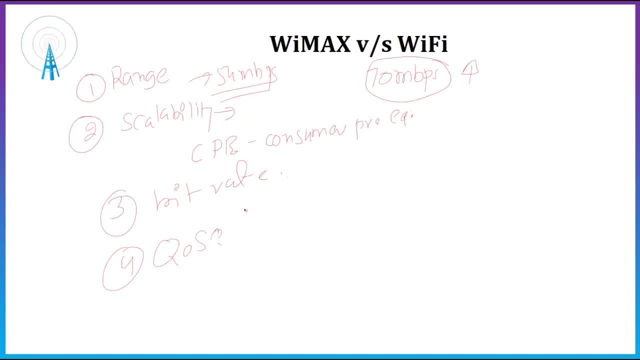 it is variable. in uh wi-max it is 1.25 to 20 megahertz, but whereas in that case it was like 20 megahertz or 25 megahertz. so this is actually you could say wi-max is an important parameter. 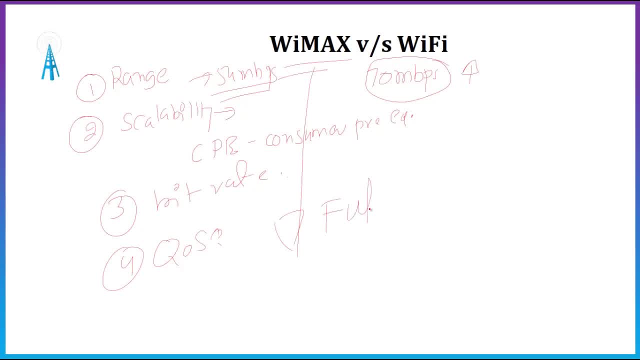 which i forgot to tell you. this is actually your full duplex systems. okay, wi-fi is not a full duplex system, but these systems are actually half duplex, so i just forgot to mention this parameter. so always consider your wi max to be a full duplex systems. okay, and uh, these actually use radio technology, like uh, ofdm, and they have a. 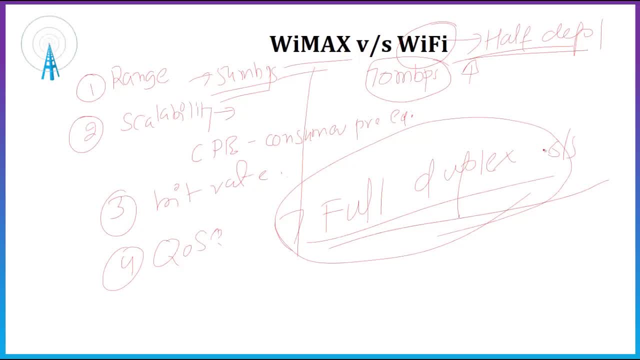 what we could say forward error correction techniques are: the encryption is actually aes or 3des. is there optional encryption in your ymax but mandatory is actually 3ds? so what we could say then again, access protocol, uh, what we used to study in our ccn or computer communication networks. so 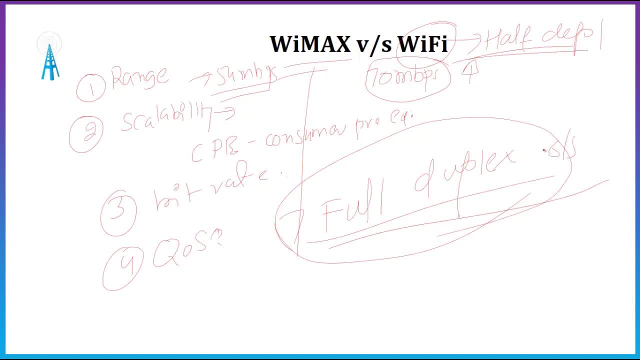 i think you might have gone through like csm, csm techniques, csmsca. so they were used in your wi-fi, but whereas in 802.16a or in ymax it is actually a request and grant kind of thing. so this is all about your ymax and a wi-fi. so what are the salient features of? 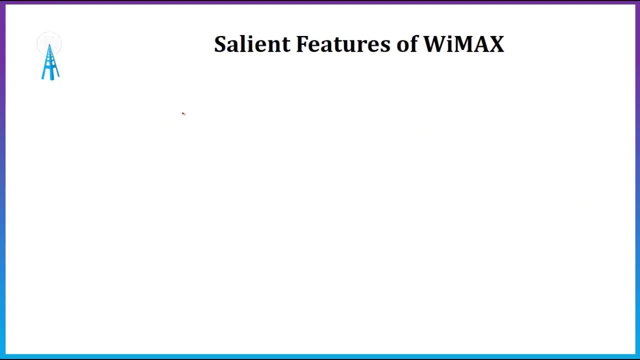 your ymax. so uh, what? we could say that directly getting into those things. okay, fine, i'll just get into this. so ymax is actually your wireless broadband solution that offers a rich set of a feature with a lot of flexibility in terms of your deployment of option, then potential. 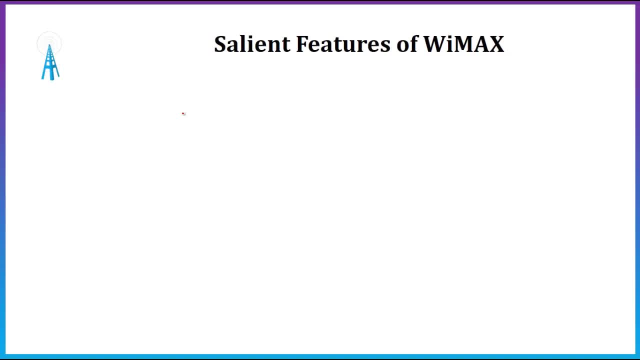 offering and some of the more salient features, uh, that deserve highlighting as as such. uh, we could say, uh, it provides actually two forms of services. so i could just simply, in a shortcut, write: services, so two form of services. what are those two forms? so one is actually. 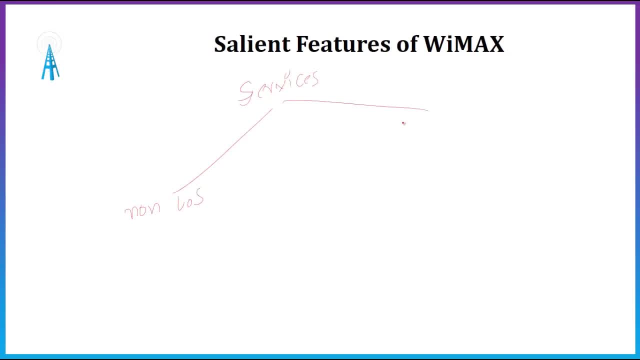 non-line of sight and second, one is actually line of sight. so obviously, non-line of sight means: uh, the one is series is a point, and the other is a line of sight. sorry, line of sight means a point, so for an antenna to stop. so here, for example, if you are connection and if it is a line of 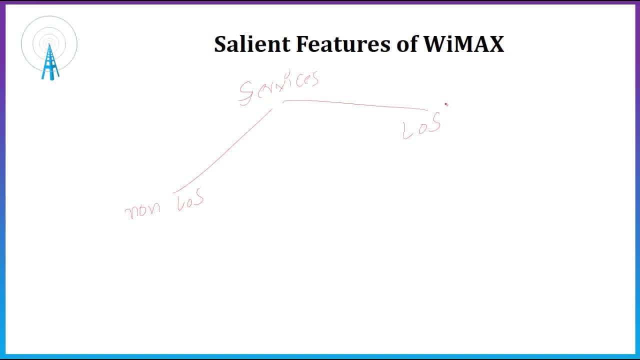 sight. uh, then it will start a line of sight. the why this i'm showing you as a small one that is, is A service. uh, service is actually wi-fi sort of service. uh, here, a small antenna on your computer connects to a wi-max tower. in this mode, wi-max uses a low frequency range of 2 to 11. 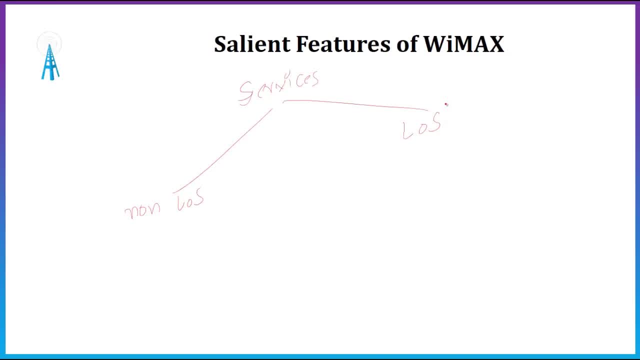 where a fixed dish antenna point straight to your ymax tower from your rooftop or a pole. the line of sight connection is actually stronger and more stable, so it's able to send a lot of data with fewer errors. so line of sight transmission uses actually a higher frequency with a range. 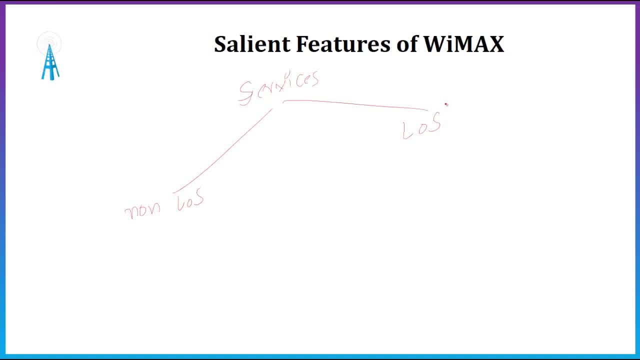 reaching possibly like 66 gigahertz. obviously you can understand that, which technique is better, so obviously line of sight is better, but again that kind of placement needs to be made. so again some of the feature I could mention is like: Oh, FDM, there is the physical layer, physical layer, so 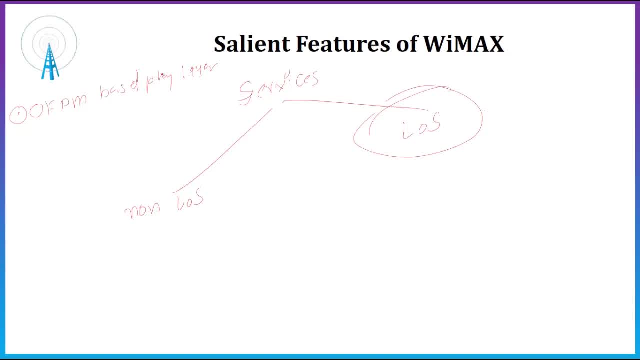 ymax physical layer is actually based on your orthogonal frequency division multiplexing. now, if I need to tell or game in short, so I would in this actually a scheme that offers a good resistance to multipath, and in this case it's actually. it allows ymax to operate in a and non-line-of-sight condition. okay, so again these. 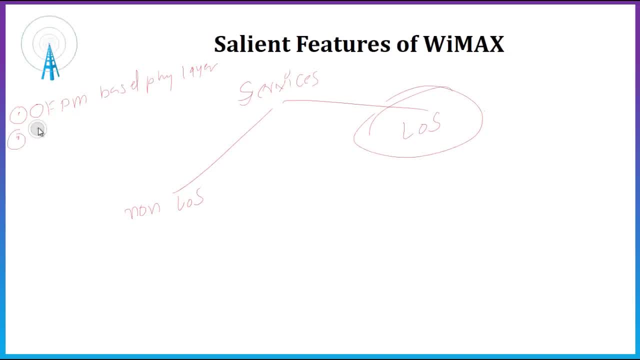 another parameter which is called as hi. I'm not writing entirely high peak, they direct ok, so mx is actually capable of providing you very high data rate, like, in fact, peak physical data rate can be as as high as like your 74 mbps and operating using like your 20 megahertz wide. 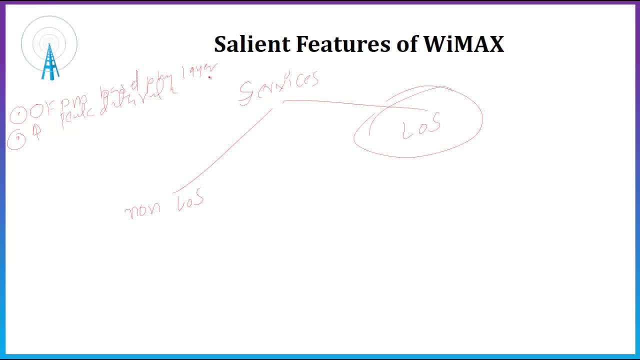 spectrum. so more typically using uh 10 mega spectrum, using tdd scheme, uh with a, but we could say three is to one. uh download to uplink ratio. the peak physical data rate is about like 25 mbps and 6.7 mbps for the downlink and uplink respectively. so 27 would be your downlink and 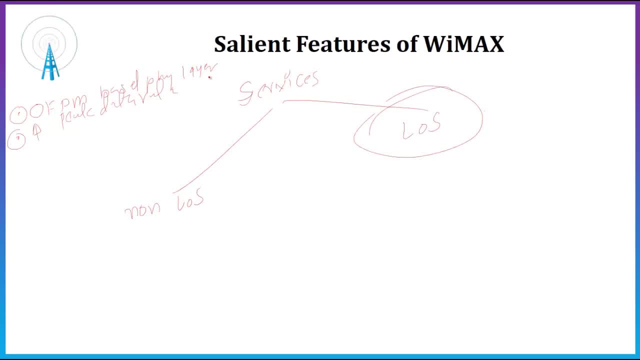 uplink would be like 6.7. then again, there are many parameters like scalable bandwidth and data rate supports, so there is like 128- 512 and different bit supports are there. so again, uh, it does have some kind of what we could say adaptive modulation coding. so here let me just consider these features. 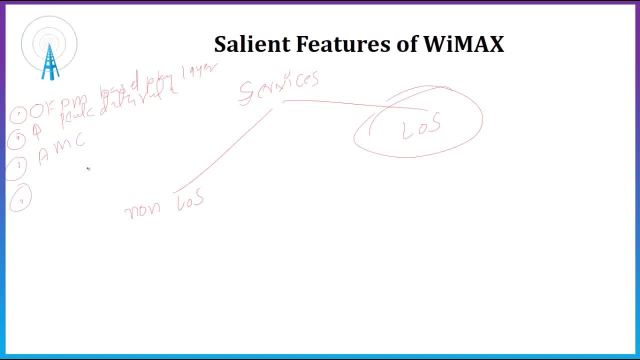 adaptive modulation coding. okay then. uh, what happens with these kind of things? so amc is actually effective mechanism to maximize your throughput, uh, in a time varying channel, okay, so again, there is uh something called as your link layer retransmission, link layer retransmission. so what is this? link layer retransmission is actually so. 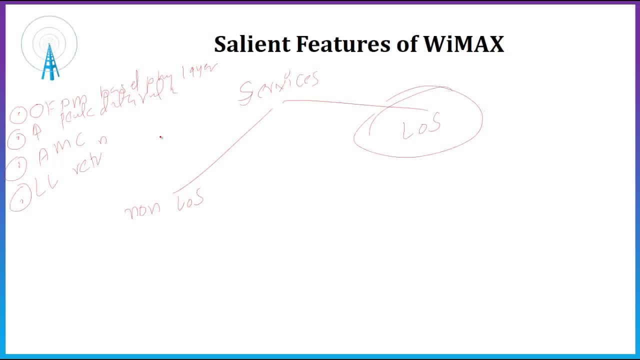 ymax supports automatically retransmission request. so whatever we call as a arq request, uh, that supports arq at the link layer from connection that requires a enhanced reliability. okay, so this again supports you. like. if i need to consider a parameter, so it will be like: tdd and fdd supported. 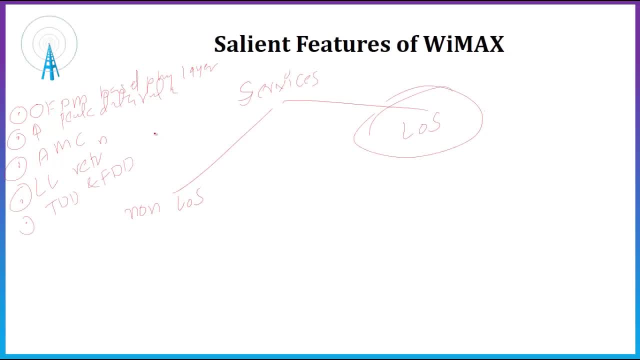 time division duplexing and frequency division duplexing, so just to make a low cost implementation. then again the the link layer retransmission also supports, like you already saw, the link layer retransmission. then this function is actually a dynamic. as for resource allocation, that we have already seen. quality of services there, then the robust security. 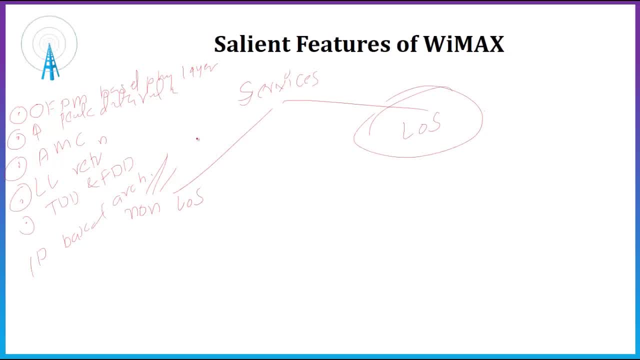 is there? support of mobility is there? uh, and i think i just forgot one thing. uh, it's actually a. a WiMAX forum has defined a reference network architecture that is based on all IP platforms, so all end-to-end services are delivered over an IP architecture relying on IP based protocols for end-to-end transport. okay, 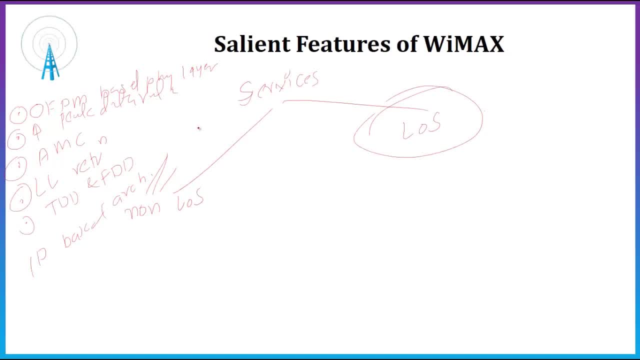 so end-to-end transport, then again with for your quality of service, then session management, security and mobility. so it was actually a better advantages that to used with your IP architecture. so now we'll move on to the next building blocks of your WiMAX. so WiMAX has actually building two different building blocks. 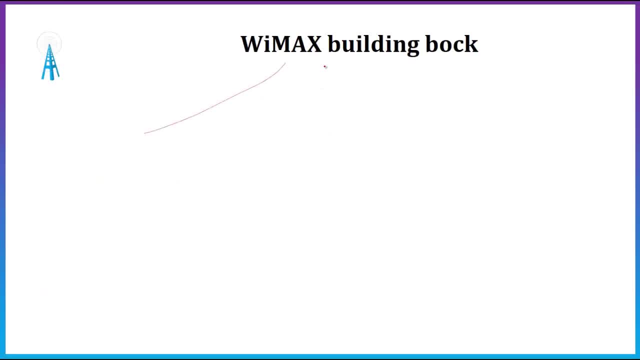 so we could say they are. there are two building blocks. one is actually called as your BS and another is called as your receiver. so what is BS? so it is actually a WiMAX base station. why am I the base station and this is your WiMAX receiver? WiMAX, there is okay. 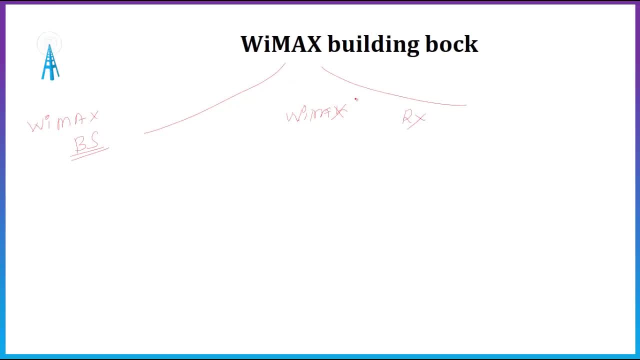 so what is WiMAX base station? so WiMAX base station is actually a consists of a indoor electronics and WiMAX tower similar to that of like your cell phone tower. okay, so there will be indoor electronics plus, your antenna should be connected to your WiMAX base station and this is your. 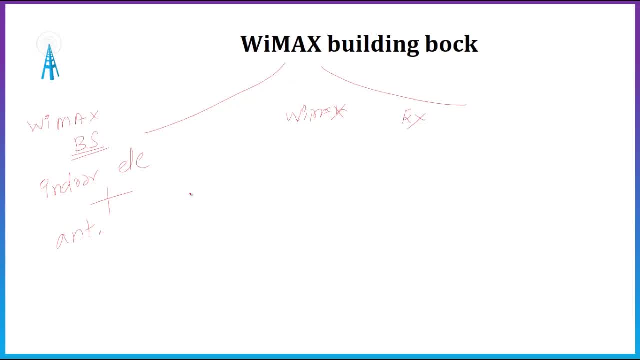 would be there. so instead of tower, I'll just write it down as an antenna. okay, so WiMAX base station would you use? Mac Lair, defined in a standard common interface that makes network interoperable and would allocate uplink and downlink bandwidth to subscriber according to their need. so on a essentiality, on a 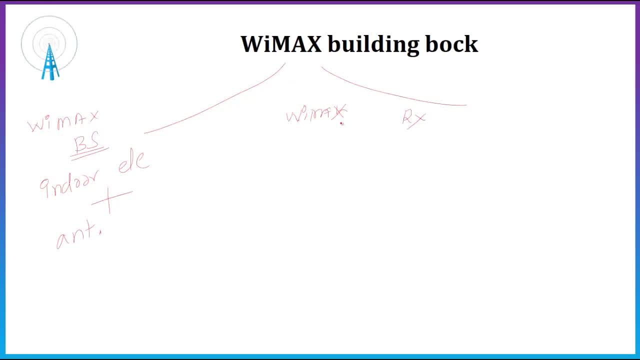 real-time basis. so each base station would provide a wireless coverage over area area. we could say that thing to be a cell, okay. so, uh, each station would be provided with a wireless coverage over area, which is also called as a cell. so in general, theoretically, we could say: 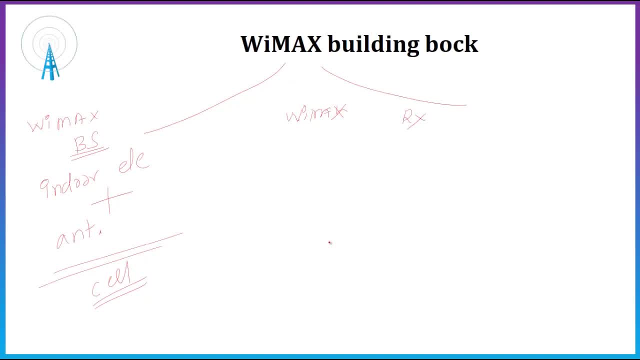 that the maximum radius of cell is like your 50 kilometer, okay so, or 30 miles in general. so we know we do understand better way in a kilometer, so i'll just write it down as a 50 kilometer. so practical consideration is actually. yeah, this is actually ideal value, but practically it is. 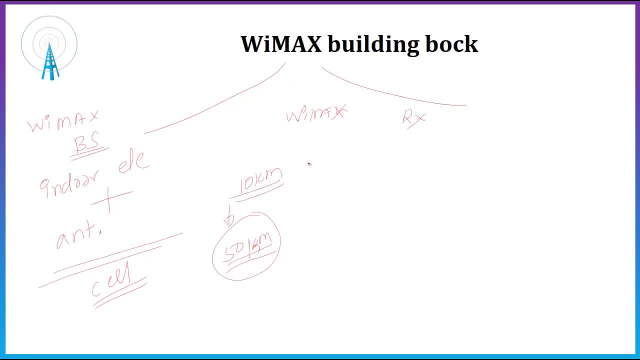 like 10 kilometers. okay, so y max receiver. so what is a y max receiver then? so y max receiver may have a separate antenna, or or we could say could stand alone in a box, or we could say like a computer-based hardware or anything would be there. so this is also referred as your customer premises. 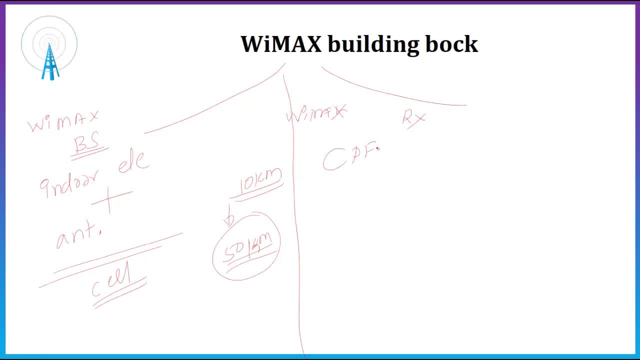 equipment. whatever we previously seen, CP, CP, what we are seeing. so this is actually customer premises equipment. okay, so why? max base station is similar to accessing wireless access point in a Wi-Fi network, but the coverage is greater. okay, so there's one more parameter I just forgot, which is called 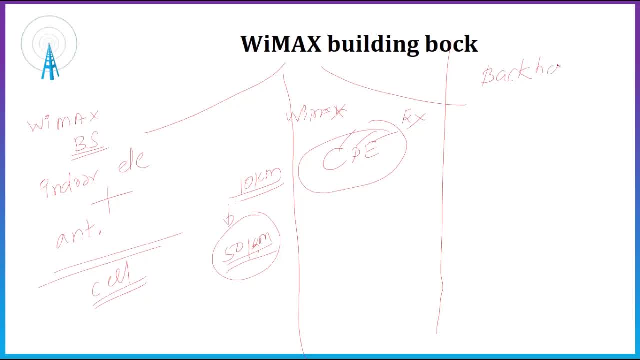 as your backhaul. so what is the backhaul? so a WiMAX tower station can connect directly to an internet using a high bandwidth wired connection- okay, like t3 line. it's an example. so it can also connect another WiMAX tower using your line-of-sight microwave link. so backhaul refers to both. refers to both, to the 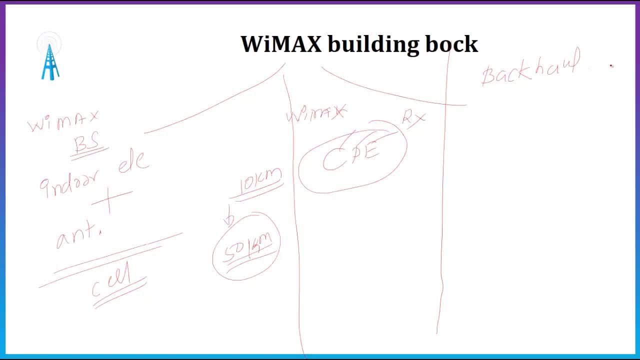 backhaul, so backhaul refers to both to the backhaul, so backhaul refers to both to the like connection from access point. like connection from access point, like connection from access point back to the base station. okay so, or we could back to the base station. okay so, or we could. 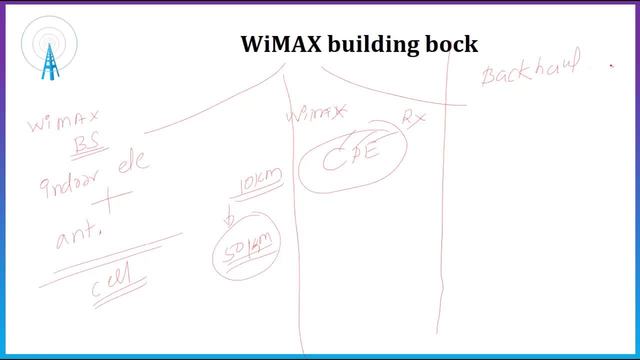 back to the base station. okay so, or we could say it can. it is possible to say it can. it is possible to say it can. it is possible to connect several base station to one another. connect several base station to one another. connect several base station to one another using your high-speed backhaul. 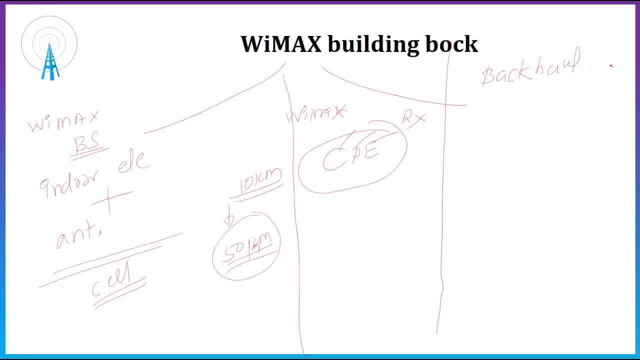 using your high-speed backhaul, using your high-speed backhaul microwave links. so this will also allow microwave links. so this will also allow microwave links. so this will also allow you for roaming by WiMAX subscriber from you, for roaming by WiMAX subscriber from you. for roaming by WiMAX subscriber from one base station coverage area, or we could. 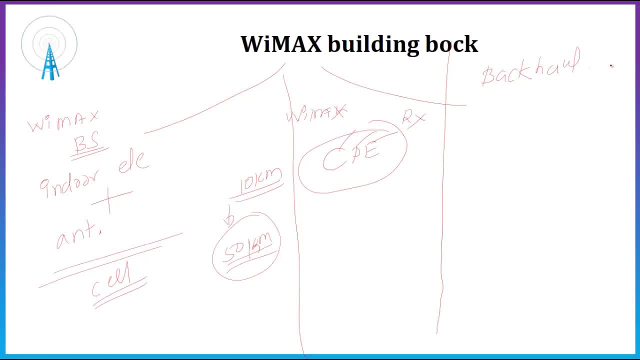 one base station coverage area, or we could one base station coverage area, or we could say: so, I think no, so this would say so, I think no, so this would say so, I think no, so this would actually allow you to roam by WiMAX, actually allow you to roam by WiMAX. 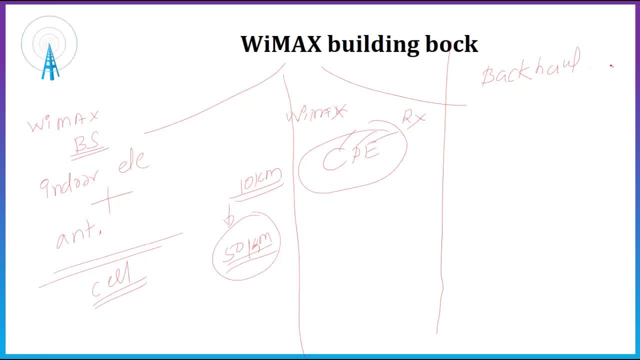 actually allow you to roam by WiMAX subscriber from one base station coverage subscriber from one base station coverage subscriber from one base station coverage area to another, and similar to roaming area to another, and similar to roaming area to another and similar to roaming enabled by your cell phones. okay, so this? 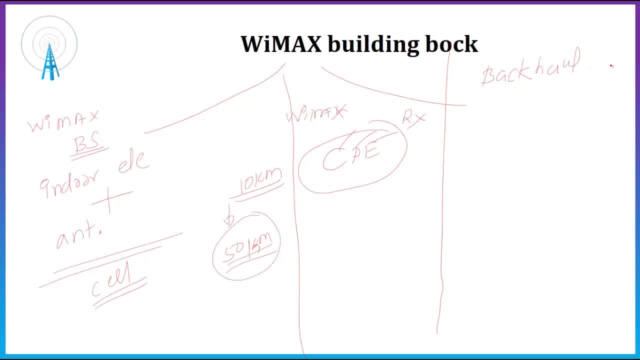 enabled by your cell phones. okay. so this enabled by your cell phones, okay. so this is all about your building blocks of is all about your building blocks of is all about your building blocks of your WiMAX- so these are actually main- your WiMAX, so these are actually main. 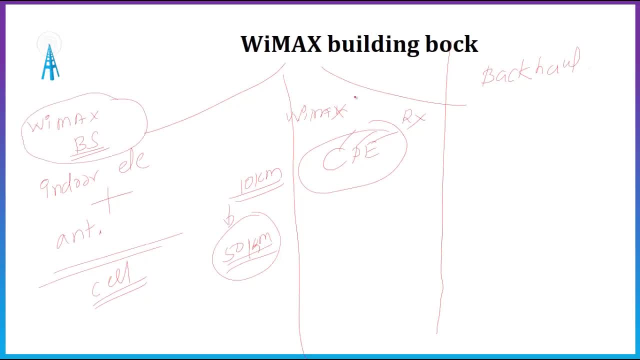 your WiMAX. so these are actually main building blocks. so WiMAX base station building blocks, so WiMAX base station building blocks. so WiMAX base station, WiMAX receiver and this is actually a WiMAX receiver and this is actually a WiMAX receiver and this is actually a supplementary thing which is called as a 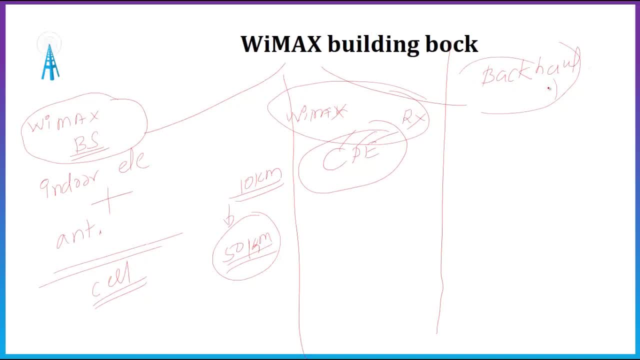 supplementary thing which is called as a supplementary thing, which is called as a back off. so WiMAX reference network back off. so WiMAX reference network back off. so WiMAX reference network model should be considered while we are model, should be considered while we are model should be considered while we are discussing. so this is your WiMAX. 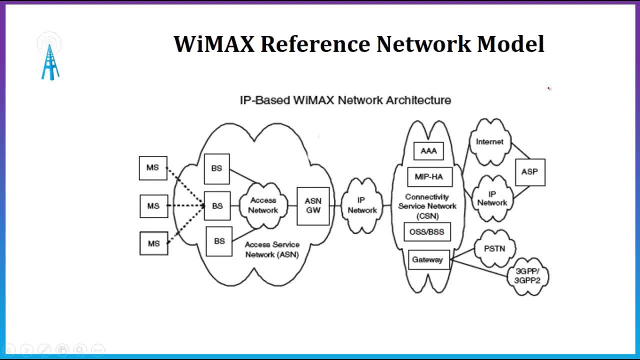 discussing. so this is your WiMAX discussing. so this is your WiMAX reference network model. so what is about reference network model? so what is about reference network model? so what is about this thing? so I triply 802 point 1, 6 e this thing. so I triply 802 point 1, 6 e. 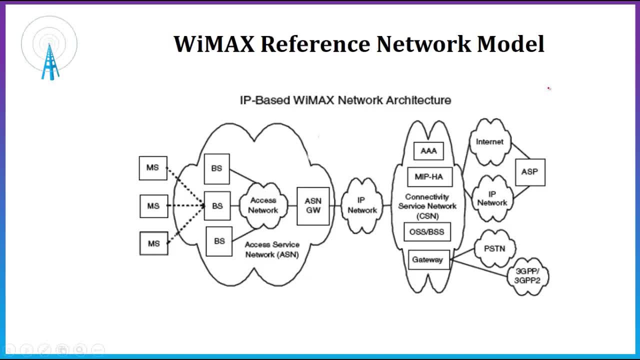 this thing. so I triply 802, point 1, 6 e, which was actually considered in 2005, which is actually a standard, which, which is actually a standard, which, which is actually a standard which provides a area interface for WiMAX, but provides a area interface for WiMAX, but. 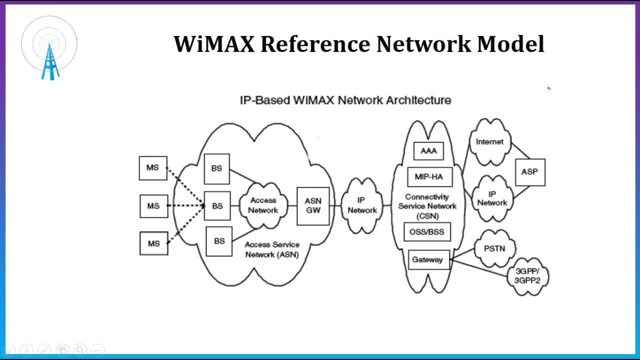 provides a area interface for WiMAX but does not define a full end-to-end WiMAX. does not define a full end-to-end WiMAX. does not define a full end-to-end WiMAX network. so the WiMAX forum network group network. so the WiMAX forum network group. 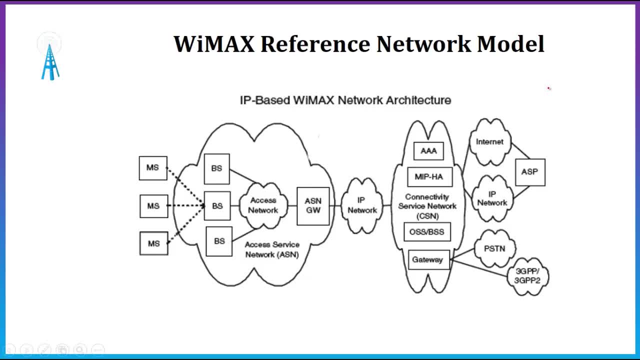 network. so the WiMAX forum network group, which is actually called as a NWG, it is which is actually called as a NWG, it is which is actually called as a NWG. it is responsible for developing end-to-end responsible for developing end-to-end, responsible for developing end-to-end network requirement architecture. okay, 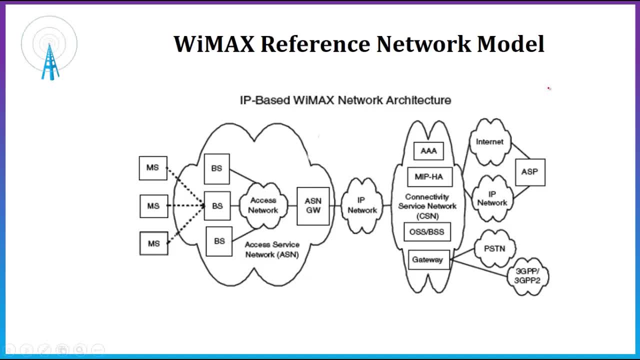 network requirement architecture: okay. network requirement architecture: okay. like network requirement is there, then like network requirement is there, then like network requirement is there, then they'll define. if there is any new, they'll define. if there is any new, they'll define. if there is any new requirement of architecture or a protocol. 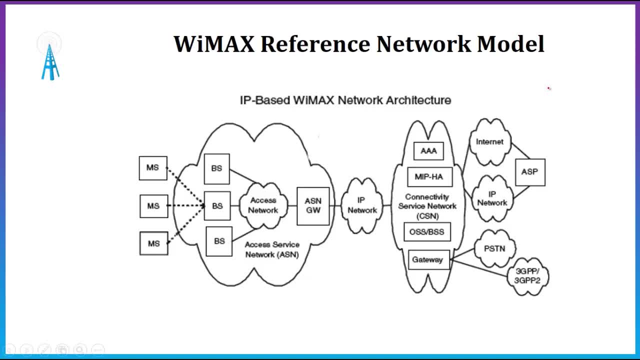 requirement of architecture or a protocol. requirement of architecture or a protocol for WiMAX. so using 802.1616 e-2005 for WiMAX. so using 802.1616 e-2005 for WiMAX. so using 802.1616 e-2005 as an area interface. so WiMAX NWG has. 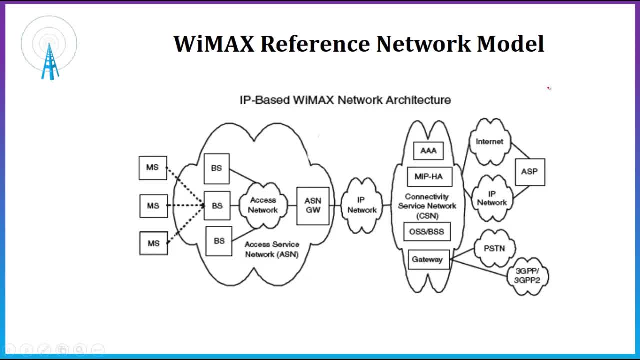 as an area interface. so WiMAX NWG has as an area interface. so WiMAX NWG has developed a network reference model to developed a network reference model, to developed a network reference model to serve architecture framework of WiMAX, serve architecture framework of WiMAX, serve architecture framework of WiMAX. deployment, the network reference model. 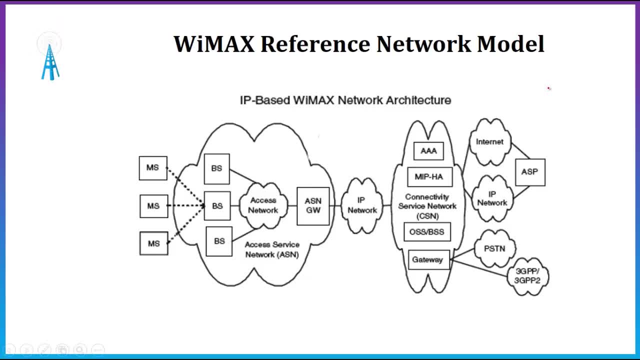 deployment: the network reference model. deployment: the network reference model: envision a unified network architecture. envision a unified network architecture. envision a unified network architecture for supporting fixed nomadic and your for supporting fixed nomadic and your for supporting fixed nomadic and your mobile deployments, and is based on your. 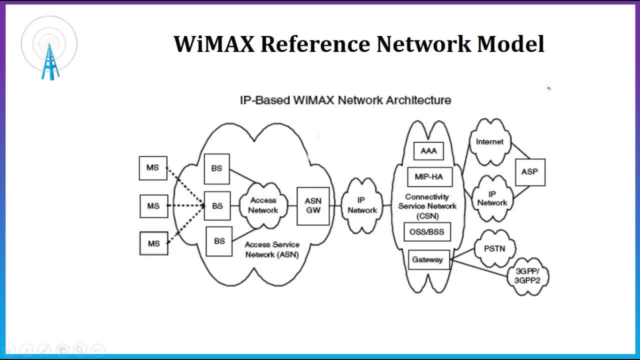 mobile deployments and is based on your mobile deployments and is based on your IP service model. so, whatever this thing- IP service model, so whatever this thing- IP service model, so whatever this thing is, this is actually what we could see is- is this is actually what we could see is. 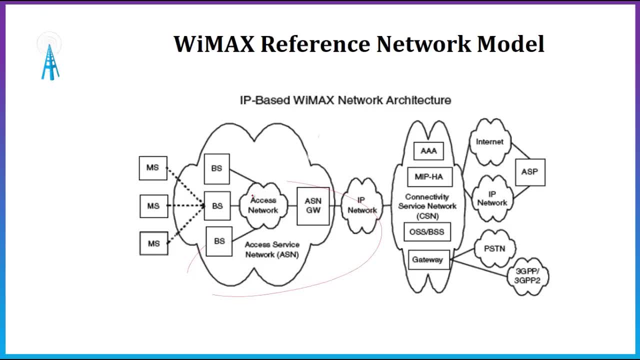 is. this is actually what we could see is a simplified version or simplified. a simplified version or simplified. a simplified version or simplified illustration of your IP based WiMAX. illustration of your IP based WiMAX. illustration of your IP based WiMAX network architecture. so this is the 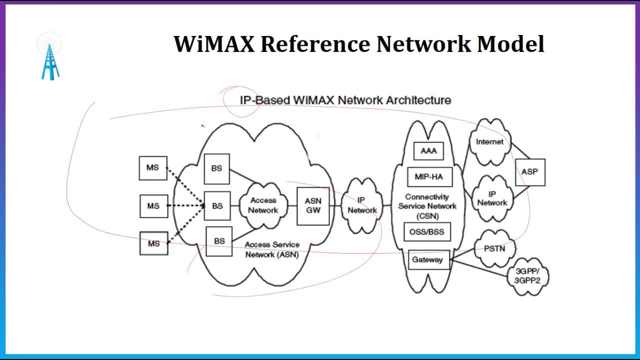 network architecture. so this is the network architecture. so this is the entire architecture which is actually based, entire architecture which is actually based, entire architecture which is actually based on your IP. okay, so here we could on your IP. okay, so here we could on your IP. okay, so here we could divide this thing into three parts. 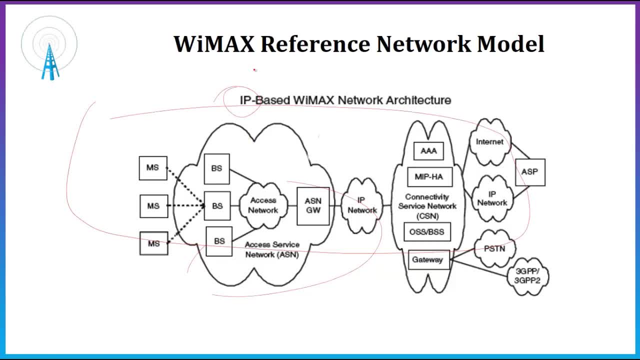 divide this thing into three parts. divide this thing into three parts logically, so first one is your mobile. logically, so first one is your mobile. logically, so first one is your mobile session. so this could be your first part session, so this could be your first part session. so this could be your first part, and the second would be access services. 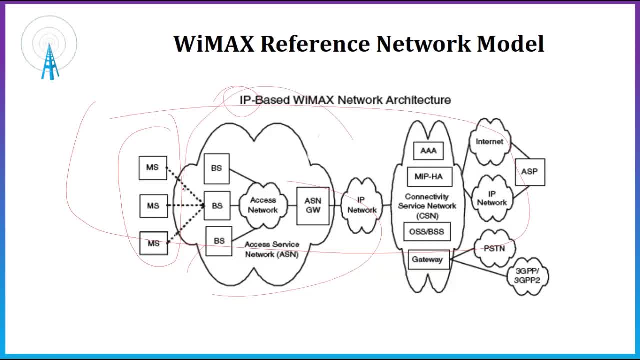 and the second would be access services and the second would be access services or ASN in general. so this entire part, or ASN in general, so this entire part, or ASN in general. so this entire part will be like ASN and the third one will will be like ASN and the third one will. 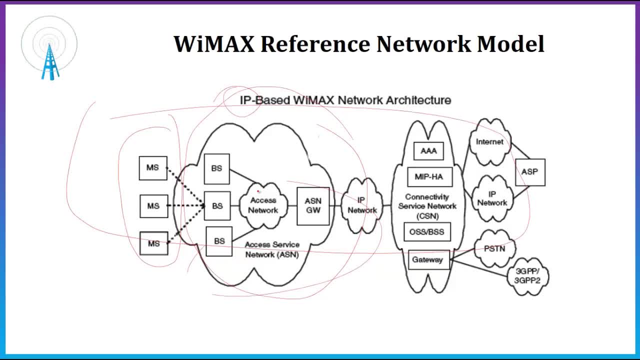 will be like ASN. and the third one will be connectivity service network. okay, so be connectivity service network. okay, so be connectivity service network. okay, so whatever this CSN's are there, so this is whatever this CSN's are there, so this is whatever this CSN's are there, so this is considered as your CSN, or just consider: 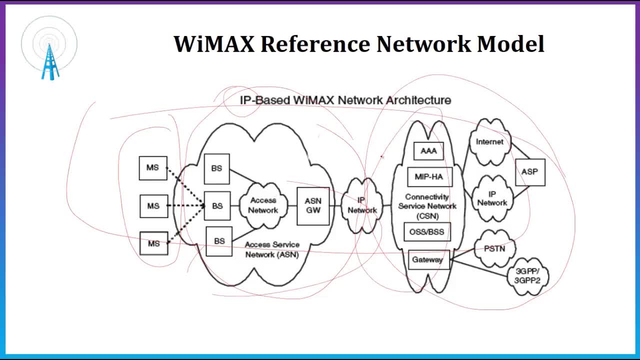 considered as your CSN, or just consider, considered as your CSN, or just consider this thing, this cloud, you consider that this thing, this cloud, you consider that this thing, this cloud, you consider that is actually your CSN, so now you are is actually your CSN, so now you are. 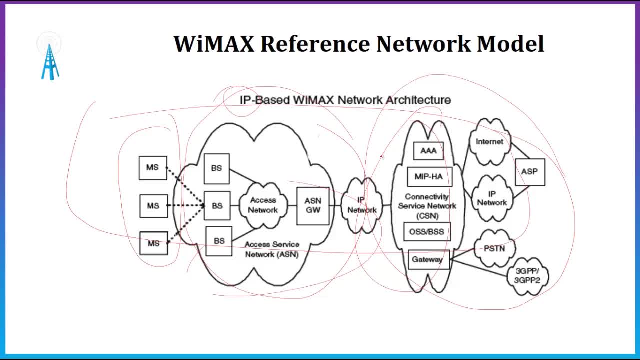 is actually your CSN. so now you are divided into in three different parts. so divided into in three different parts. so divided into in three different parts. so MS or mobile stations. mobile stations are MS or mobile stations. mobile stations are MS or mobile stations. mobile stations are used by an end user to access a network. 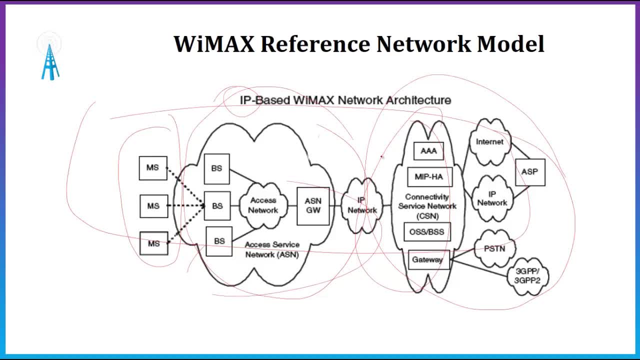 used by an end user to access a network. used by an end user to access a network. okay that you know it better. so the what? okay that you know it better. so the what? okay that you know it better. so the what is ASN? so access service network, which. 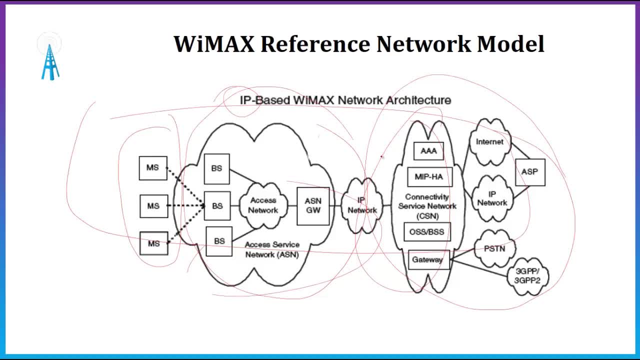 is ASN, so access service network, which is ASN, so access service network, which comprise one or more base station, and one comprise one or more base station, and one comprise one or more base station and one or more ASN gateways that form a radio, or more ASN gateways that form a radio. 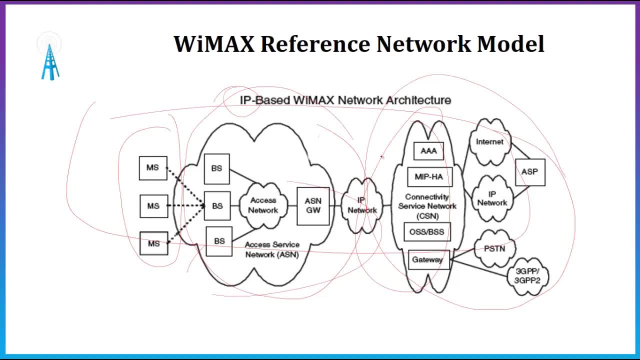 or more ASN gateways that form a radio access network at a edge, then your CSN access network at a edge, then your CSN access network at a edge, then your CSN, which provides your IP connectivity, and which provides your IP connectivity, and which provides your IP connectivity and IP core network function. okay, so in 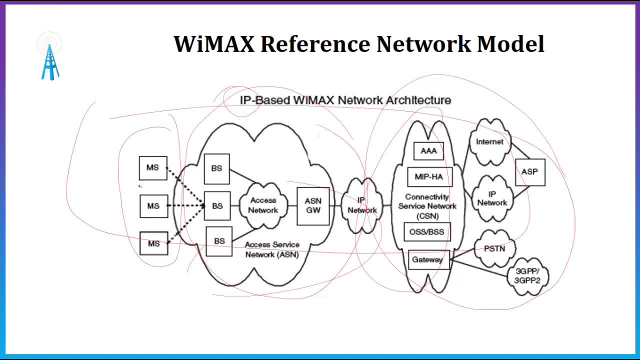 IP core network function okay. so in IP core network function okay. so in detail, to say like your this BS, MS, BS. detail. to say like your this BS, MS, BS. detail. to say, like your this BS, MS, BS, your ASN, CSN, what they do. so the network, 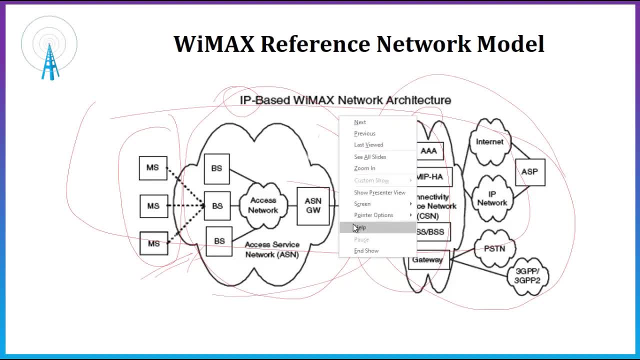 your ASN CSN. what they do so. the network- your ASN CSN. what they do so. the network: reference model developed by WiMAX group. reference model developed by WiMAX group. reference model developed by WiMAX group. defines a number of functional entities. defines a number of functional entities. 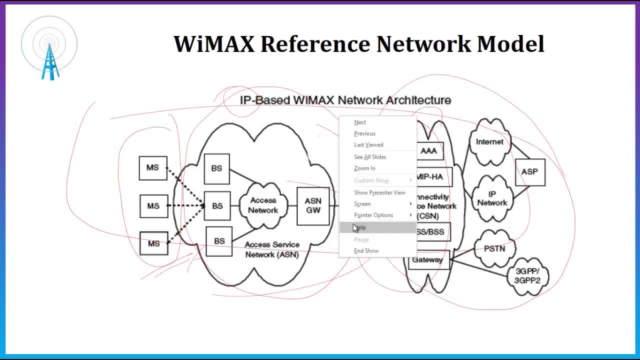 defines a number of functional entities or the interfaces to. so what are those? or the interfaces to? so what are those? or the interfaces to? so what are those? so like here we could see there is a. so like here we could see there is a. so like here we could see there is a. where is my marker? so here it is your BS. 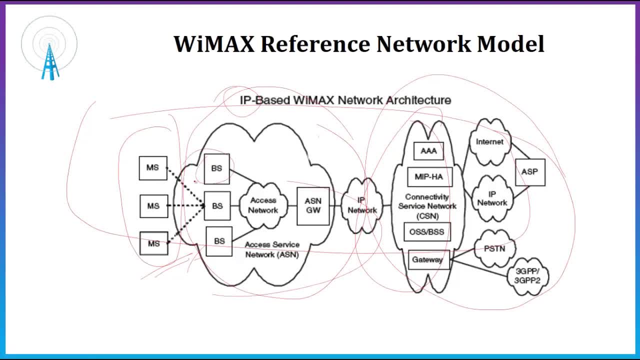 where is my marker? so here it is your BS. where is my marker? so here it is your BS. just a second. so this is your BS. so this, just a second. so this is your BS. so this, just a second. so this is your BS. so this is actually your another entity. so what? 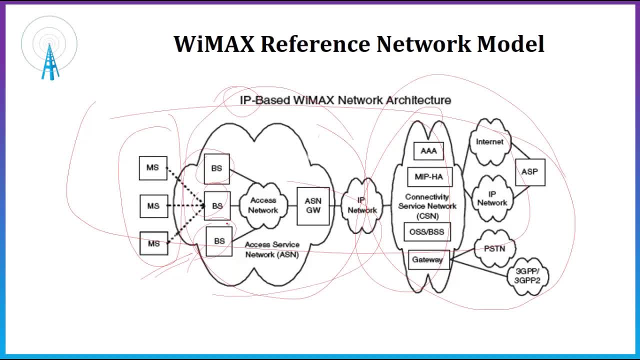 is actually your another entity. so what is actually your another entity? so what is this BS? so BS is actually responsible? is this BS so BS is actually responsible? is this BS so BS is actually responsible for providing your air interface to MS, for providing your air interface to MS? 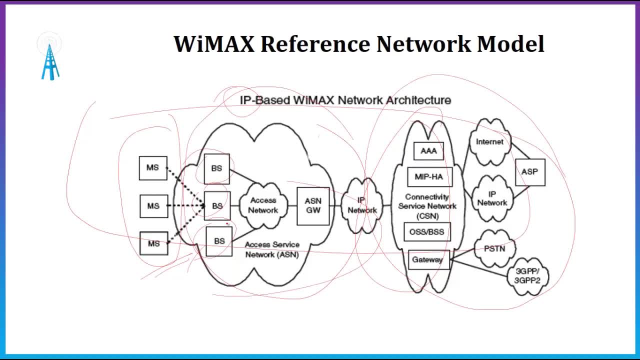 for providing your air interface to MS. so additional function that may be a part. so additional function that may be a part. so additional function that may be a part of BS, of a micro mobility management of BS, of a micro mobility management of BS, of a micro mobility management function such as like a handoff. 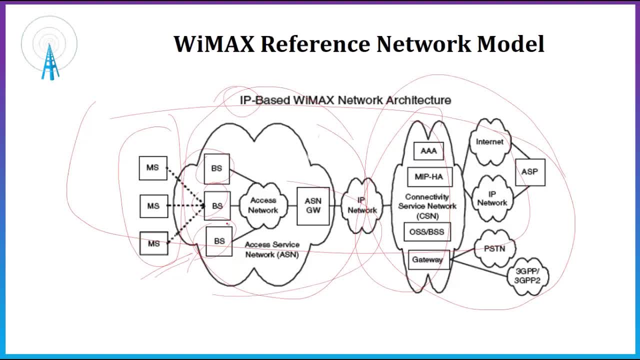 function, such as like a handoff function, such as like a handoff triggering then tunnel establishment, radio triggering then tunnel establishment. radio triggering then tunnel establishment, radio resource management: quality of service resource management. quality of service resource management. quality of service policy enforcement. traffic policy enforcement. traffic classification. 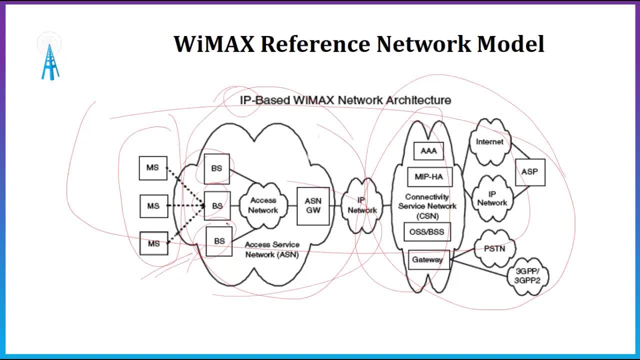 policy enforcement traffic classification- DHCP. so the key management and session classification DHCP. so the key management and session classification DHCP. so the key management and session management function could be management function could be management function could be done by your BS. so again there is the simply done by your BS. so again there is the simply. 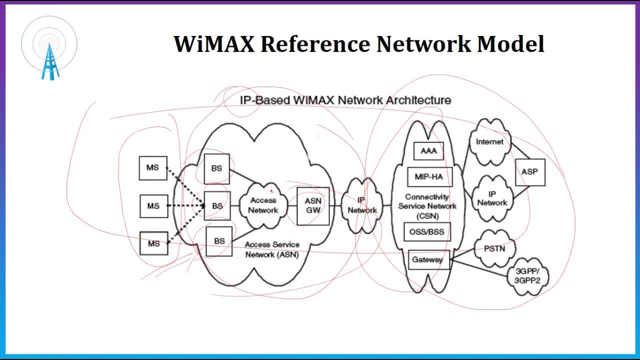 done by your BS. so again there is the simply like ASN GW is there. so what is like ASN GW is there. so what is like ASN GW is there. so what is this ASN GW? so it is actually your access, this ASN GW? so it is actually your access. 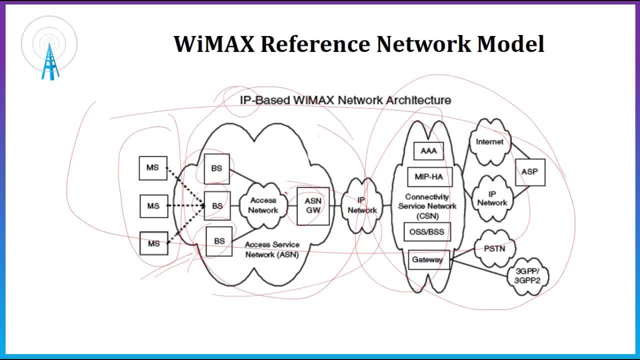 this ASN GW. so it is actually your access service network gateway. so obviously you service network gateway. so obviously you service network gateway. so obviously you know what is the function of gate. so know what is the function of gate. so know what is the function of gate. so again there is a CSN I think we have. 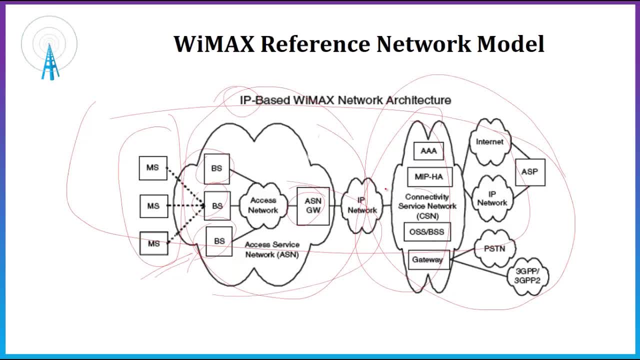 again there is a CSN. I think we have again there is a CSN. I think we have already discussed. what is CSN so what is already discussed. what is CSN so what is already discussed. what is CSN so what is CSN? to CS in CSN will provides like: 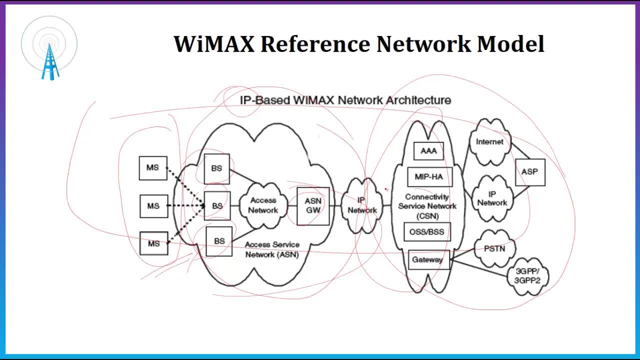 CSN to CSN in CSN will provides like CSN to CSN. in CSN will provides like connectivity to an internet or other connectivity to an internet or other connectivity to an internet or other public network or internet or ESPs, or public network or internet or ESPs, or. 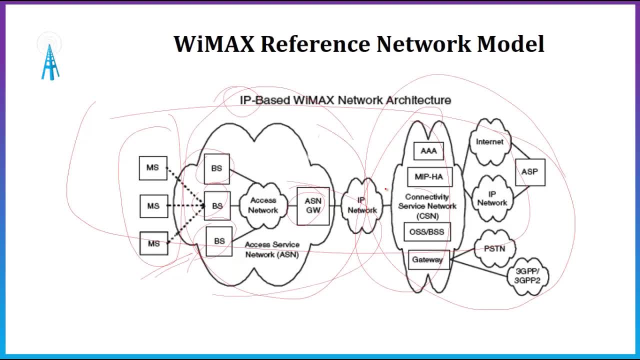 public network or internet, or ESPs, or public network or corporate network. so public network or corporate network? so public network or corporate network. so actually CSN is owned by your NSP and actually CSN is owned by your NSP and actually CSN is owned by your NSP and includes, like your, these AAA servers. so 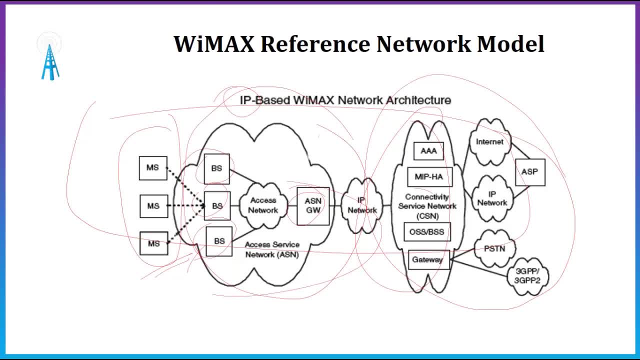 includes, like your, these AAA servers. so includes, like your, these AAA servers so that supports actually your, that supports actually your, that supports actually your authentication devices or user specific authentication devices or user specific authentication devices or user specific services. the CSN will also provide you services. the CSN will also provide you. 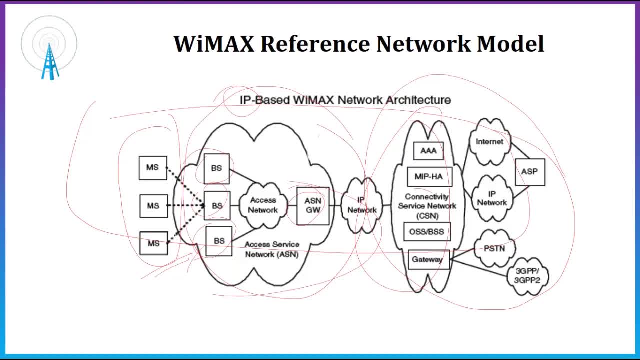 services. the CSN will also provide you what we could say the user policy, what we could say the user policy, what we could say the user policy- management or quality of service, or management, or quality of service, or management or quality of service or security. okay, so WiMAX architecture. 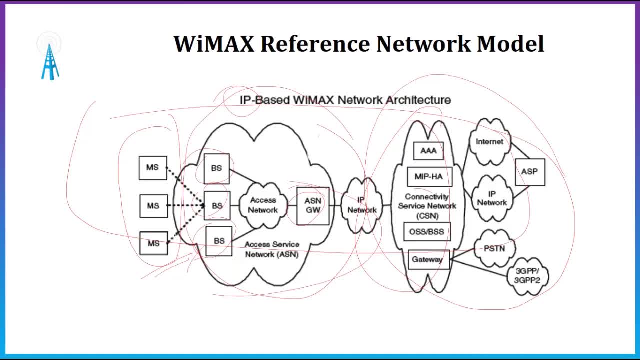 security. okay so WiMAX architecture security. okay, so WiMAX architecture framework allows you a flexible framework, allows you a flexible framework, allows you a flexible decomposition and or a combination of decomposition and or a combination of decomposition and or a combination of functional entities. while building your functional entities, while building your 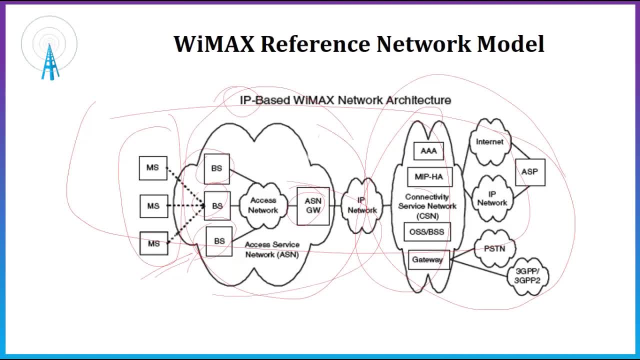 functional entities while building your physical entities. for example, ASN may be physical entities. for example, ASN may be physical entities. for example, ASN may be more base station trans receiver, we more base station trans receiver, we more base station trans receiver. we could say combinedly and base station. 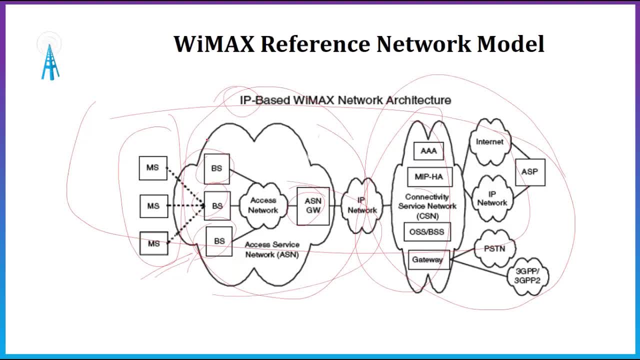 could say combinedly, and base station could say combinedly, and base station controllers like BSC, then again serving controllers like BSC, then again serving controllers like BSC, then again serving GPRA support node as GSN, so these kind GPRA support node as GSN, so these kind. 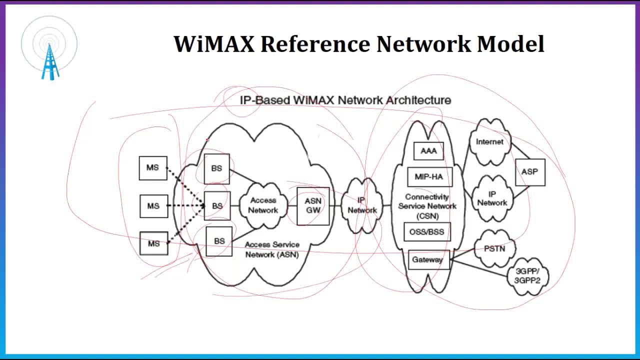 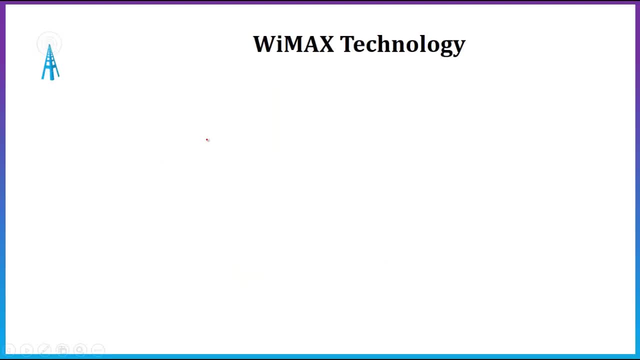 GPRA support node as GSN. so these kind of entities are there. so now parameter of entities are there. so now parameter of entities are there. so now parameter comes is WiMAX technology. so in WiMAX comes is WiMAX technology. so in WiMAX comes is WiMAX technology. so in WiMAX technology it is actually based on your. 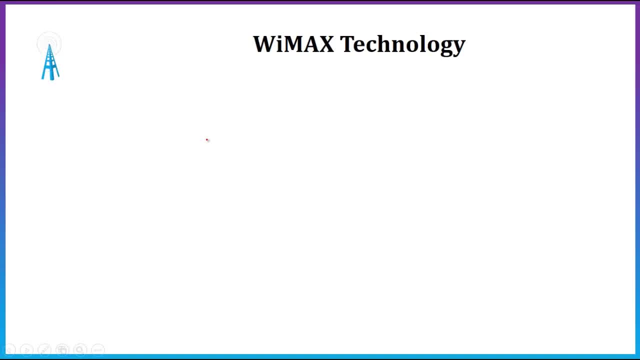 technology. it is actually based on your technology. it is actually based on your IEEE 802.16 specification. so, IEEE 802.16 specification, so to enable a delivery of your last-mile, to enable a delivery of your last-mile, to enable a delivery of your last-mile wireless broadband access as an 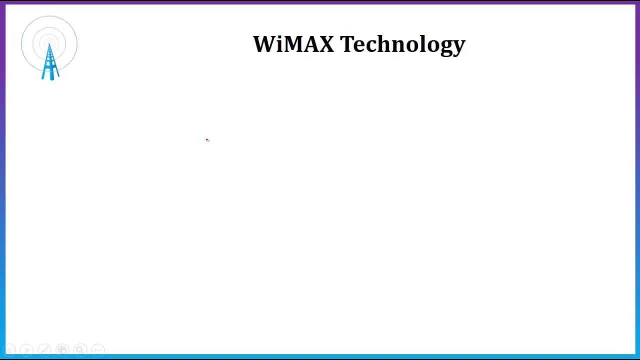 wireless broadband access as an wireless broadband access, as an alternative to your cable or DSL. so the alternative to your cable or DSL, so the alternative to your cable or DSL. so the design of WiMAX network is actually design of WiMAX network is actually design of WiMAX network is actually based on following major principles: so: 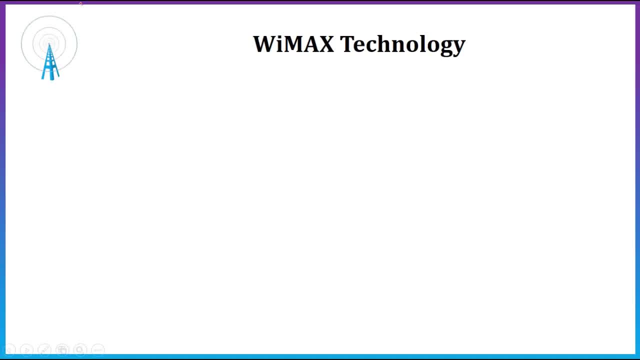 based on following major principles. so, based on following major principles. so what are the following principles that? what are the following principles that? what are the following principles that we consider so WiMAX technology follows? we consider so WiMAX technology follows. we consider so WiMAX technology follows like spectrum. second one is like your. 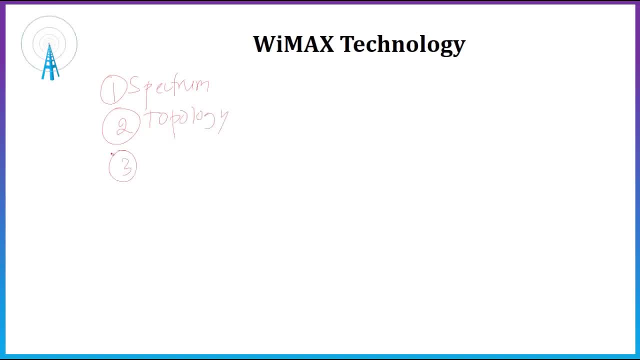 like spectrum. second one is like your like spectrum. second one is like your topology: topology. topology like internet, no interworking. then I think like internet, no interworking. then I think like internet, no interworking. then I think there is IP connectivity also there. there is IP connectivity also there. 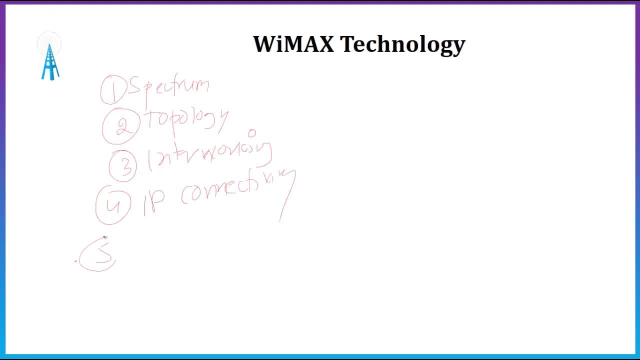 there is IP connectivity also there and there is a sorry: this is not mobile. and there is a sorry: this is not mobile. and there is a sorry: this is not mobile. this is actually should be mobility. this is actually should be mobility. this is actually should be mobility management. okay. 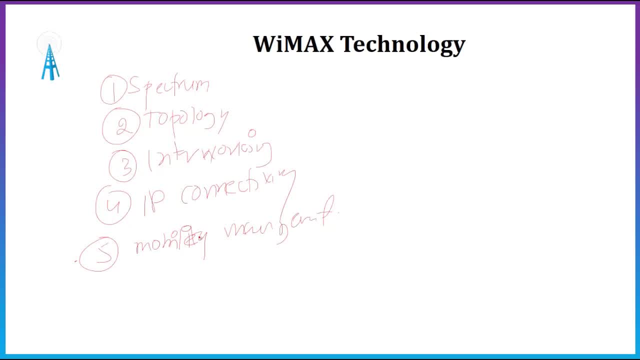 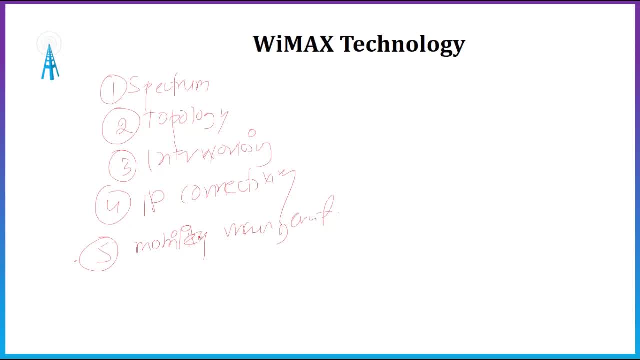 networks are designed so spectrum is. networks are designed so spectrum is. actually it is capable of deploying both. actually it is capable of deploying both. actually it is capable of deploying both: license and license. spectrum topology is license and license. spectrum topology is license and license. spectrum topology is actually like it provides a ran. 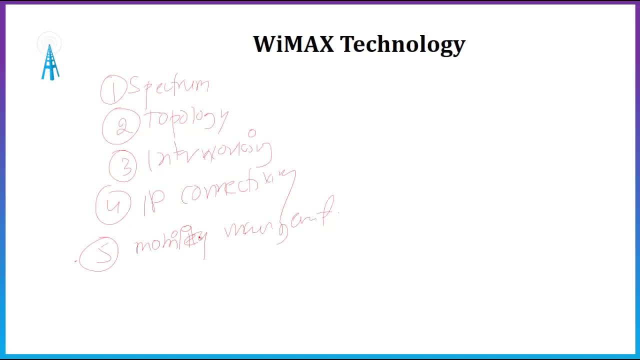 actually like it provides a ran. actually like it provides a ran. topologies like radio access network. topologies like radio access network. topologies like radio access network. topologies. internet working like 3gbp topologies. internet working like 3gbp topologies. internet working like 3gbp and 3gbp. to networks are being added IP. 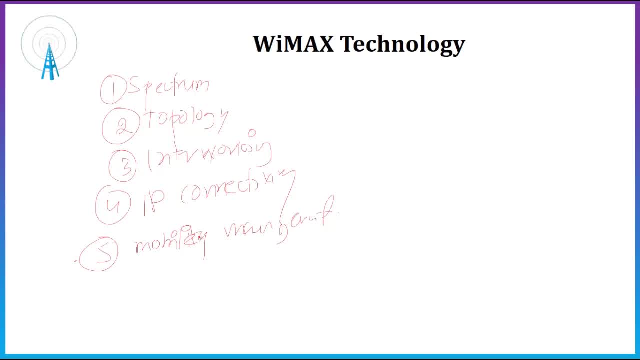 and 3gbp to networks are being added. IP and 3gbp to networks are being added. IP connectivity means like to support a mix. connectivity means like to support a mix. connectivity means like to support a mix of IP, v4 and v6, so this is actually IP. 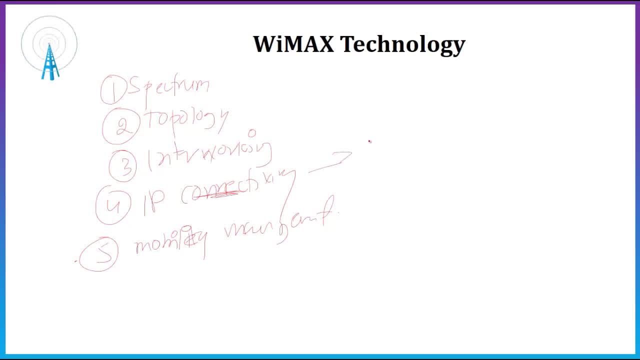 of IP v4 and v6, so this is actually IP of IP v4 and v6, so this is actually IP connectivity. so it's a combination of IP connectivity. so it's a combination of IP connectivity. so it's a combination of IP v4 and v6. so mobility management is like. 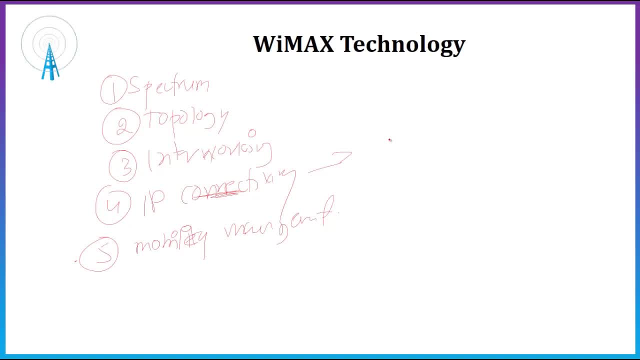 v4 and v6. so mobility management is like v4 and v6. so mobility management is like possibility to extend a fixed access to possibility to extend a fixed access to possibility to extend a fixed access to mobility and broadband multimedia mobility and broadband multimedia mobility and broadband multimedia service delivery. okay, so there are. 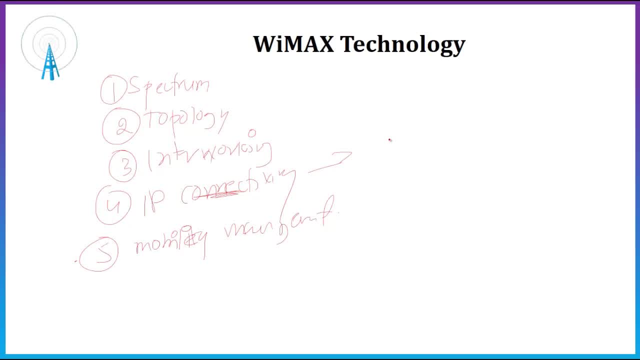 service delivery. okay, so there are service delivery, okay, so there are actually many parameters that we could actually many parameters that we could actually many parameters that we could inferred your what we could say WiMAX inferred your what we could say WiMAX inferred your what we could say WiMAX physical, in which there is actually 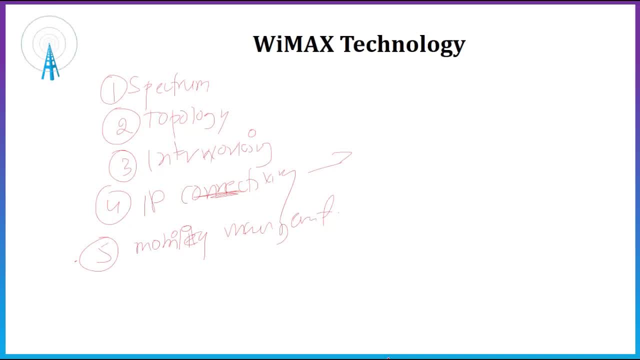 physical in which there is actually physical, in which there is actually adaptive modulation and coding in WiMAX: adaptive modulation and coding in WiMAX, adaptive modulation and coding in WiMAX. so again there comes with like some of so again there comes with like some of so again there comes with like some of the downlink or uplink related various. 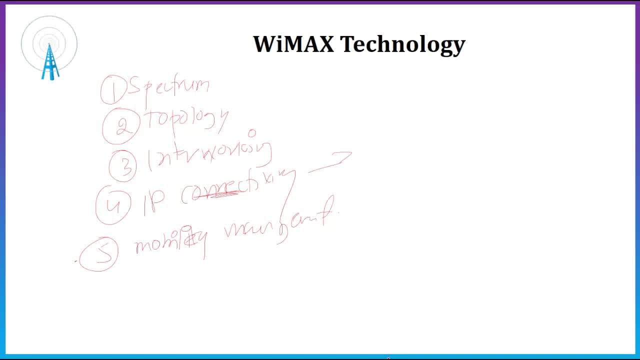 the downlink or uplink related various. the downlink or uplink related various modulation coding schemes for WiMAX. so modulation coding schemes for WiMAX, so modulation coding schemes for WiMAX. so like mean downlink it may be possible. like mean downlink it may be possible. 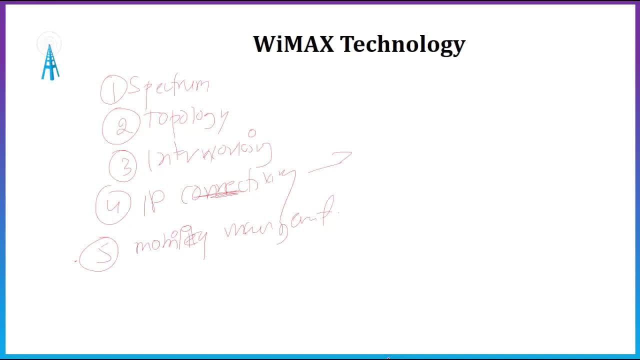 like mean downlink. it may be possible that both can have a same modulation, that both can have a same modulation, that both can have a same modulation technique. so downlink and uplink technique, so downlink and uplink technique. so downlink and uplink modulation techniques could be like a BPS. 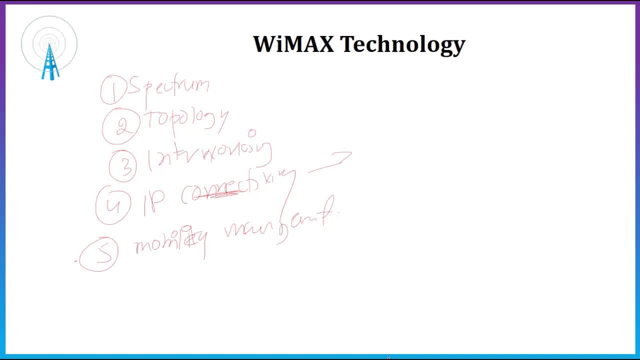 modulation techniques could be like a BPS. modulation techniques could be like a BPS. he will be there. QPS will be there. 16. he will be there. QPS will be there. 16, he will be there. QPS will be there. 16 comm will be there. 64 comm will be there. 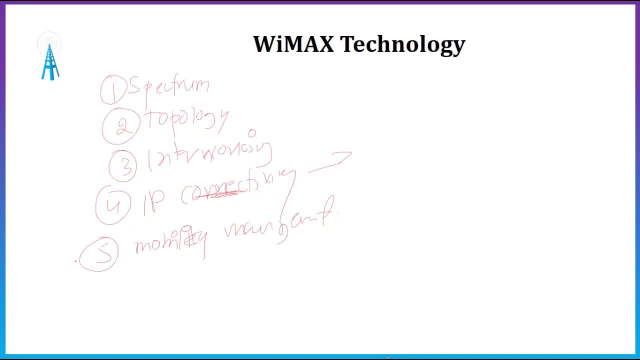 comm will be there, 64 comm will be there. comm will be there, 64 comm will be there. then like o FDM for a physical channel, then like o FDM for a physical channel. then like o FDM for a physical channel will be there. then there is a coding. 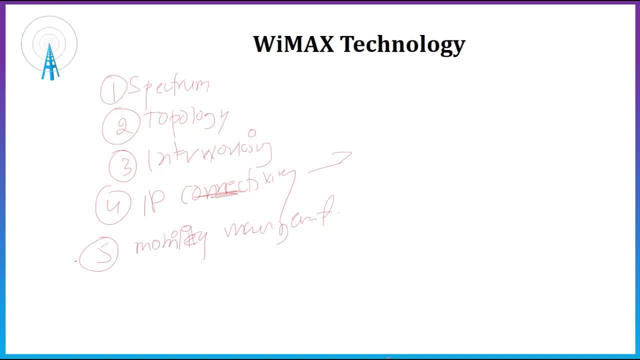 will be there, then there is a coding will be there, then there is a coding. techniques are like half rate or quarter. techniques are like half rate or quarter. techniques are like half rate or quarter rate, or we could say 2 by 3 or 5 by 6. 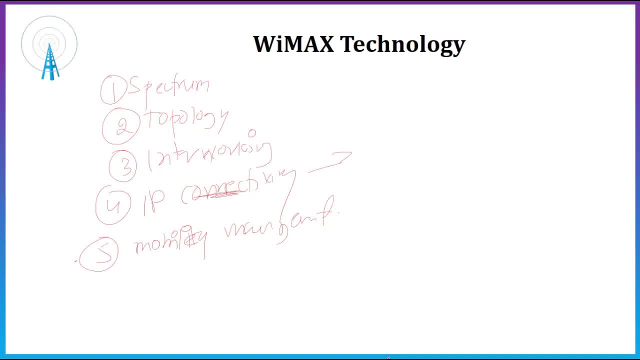 rate, or we could say 2 by 3 or 5 by 6 rate, or we could say 2 by 3 or 5 by 6. these are actually convalescent codes. these are actually convalescent codes. these are actually convalescent codes. are there which are actually a mandatory? 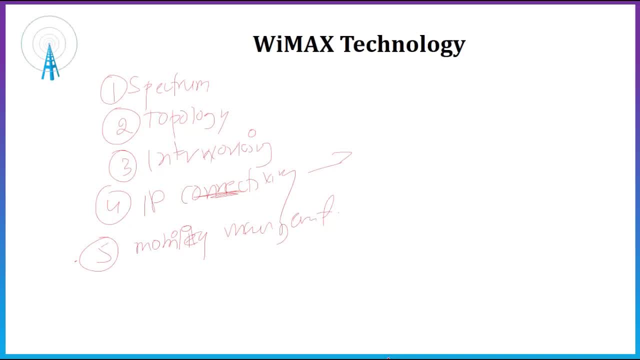 are there which are actually a mandatory? are there which are actually a mandatory? thing which is same for your uplink and thing which is same for your uplink and thing which is same for your uplink and whereas in coding for your downlink and whereas in coding for your downlink, and. 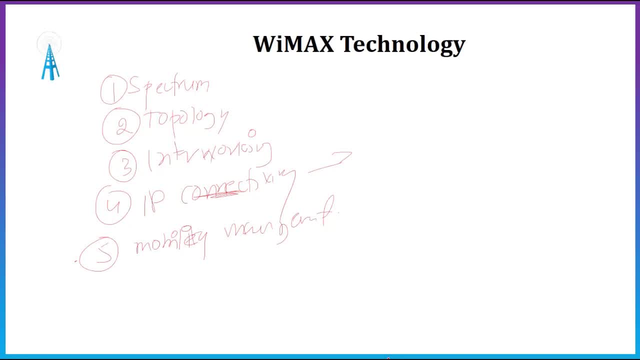 whereas in coding for your downlink and we could say for uplink, there are, we could say for uplink, there are, we could say for uplink there are actually optional codes like half 2 by 3 actually optional codes like half 2 by 3. 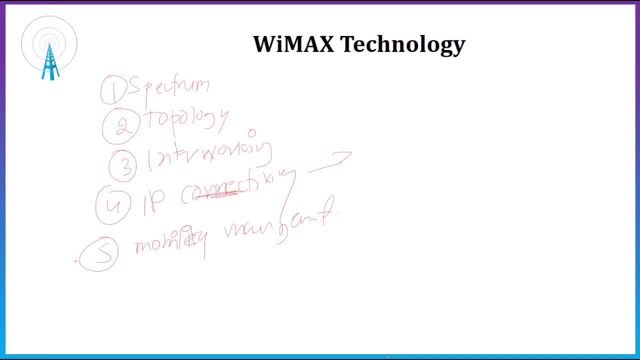 actually optional codes like half 2 by 3, 3 by 4, 5 by 6, convolutional codes are 3 by 4, 5 by 6, convolutional codes are 3 by 4, 5 by 6. convolutional codes are there or convolutional turbo codes are. 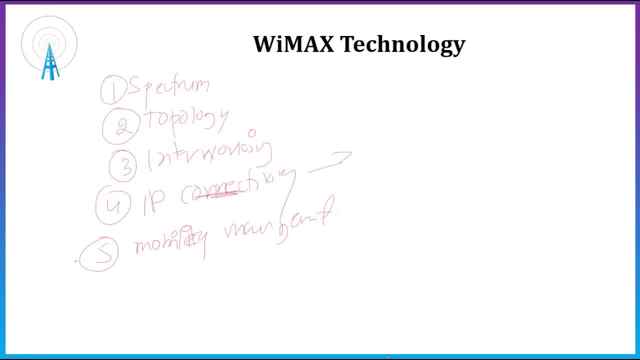 there. or convolutional turbo codes are there, or convolutional turbo codes are there. even repetition codes are run at there. even repetition codes are run at there. even repetition codes are run at half speed, or something like that is half speed or something like that is half speed, or something like that is there. so which will create actually much. 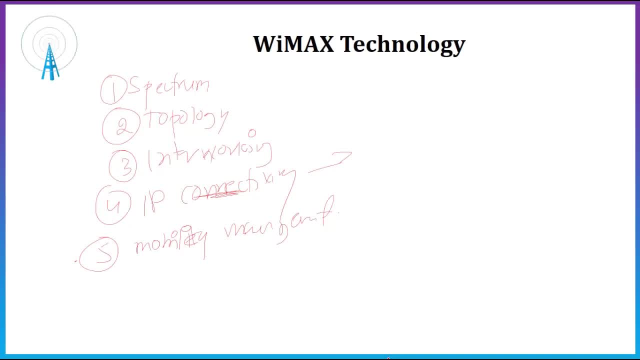 there, so which will create actually much there, so which will create actually much confusion. so I am NOT discussing those confusion. so I am NOT discussing those confusion. so I am NOT discussing those part. so the next one is your WiMAX part. so the next one is your WiMAX. 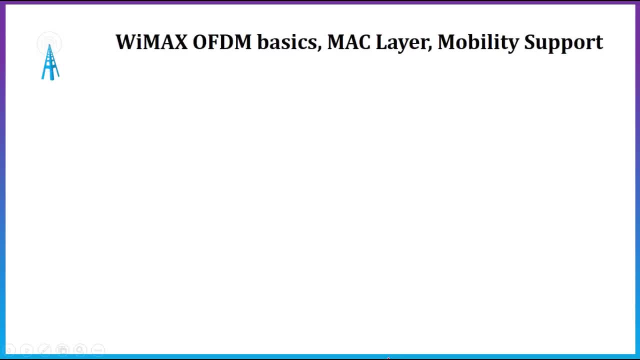 part. so the next one is your WiMAX physical layer. so I think I already physical layer, so I think I already physical layer. so I think I already discussed this thing, discussed this thing, discussed this thing: OVM basics- okay fine, so OVM actually. OVM basics- okay fine, so OVM actually. 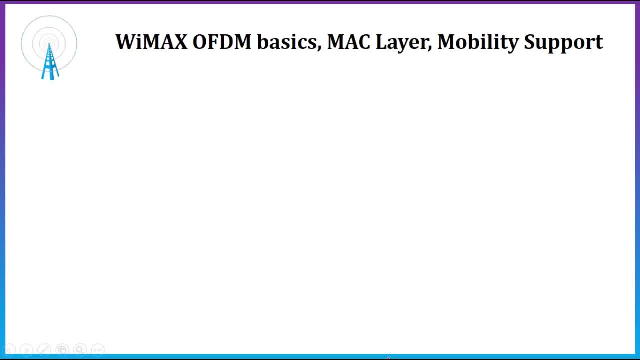 OVM basics. okay, fine, so OVM actually belongs to a family of transmission, belongs to a family of transmission, belongs to a family of transmission schemes, called as your multi carrier schemes, called as your multi carrier schemes, called as your multi carrier modulation. okay, so, which is actually? 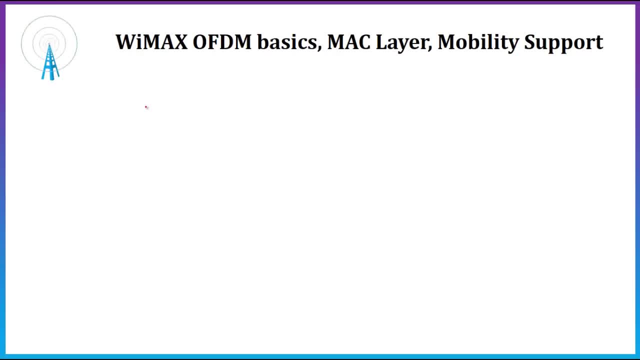 modulation. okay, so which is actually modulation? okay, so which is actually based on your idea of dividing given. based on your idea of dividing given, based on your idea of dividing given bitrate or bitrate data stream into bitrate or bitrate data stream into bitrate or bitrate data stream into several parallel lower bit streams, and? 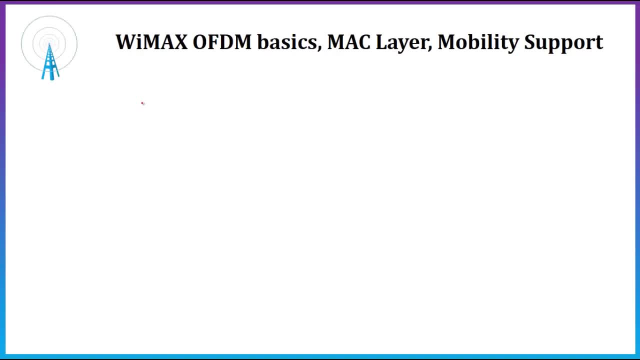 several parallel lower bit streams and several parallel lower bit streams and modulating each stream to a separate. modulating each stream to a separate. modulating each stream to a separate carrier. it is often considered as your carrier. it is often considered as your carrier, it is often considered as your tones, or we could say, the better word is: 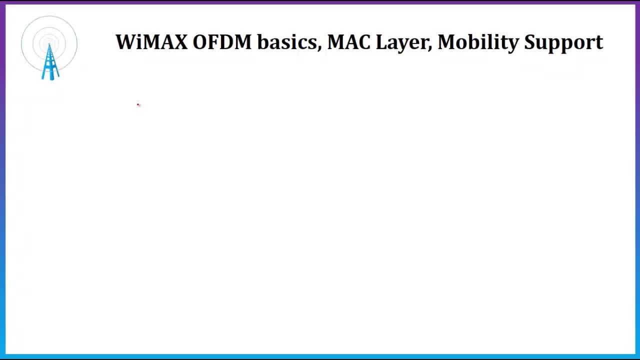 tones, or we could say the better word is tones, or we could say the better word is sub carrier, so multicolor carrier, sub carrier, so multicolor carrier, sub carrier, so multicolor carrier. modulation is actually a scheme. which modulation is actually a scheme? which modulation is actually a scheme which eliminates or minimize the inter symbol. 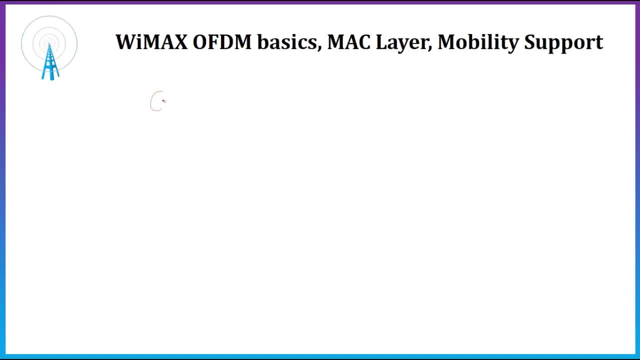 eliminates or minimize the inter symbol. eliminates or minimize the inter symbol: interference. so you already know that interference. so you already know that interference. so you already know that. OFDM: what is OFDM? orthogonal frequency, OFDM: what is OFDM? orthogonal frequency? OFDM: what is OFDM? orthogonal frequency? division, multiplexing. okay, so this is in. 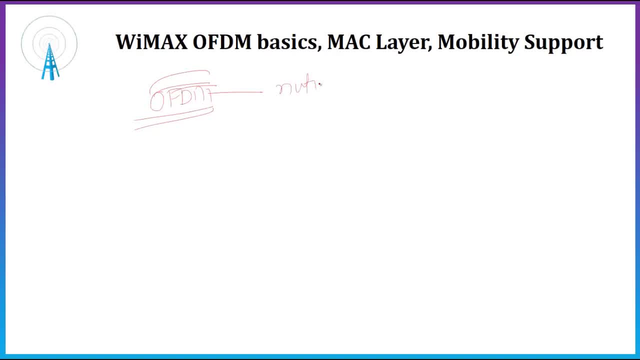 division multiplexing: okay. so this is in division multiplexing, okay. so this is in general. if you need to just consider general, if you need to just consider general, if you need to just consider some of the key parameter, so this is some of the key parameter. so this is. 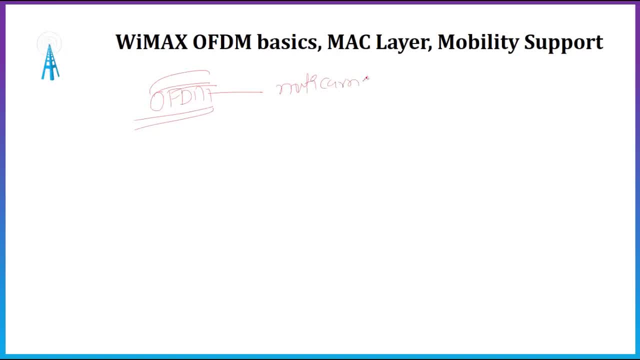 some of the key parameter. so this is actually multi carrier modulation. so what, actually multi carrier modulation? so what, actually multi carrier modulation? so what it will do? it will decrease your ISI. it will do. it will decrease your ISI. it will do. it will decrease your ISI. okay, and we could see it will make your 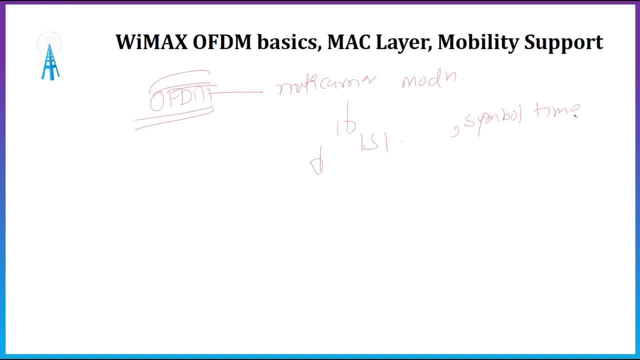 okay, and we could see it will make your okay, and we could see it will make your symbol time larger. okay, it has to be symbol time larger. okay, it has to be symbol time larger. okay, it has to be larger, larger, larger so that there will be channel induced delay will be like typically. 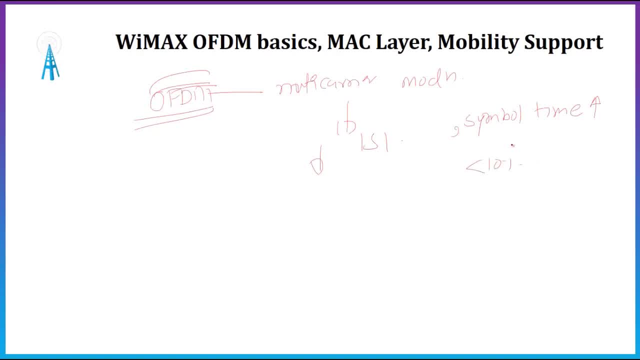 so that there will be channel induced delay will be like typically, so that there will be channel induced delay will be like typically, less than 10% would be there. so it, less than 10% would be there. so it less than 10% would be there, so it will be beneficial. so, in general saying: 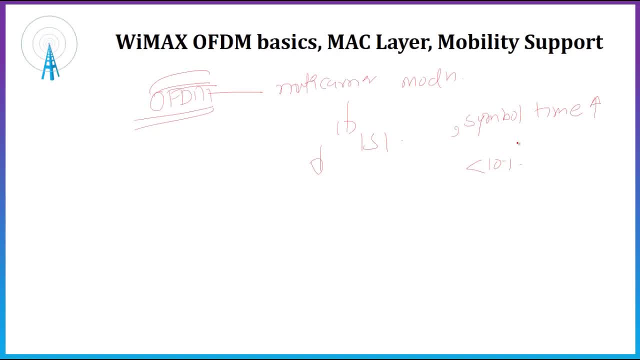 will be beneficial. so, in general saying will be beneficial. so, in general, saying OFDM is actually a spectrally efficient OFDM is actually a spectrally efficient OFDM is actually a spectrally efficient version of your multi carrier modulation version of your multi carrier modulation. 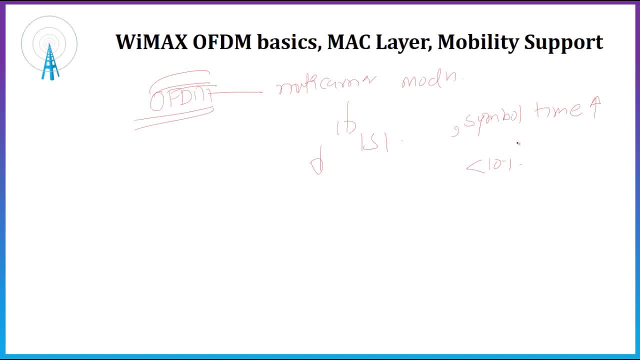 version of your multi carrier modulation where the sub carriers are selected, such where the sub carriers are selected, such where the sub carriers are selected such that they all are orthogonal to one, that they all are orthogonal to one, that they all are orthogonal to one another or a symbol duration thereby. 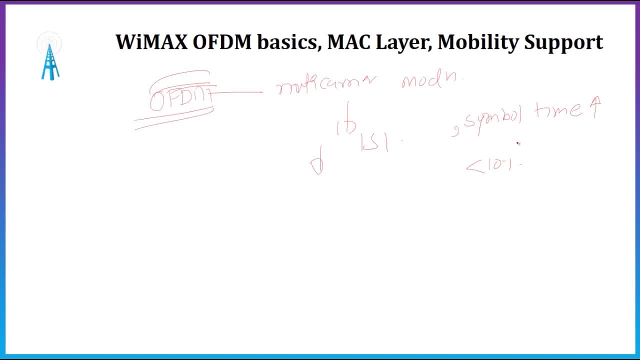 another or a symbol duration. thereby another or a symbol duration, thereby avoiding your need to have non, avoiding your need to have non, avoiding your need to have non overlapping subcarrier channels to overlapping subcarrier channels, to overlapping subcarrier channels, to eliminate your inter carrier, eliminate your inter carrier. 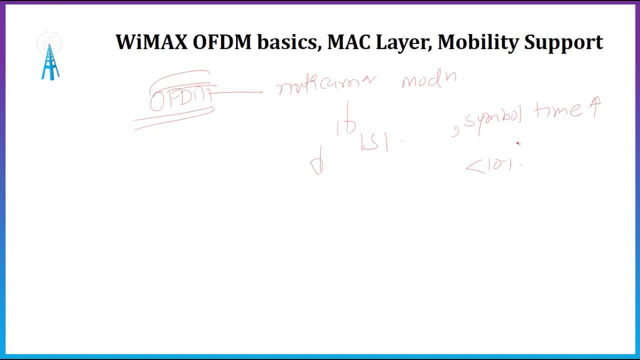 eliminate your inter carrier interference. so, in order to completely interference, so, in order to completely interference, so in order to completely eliminate. ISI guard intervals are eliminate, ISI guard intervals are eliminate. ISI guard intervals are actually used between your OFDM symbols, actually used between your OFDM symbols. 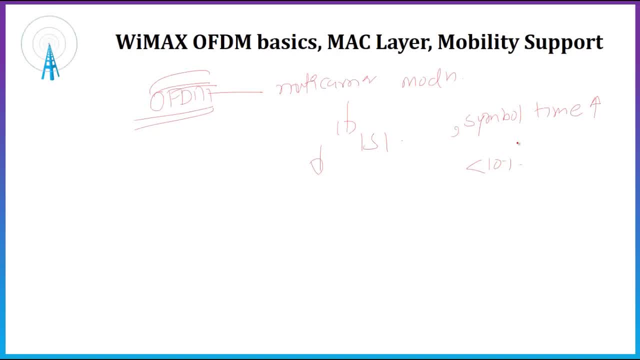 actually used between your OFDM symbols by making a guard interval larger than by making a guard interval larger than by making a guard interval larger than the expected multi multipath delay spread, the expected multipath delay spread, the expected multipath delay spread. so ISN game, you can understand that it can. 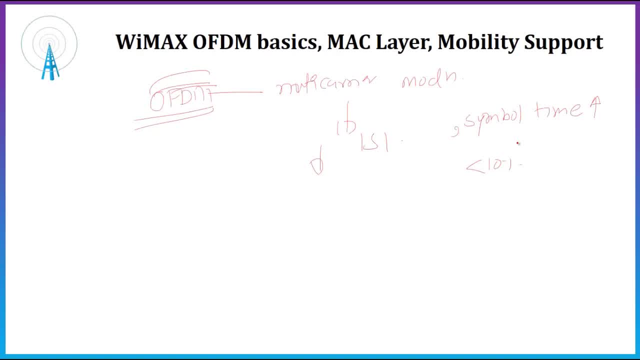 so ISN game, you can understand that it can. so ISN game, you can understand that it can be completely eliminated. so adding a be completely eliminated. so adding a be completely eliminated. so adding a guard interval, however, implies power guard interval, however, implies power. guard interval, however, implies power wastage and again decrease in a bandwidth. 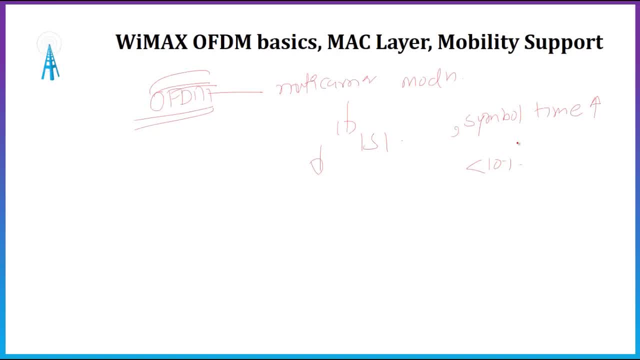 wastage and again decrease in a bandwidth wastage and again decrease in a bandwidth efficiency. so that is all about your OFDM efficiency. so that is all about your OFDM efficiency. so that is all about your OFDM. so what is a Mac layer? so I triple: 8: 0. 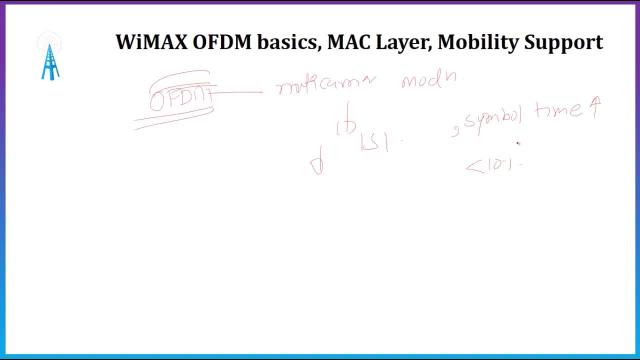 so what is a Mac layer? so I triple 8: 0. so what is a Mac layer? so I triple 8: 0. 2.16 Mac was actually designed for point. 2.16 Mac was actually designed for point. 2.16 Mac was actually designed for point to multipoint broadcast or broadband. 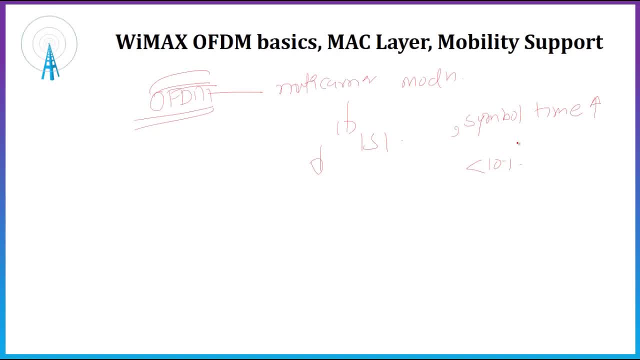 to multipoint broadcast or broadband. to multipoint broadcast or broadband wireless access application. so the wireless access application, so the wireless access application. so the primary task of this Mac layer is to. primary task of this Mac layer is to. primary task of this Mac layer is to provide you what we could say the 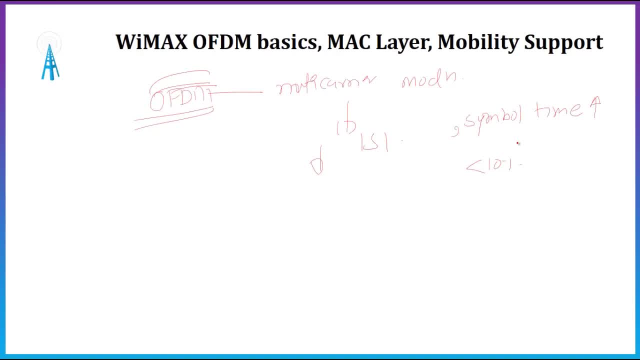 provide you what we could say. the provide you what we could say: the interface between your higher transport interface, between your higher transport interface, between your higher transport layer and physical layer. okay, so the layer and physical layer. okay, so the layer and physical layer. okay, so the what we could say, the Mac incorporates. 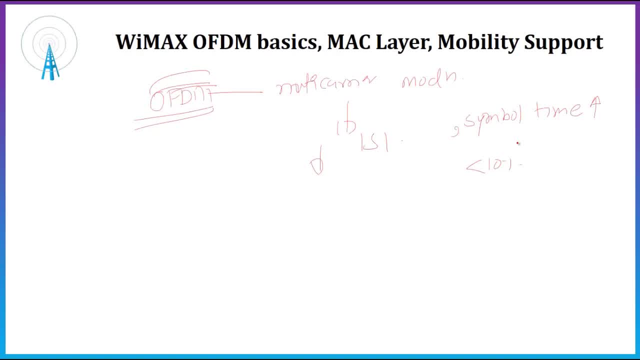 what we could say. the Mac incorporates what we could say. the Mac incorporates several features like primary key, several features like primary key, several features like primary key: management, then Mac layer security, then management, then Mac layer security, then management, then Mac layer security, then broadcast and multicast support- manageable. 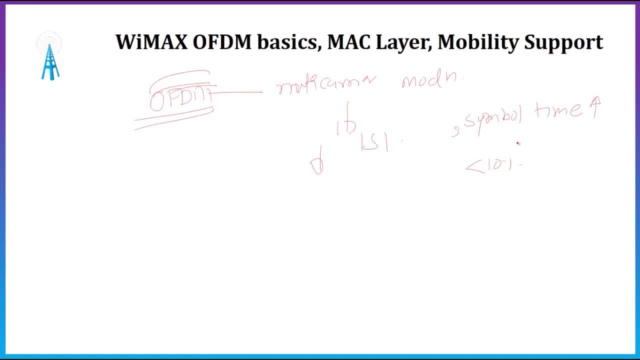 broadcast and multicast support: manageable broadcast and multicast support: manageable primitives, then high-speed handover and primitives, then high-speed handover and what we could say mobility management primitive, then three, three level power management. then there will be simply like normal operation, sleep idle will be there, header separation would be. 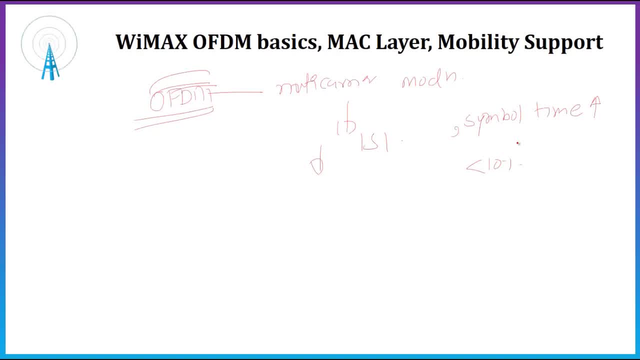 there, then packing and fragmentation for efficient use of your spectrum. then there is again something called as: your five service classes are there, like unsolicited grant services there. real-time polling service is there. non real-time polling service is there. then there is, like best effort, extended real-time variable rate, something like er er t? vr. it is called as, so I'll just repeat it. 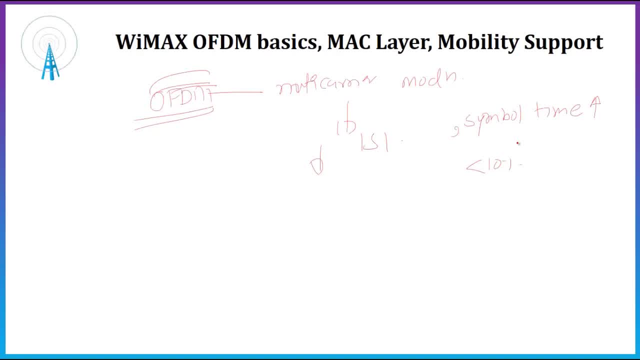 again: er t vr, so e is supposed to be extended real-time. yes, I'm right, so it is actually er t vr, so extended real-time variable rate. okay, so these kind of services are there. so this is actually your function of your mac layer. then mobility service are like what we could say. there are actually four mobility. 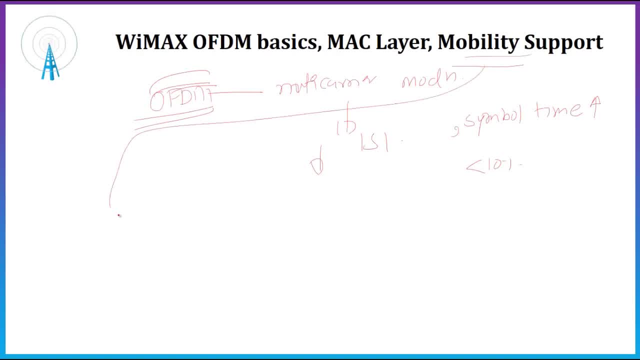 related scenario for this. so there are actually four. so what are all those? so the first one is actually it is called as nomadic, then there is again called as a portable, again there is one more called as a full mobility and then now again there is actually a simple mobility. but while considering to write these, 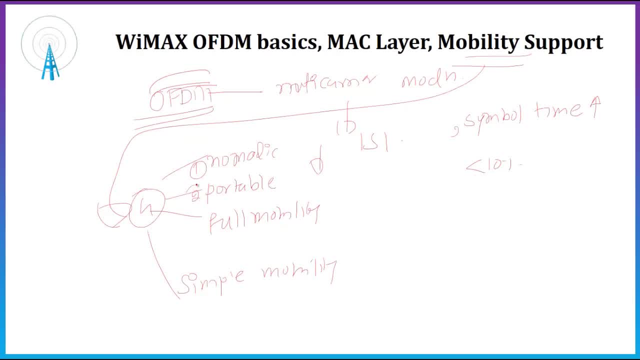 kind of things always consider this to be a first. second is this: this should be fourth and this should be third, because that creates actually a proper flow. so what is nomadic? so nomadic is actually: the user is allowed to take a fixed subscriber station and reconnect from a different. 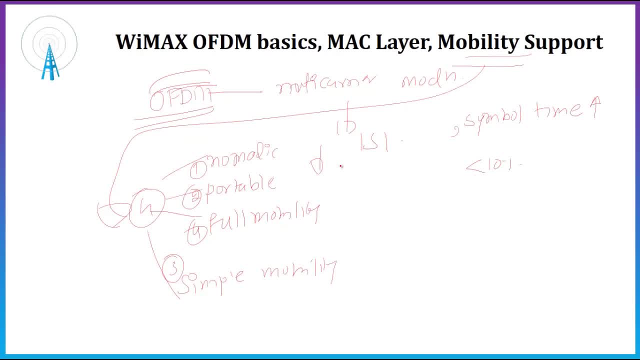 point of attachment. so that is called as your nomadic. So what could be a portable then? So nomadic access is provided to a portable devices such as PC card, with the expected best effort handover. Okay, Then the full mobility would be like up to 120 kilometer per hour mobility, seamless handoff. So these kind of features are there Again, in simple mobility, a subscriber may move at a speed of 60 kilometer per hour, with a brief interruptions, less than like one second during your handoff. 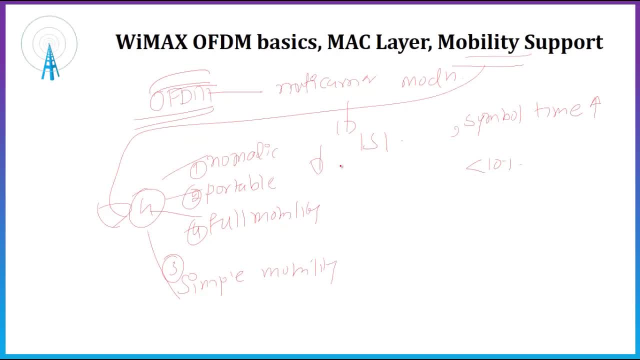 So these are actually mobility supports or usage scenario for your, what you could say, mobility related user scenario, usage scenario, the better word. So it is likely that WiMAX network will initially be deployed for a fixed or nomadic application and then evolve to support like portability for a full mobility over time. Okay, So there has to have again consideration of security functions. 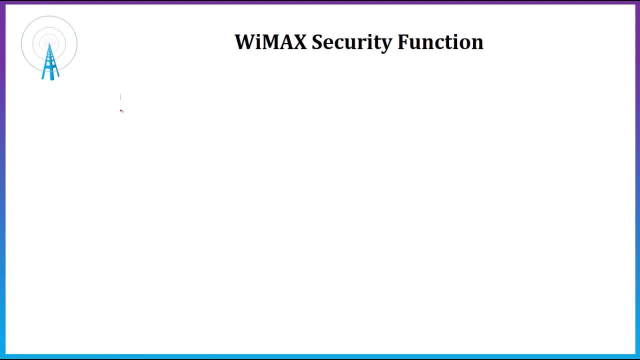 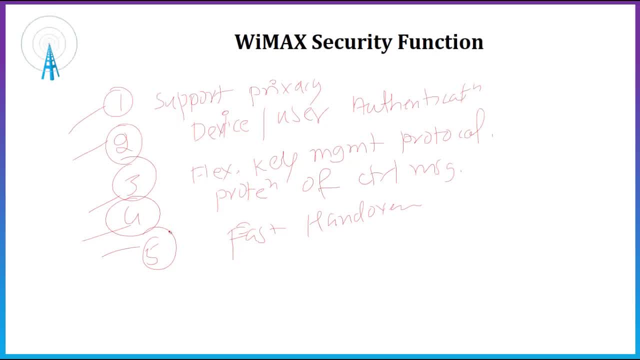 like user data in this case, is encrypted. your cipher scheme, or we could say your cryptographic schemes, and it pro it provided actually a robust robustness to create your privacy. so both like aes and your 3des, like triple data encryption standard, were actually supported. so here, 128 bit, 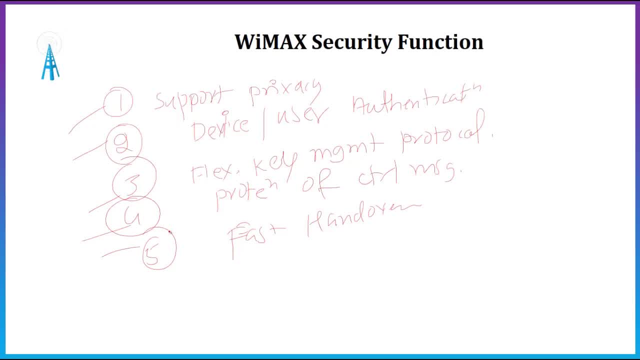 and 256 bit key is used to derive that cipher generated during the authentication phase. so again, this device and user authentication is merged, then flexible key management protocol should be there. there is actually one protocol which is called as actually a PKM v2, so it is. 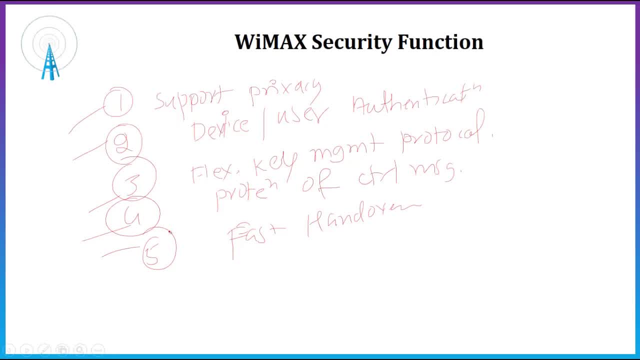 actually a privacy and key management protocol, version 2, which is used for a transmitting king material. so again there has to be a controlling messages like md5 based HMAC- all those hashing schemes are there. so fast handover. obviously it should not be simply like there is a delay, then if there is a delay, then there will be a drop. so obviously the fast. 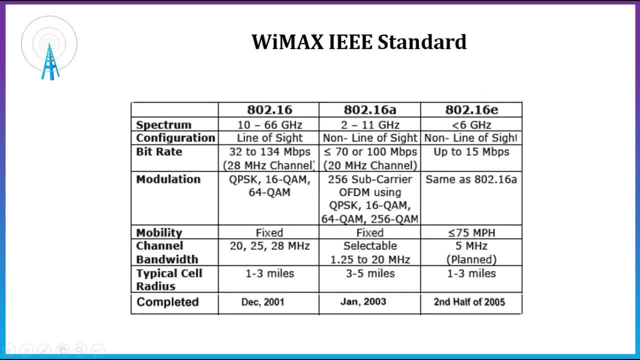 handover and all those things should be there. then there are actually various y max IEEE standards, so they are listed like this: 802 point: one six, one six eight and one six eight. so we primarily focused on this y max IEEE standard of a so which is actually- we have already seen that it is based on two to 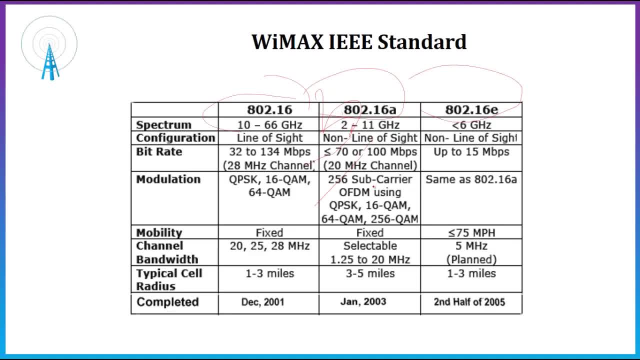 eleven, non line of sight- seventy or hundred mbps, then 256 subcarrier OMDM, then there is a fixed mobility, then when it has arrived, then typical channel radius. so these kind of parameters are there while designing these kind of IEEE standards, so the IEEE 802, point one, six standard for 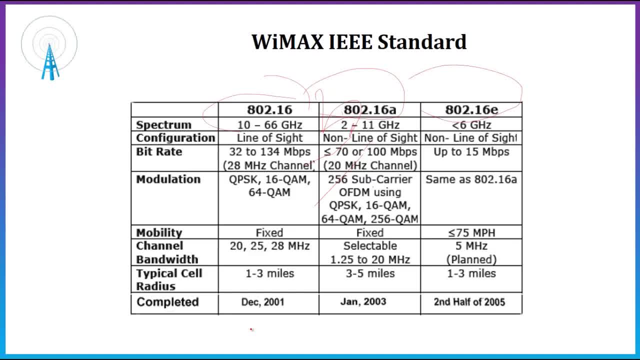 what we could say wide broadband access, so the possibility for the interoperability between your equipment from different vendors, which is in contrast to previous year BW industry where proprietary products with the high prices are actually dominant in a market. so these are actually different standards related to your y max. 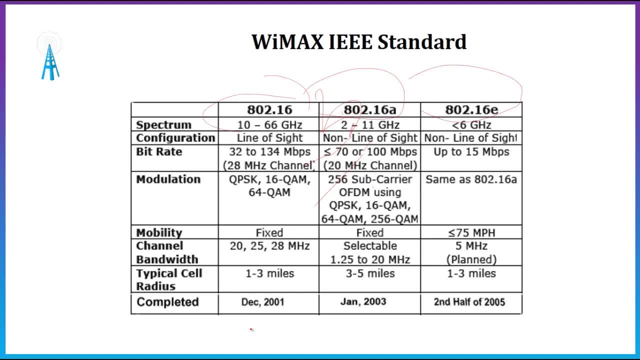 for those who are not familiar with Zelda 3, for you, because this one has its own. so just one more point. I think I have just follow and I'll just quickly cover that thing. so they's actually one more thing I needed to drill. I need to add on to: Why does football油なんто? 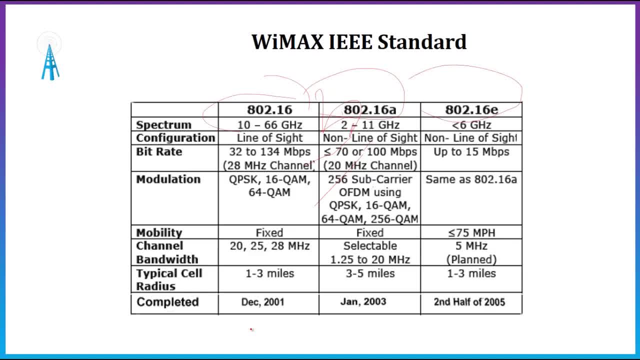 are typically delivered to smartphones and other handheld devices sold by your cellular service providers and their retail partners, but the mobile devices can be used. mobile devices can use them as well. some netbooks are available with like w1 cards installed and you could also purchase wireless fan cards to install it yourself, unlike wi-fi cards, which can